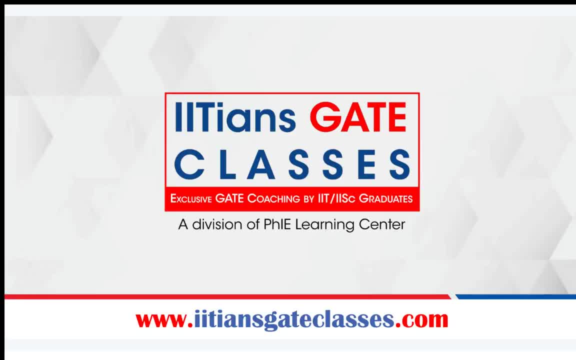 Thank you. So all of you have tried this particular question- homo problem- that I have given to you. Anyone has tried that. All right, Thank you very much. Thank you, Yeah, very good morning to all of you. Let's start the session. 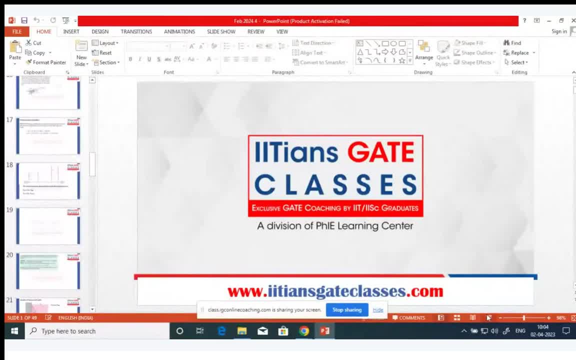 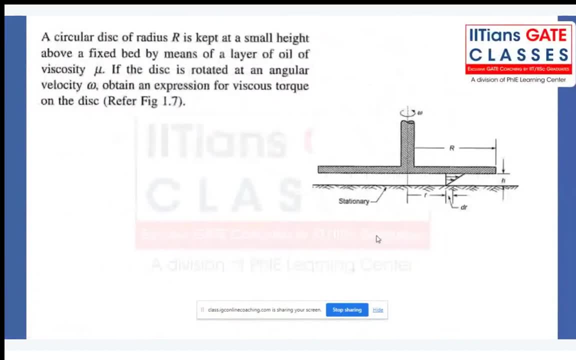 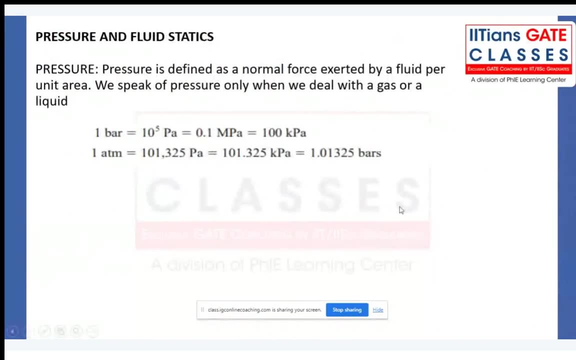 Yes, so we are discussing about the fluid statics and we have just started our discussion on to that and we have seen that somewhat, the differences between the pressure and distress, that at a particular point the pressure value will be same in all the directions, right, 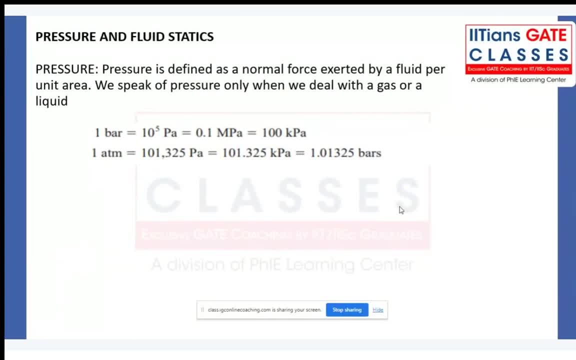 As it is not having any specific directions. So we say that it is a scalar quantity, Rather to say about the pressure. we also talked about something about the stress, that stress is a second order tensor right. That means we, for denoting the stress value, we not only require the particularly what 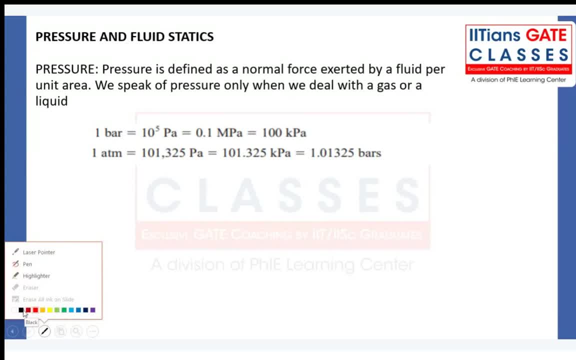 we say T, So whenever we are representing the stress. so we require two indices, right? What is it? X and X? What is the meaning of that thing? One will be required. Not only you will be required that particular plane, but you need to specify the directions. 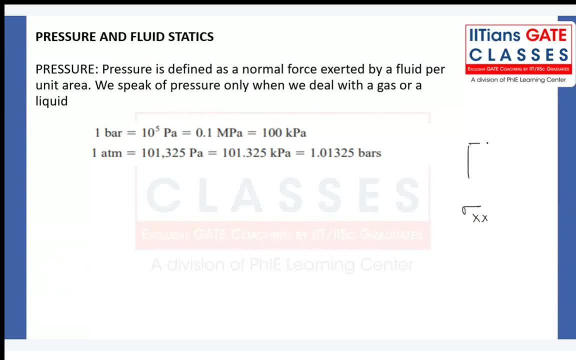 of that stress which is acting right. That means, if I draw the cubical element, so in that cubical element, if I just make it Something like this, this will be, for example, X axis, Y and Z. 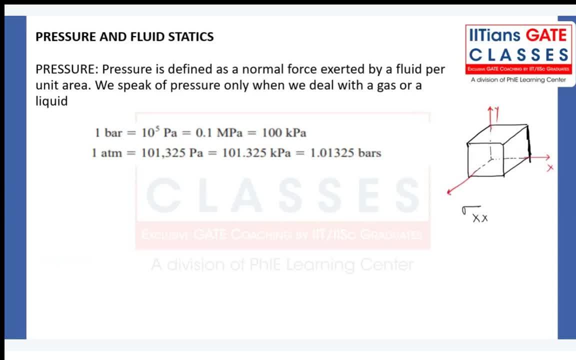 So what about this Sigma? On which phase it is acting? This is acting on a particular X phase, right? What is the meaning of phase? The phase which is perpendicular to what Particular plane? right Now, I am saying that this particular plane is an explain, right. 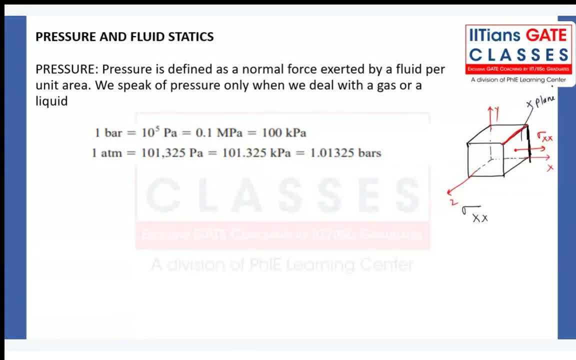 Because X axis is passing through What is? it is passing through that, right, that is the x phase and x direction, right. so this one will denote it: the phase or a plane on which it is acting, and directions, right, something like this. so if i represent it like this, then what we can write on a y phase: 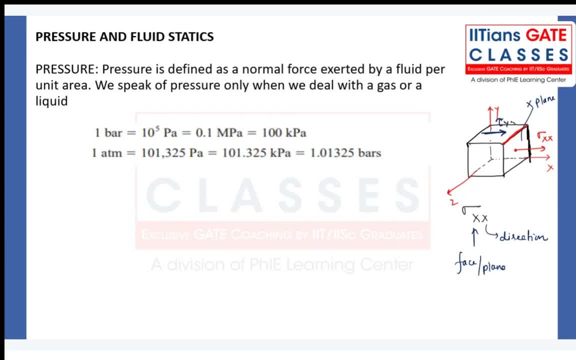 in x direction, so this will be yx. right, so we used to represent it by two indices: right, that is a second order tensor. right, second order tensor, that is a. but you, whenever you observe the fluid element, whenever you observe any fluid element, same cubicle element, if i just draw, 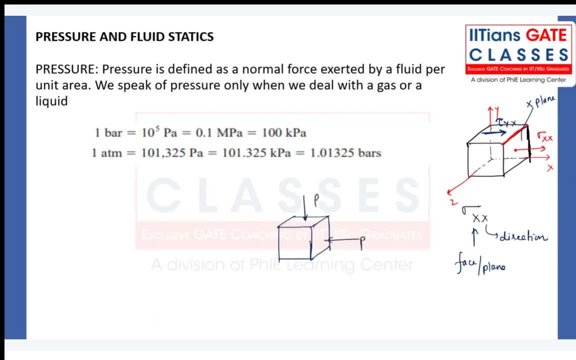 it. so what? i will just say: whatever the pressure will be acting, the pressure will be denoted by like this: we don't say at all that it is px, it is py, it is pz, because px equal to py, equal to pz, that is equal to minus p. so no need to specify the direction. 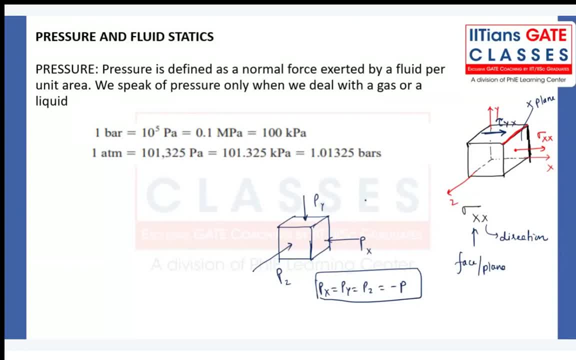 correct for the case of pressure right, that is the. we have the differences between the pressure and the stress right and this particularly hydrostatic. this is what we are calling. this is we are calling hydrostatic state of stress right. this is a general state of stress condition, general. we will talk in some in the strength of 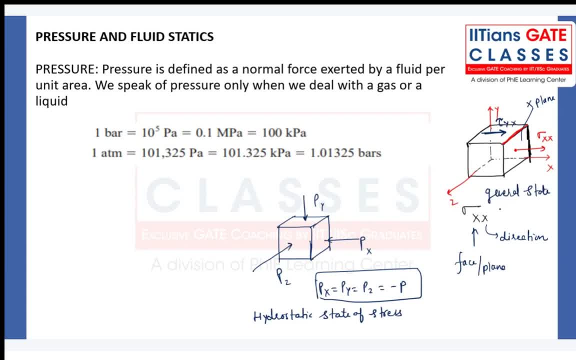 material. as of now we are dealing with the some basic understanding, general state of stress. of course you will be having some another. i only so on. i just shown you this two component of the stresses, but actually there is a matrix. you know there will be totally nine component in that. 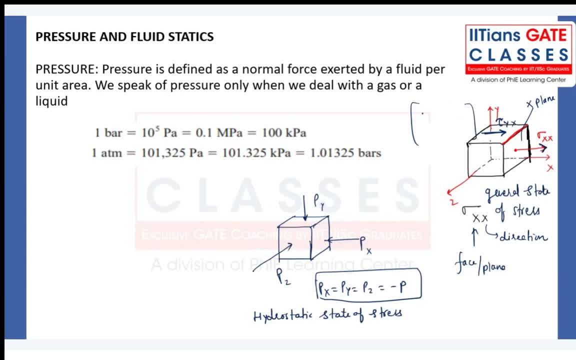 three components will be what same and six components are independent and three components are equal. actually, tau x, y is equal to tau y x, tau x, z is equal to tau z, x and tau what we say, z, y equal to tau y, z. right, Total components of the stress are 9 at a particular point. 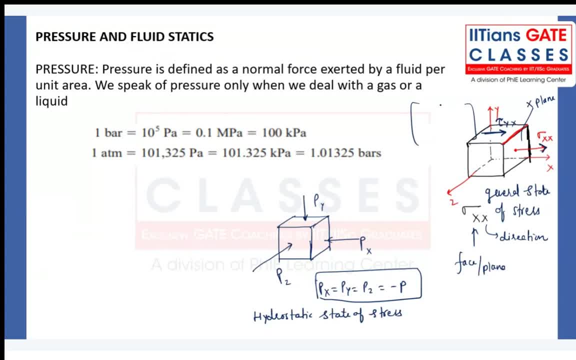 So these are the some differences, what we have observed in case of pressure and the stress. So that is also one of the famous question that can be asked about the differences between the pressure and stress. One more difference is there: pressure can be measured with the help of what? 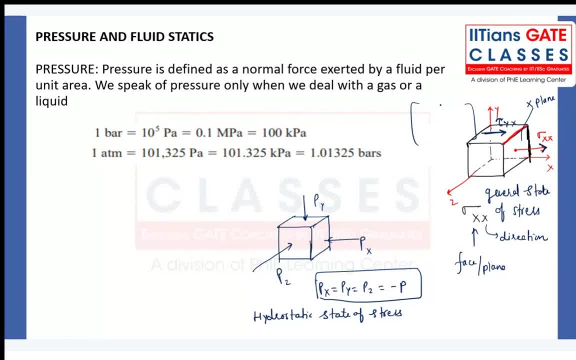 Strain gauges, Sorry, whatever the pressure gauges are there, with the help of pressure gauges we can able to measure the pressure right, Yes or no? guys, Getting my point, what I am saying? No distortion will occur. 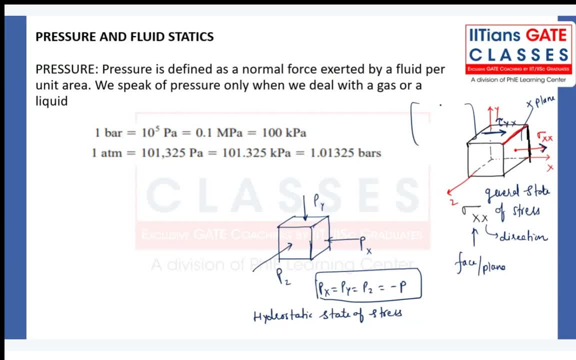 There will be. only volumetric changes will happen, right. Only volumetric energy will be stored. right, Volumetric strain energy will be stored. there will not be any distortion energy in this case. Tell me, guys, how to measure the pressure. 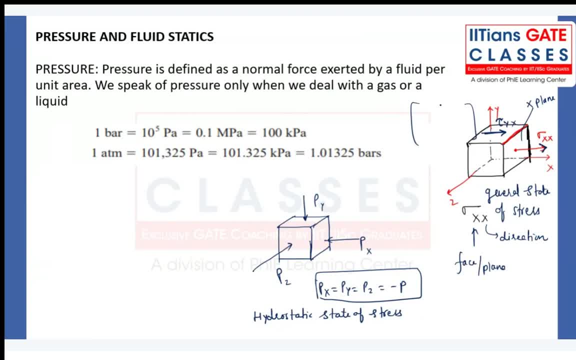 How to measure the pressure. Pressure can be measured by pressure gauges, right? Have you seen that We just connect it like this and we can able to measure the, whatever the pressure is there of a particular control volume or of a particular room, right? 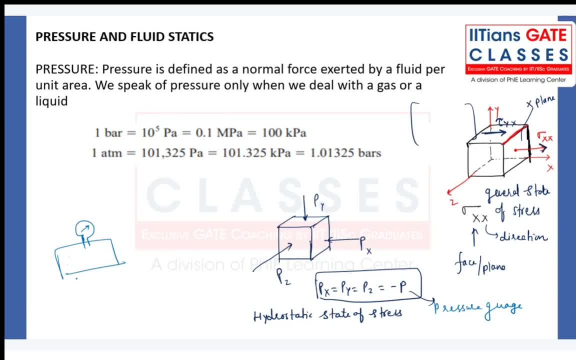 But the stress cannot be measured directly, right Stress. for measuring the stress, of course we have the universal testing machine. but universal testing machine will not give directly the values of that. It will give the release of different, different deformations and through making the table, 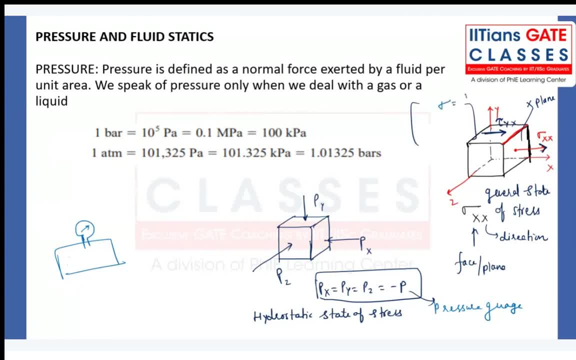 we can able to get the values off Sigma. What is that? Force divided by area, right, So force that will be applied by the universal testing machine directly. there is no such an instrument called stress gauge or something like that by means of which we can measure. 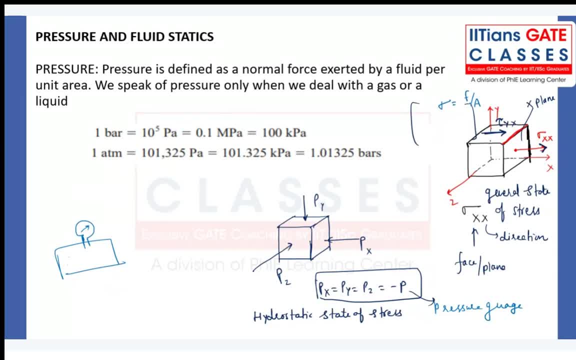 the stress. No, we do not have such an instrument directly. We have to perform the experiment right Now. the magnitude of the pressure value at a particular point will be same in all the directions. That is valid when the fluid is under rust condition, but that is also valid when the 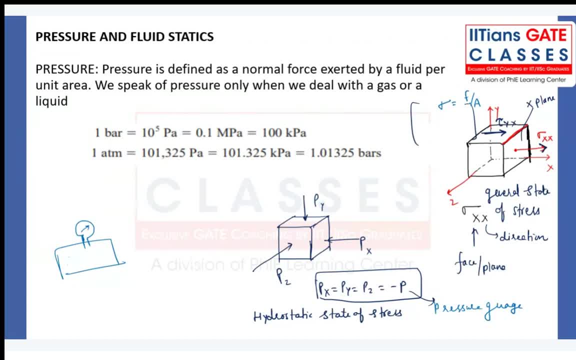 fluid is under what? In a rigid body motion, right Now, what is a rigid body motion? We will see that That is a different phenomena. And one more thing. I would like to tell you that here. Okay, So whenever the fluid is subjected to hydrostatic state of stress, whenever the fluid is subjected 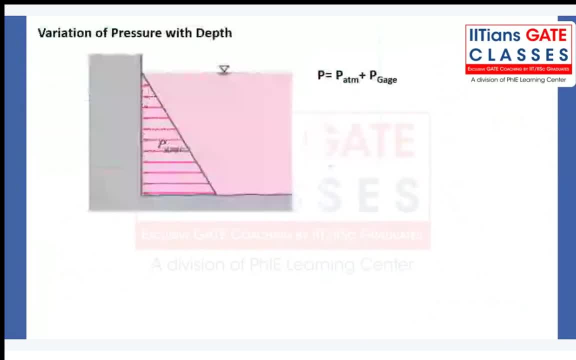 to hydrostatic state of stress conditions, you will be having just wait. Yes, Okay, So whenever the fluid is subjected to hydrostatic state of stress, for example, you are talking about the fluid case where it is being subjected to hydrostatic state of a stress condition. 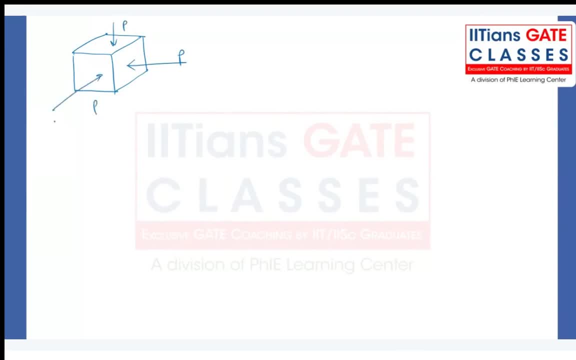 like this: P, P and P. So if I make it 2D figure of that, something like this: this will be P, This will be P. Now, if you just make the, this will be P. Now, if you just make the. 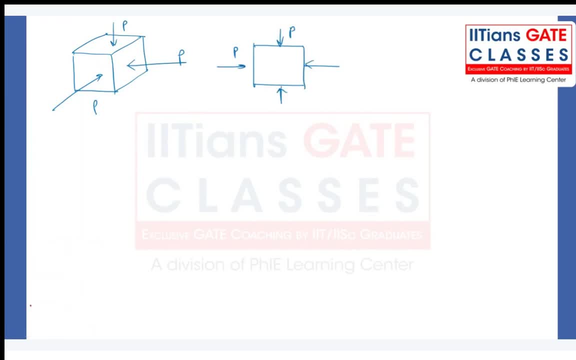 if you just make the Mohr circle of that and you know I'm talking about the hydrostatic state of stress, hydrostatic state of stress. Now, in case of hydrostatic state of stress conditions, if you just calculate the tau, is theta right? 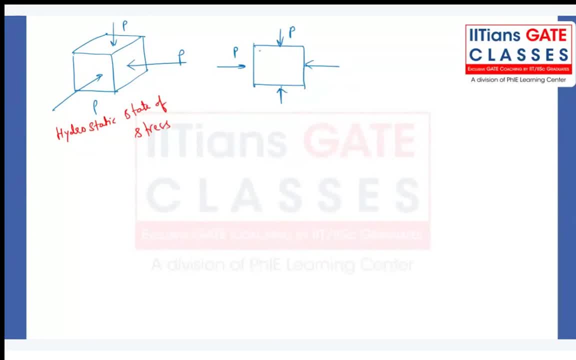 Very well. So when you just calculate the tau is theta at an angle, theta from a plane, what is the value? of tau is theta If you just want to calculate, right. So this formula I have discussed, I think, in the particularly, you know, demo class. 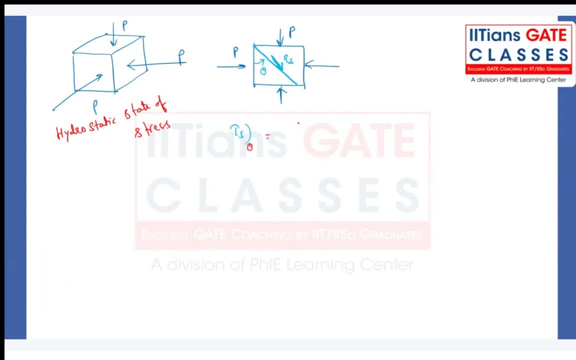 what is the shear stress formula at an angle theta? we have seen this one. What is that? Sigma X minus sigma Y by two, minus of that, sine two theta plus, Okay Okay. Sigma X minus sigma Y by two theta plus tau X Y cos two theta as this particular element. 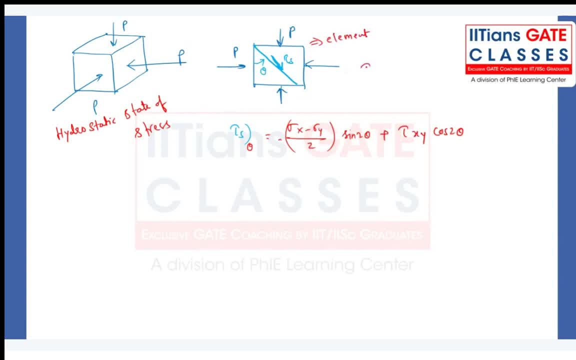 this element is stress element- is not subjected to any tau X Y. as you can see, there is no such a value called tau X Y. tau X Y is zero, right. This is zero. Sigma X is what Minus P Sigma Y is what. 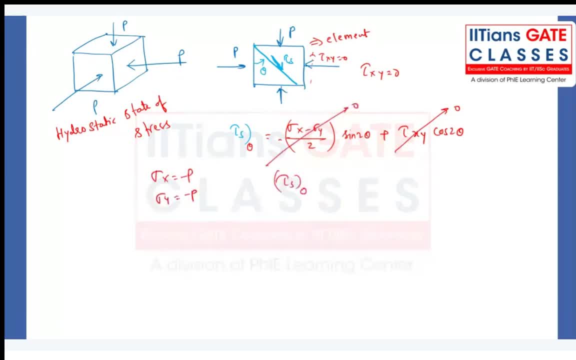 Minus P. Once again, this will be zero. So tau is theta will become zero. That means when tau is theta will be zero, my different right right. what you are calling about that? tell me guys. there will not be any. say the stress. 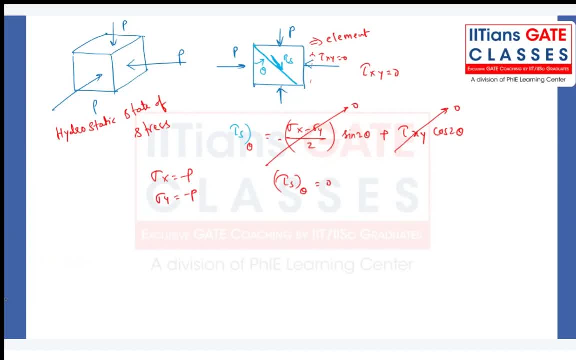 will be acting in a fluid element which is being subjected to hydrostatic state of stress conditions. getting my point, the fluid element will not be subjected to any kind of say stresses whenever the fluid is under what, subjected to hydrostatic state of stress conditions. make a note of it. 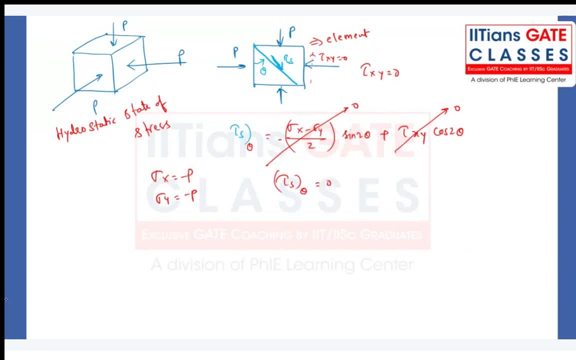 you. so that's why you know the reason. you will observe that there will not be any say deformations whenever the fluid is subjected to hydrostatic state of stress conditions. whenever the fluid element is subjected to hydrostatic state of stress conditions, they will never gonna undergo right. 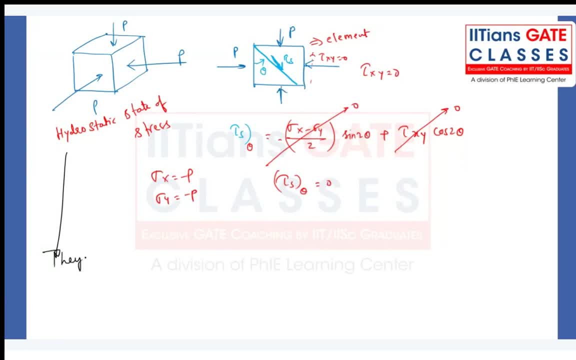 they will never undergo right right pain. distortion. what is the meaning of distortion? see, I am talking about the fluid element. yes, they can. basically what increase or decrease as a pressure is acting? definitely the volume will decrease. definitely total volume will decrease. there is no argument in that, you know. 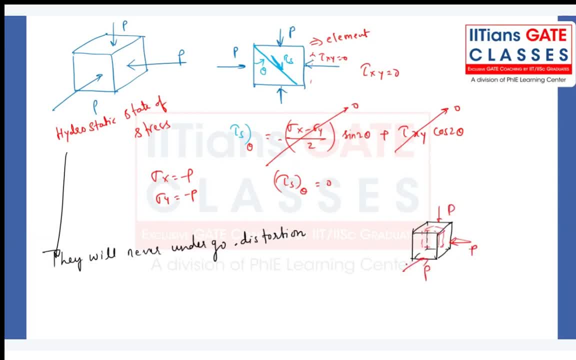 because of the pressure value. whatever I am saying that they may decrease their volume, linear deformation in x, y, z directions, but there cannot be any say deformations, right? that's why you observe sea rock or submarines, right? whatever the submarines are there, the submarines are basically subjected to what they are never gonna fail. uh, you know, fail by distortion they will. 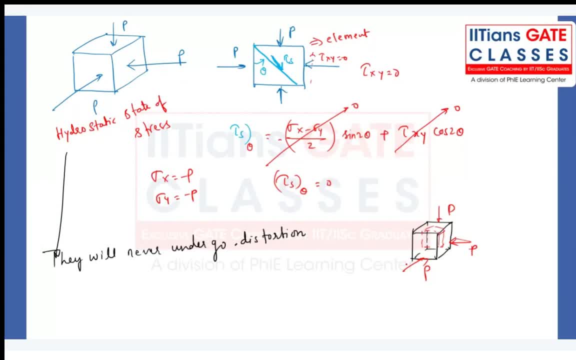 always basically fail by normal stresses. right, make a note of it correct. there will not be any safe changes, right? i'm talking about, say, deformation means something like this: this is a fluid element. now the safe will change like this. or maybe we can have the safe changes like: 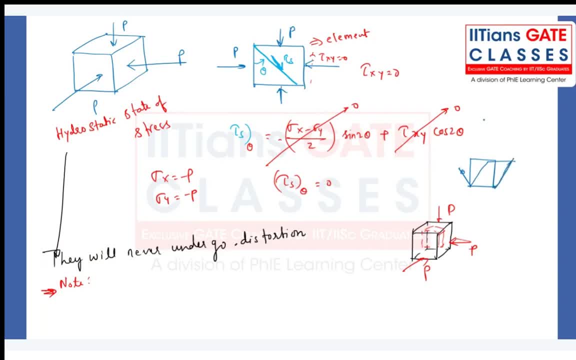 this, you know, or if we have the deformation like this, something like this, these are the safe changes. this is only possible when the fluid element is subjected to some kind of say stresses: right, this tau value, when there is a, no tau, c, tau s, theta is zero. means what? not only on one. 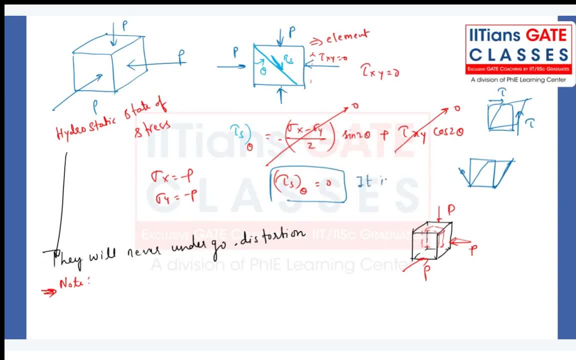 particular plane, on any plane. it is independent of orientations of planes. that means, whether you rotate theta equal to 0, theta equal to 90, theta equal to 45, theta equal to 30, theta equal to what 46 degrees theta is equal to what 76 degrees theta is equal? 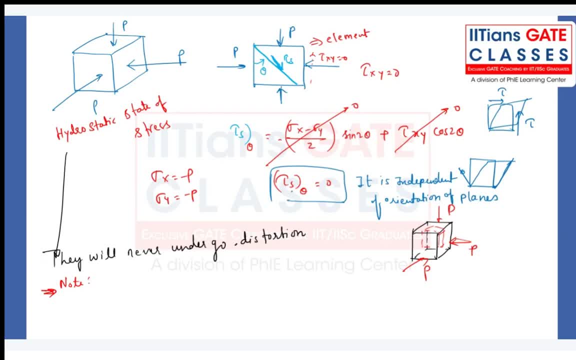 to what? 200 degree? whatever the degree you rotate it, everywhere, tau s theta will be zero, right, so make a note of it. see, rock submarines fails by normal stresses. right, they will never undergo the distortion or CA deformations, because, see, tau s theta. tau s theta is what, according to Hooke's law, for this: 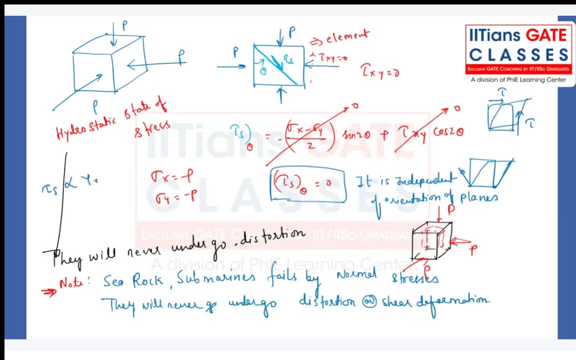 air. tau s is what directly proportional to gamma XY, for example, gamma right. this is what gamma is what. my different? this is nothing but say a strain right. and in case of fluid, that will become what say this strain rate. if tau s is zero, then this will also be zero. that that is as simple as that. is that clear, all of you. 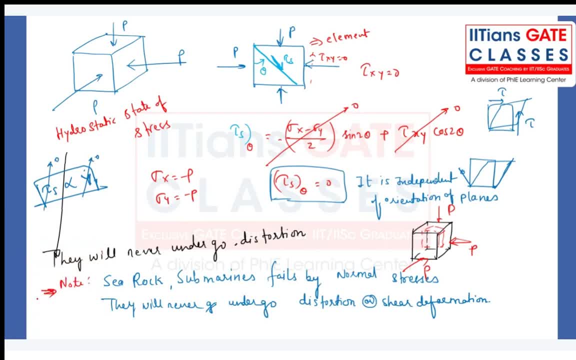 all of you are understanding or not, when we discuss the in the solid mechanics. the picture will be more clear when we talk about the different different types of state of stress condition, in that one of the special case- hydrostatic state of stress conditions which, see, you might be thinking so- this is a solid body of fluid body. see, 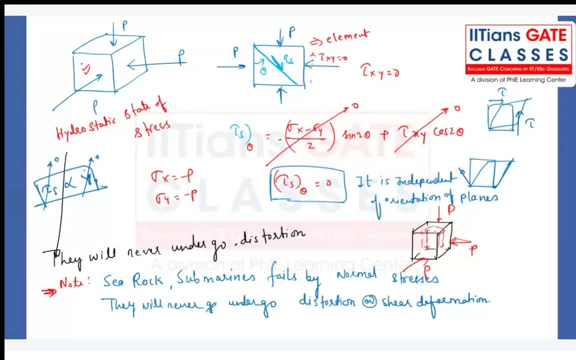 whenever we talk about this whole body, we don't say pressure value, we say stress. we say 3d compressive stress of equal magnitude. but the moment we are talking about the fluid, liquid or gases, we don't say stress, we say that, okay, pressure value is acting right. so that's why the name, basically the basics only. I 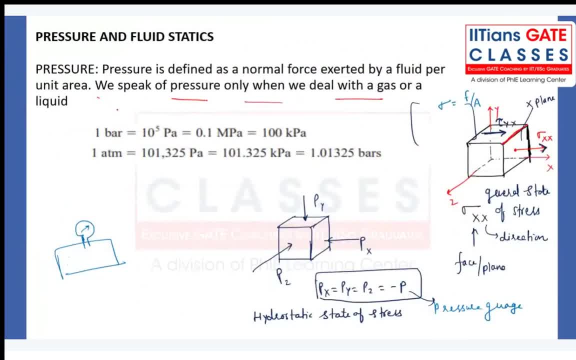 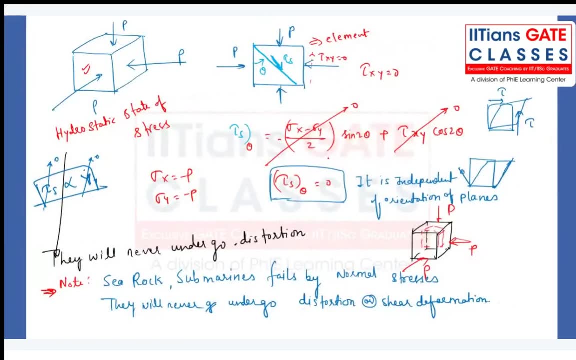 have given that we speak of pressure only when we deal with the gas or liquid right, and that is not given by me, that is given by singel right. so definitely there has to be validity of that statement. so, whatever the things we have discussed in the past, I would say 20 minute or in the last class, in the last 10 minutes we are 30 minutes. so, whatever the things we have discussed in the past, I would say 20 minutes. or in the last class, in the last 10 minutes, we are 30 minutes. so, whatever the things we have discussed in the past, I would say 20 minutes. or in the last class, in the last 10 minutes, we are 30 minutes. so, whatever the things we have discussed in the past, I would say 20 minutes. or in the last class, in the last 10 minutes, we are 30 minutes. so, whatever the things we have discussed in the past, I would say 20 minutes. or in the last class, in the last 10 minutes, we are 30 minutes. so, whatever the things we have discussed in the past, I would say 20 minutes or in the last 10 minutes we are 30 minutes. so, whatever the things we have discussed in the past, I would say 20 minutes or in the last 10 minutes we are 30 minutes. 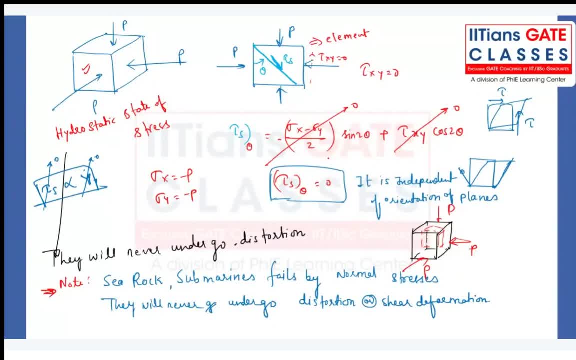 will play a very important role whenever you go for any interview in Emtek. also, suppose you are opting for any, you know interdisciplinary branches in ISE. definitely, you have to face the interviews and these are the questions will be there. Now, once it is done, let me know. can I move to the next segment? 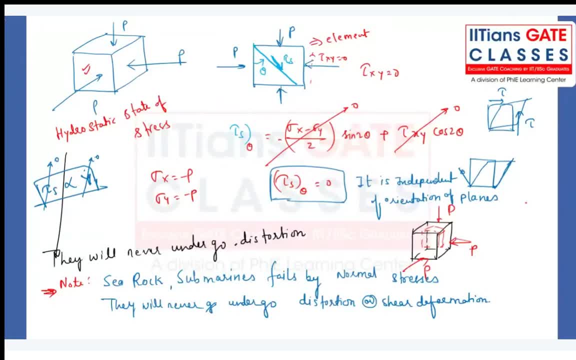 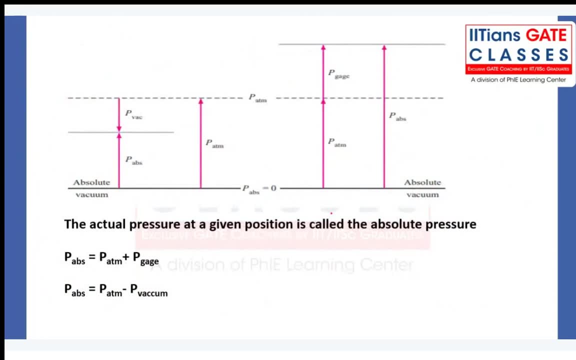 See, guys, note down the next segment, the types of pressure we are going to see. So note down, as you can see, this particular diagram, so make a note of it, very, very important note: Actual pressure at a given position is called absolute pressure. 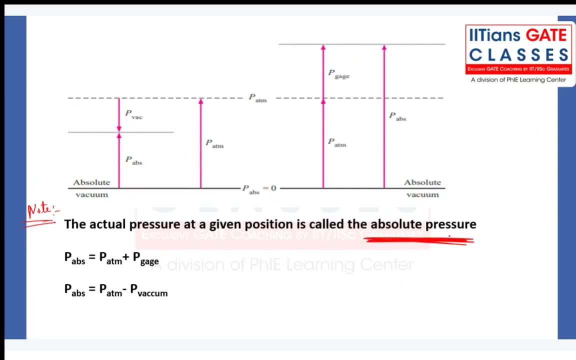 So any law? you know that at a particular point the pressure is same in all the directions. We say something law, Tell me this pascal law, not tell me whether pascal law is only applicable for the fluid at the rest condition or when the fluid is under certain type of situation, where it is. 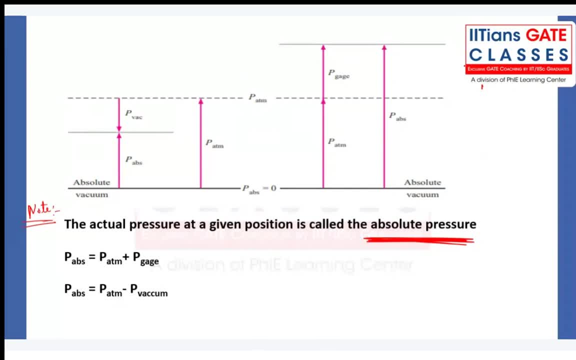 under motion also. it is applicable because we always heard the pascal law whenever the fluid is at the rest. That is the start, That is the starting of this statement. The pressure is same in all the directions, but remember that the pascal law is applicable. 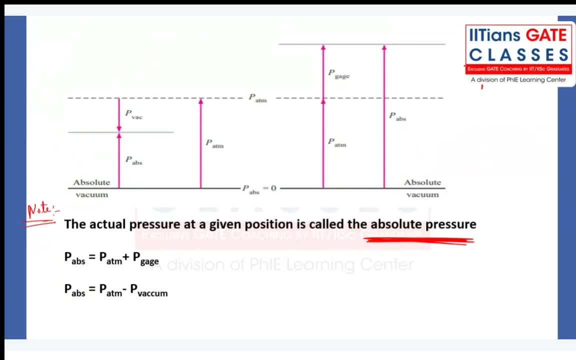 even though the fluid is undergoing motion, that is, a rigid body motion, Even though it has the acceleration. still we talk about the validity of the pascal law, How and why. we will discuss about that in detail, about discussing this particular slide. 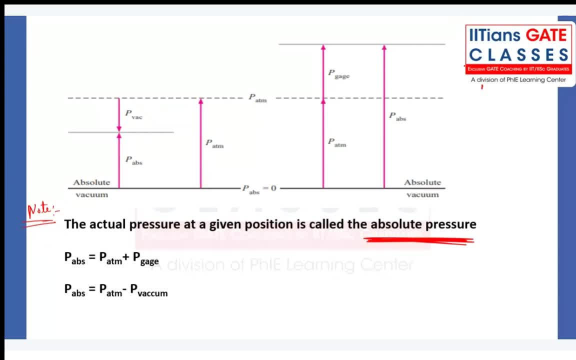 So, guys, here are the few points I would like to give. Actual pressure at a given location will always tells you the absolute pressure value. Second thing: you just make a note of it, note number one- and you can make here note number two, as absolute pressure can never be negative. 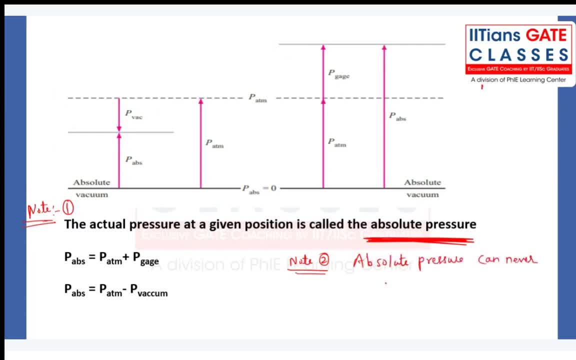 Absolute pressure can never be negative, my dear friend. So what is the first thing you are observing? this is a reference, one right, This is my zero line. Definitely you will be having some atmospheric pressure. What is that value? 101.325 kilopascal. 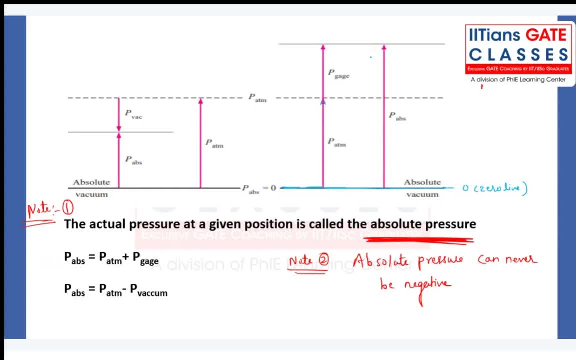 What is the atmospheric pressure? What is the atmospheric pressure? Or one bar, or let us say one atm, right, one atm. So here what I am saying: that you will be having certain values If, at a particular point, right, whenever you have the absolute pressure more than atm. 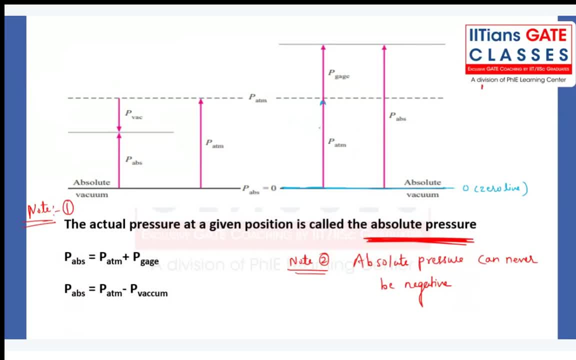 pressure, then whatever the excess pressure is there apart from this atm pressure that we say gauge pressure, right? So what is the definition of the positive gauge pressure? Positive gauge pressure, What is the definition, my dear friend? The definition is whenever absolute pressure, when P absolute is more than P atm, then the 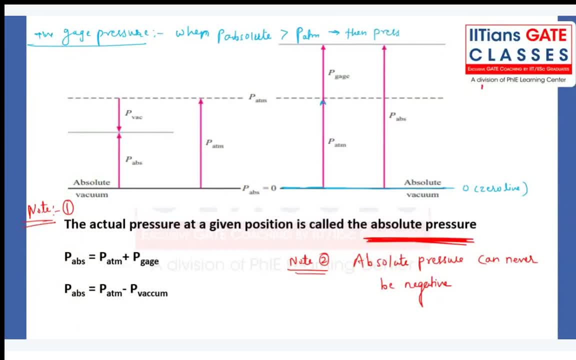 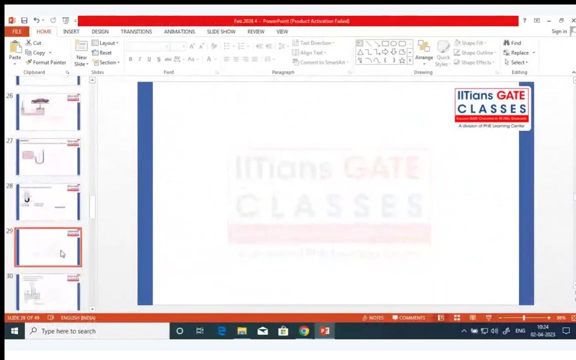 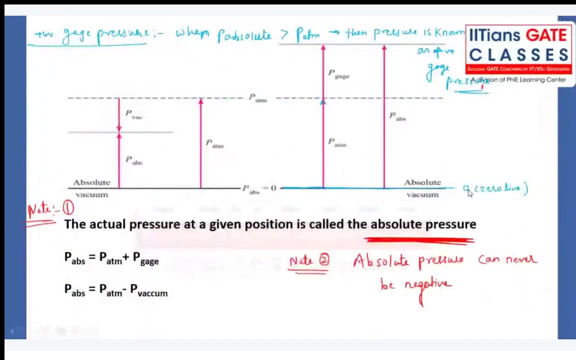 pressure is known as Positive gauge pressure, Then the pressure is known as positive gauge pressure, Or we can also write in the next slide, But sometimes what is happening? the pressure might be total, pressure might be lower than ATM pressure. right, 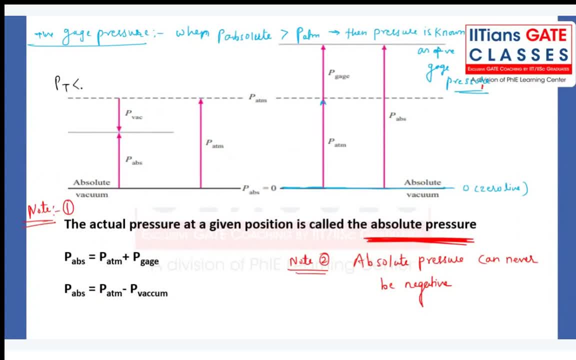 When the total pressure is less than ATM pressure. when the total pressure is less than P-ATM, total pressure means absolute pressure. In that case, my dear friend, you will be having negative gauge pressure. That negative gauge pressure will be called as vacuum pressure. 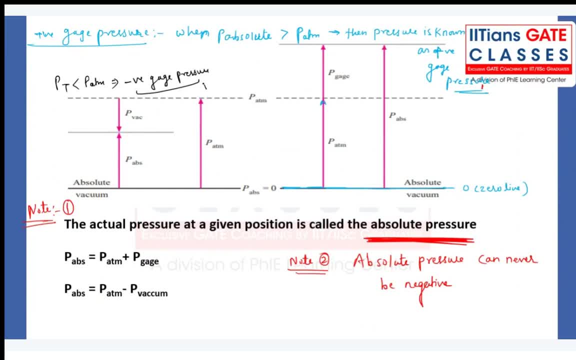 That negative gauge pressure only. we are calling vacuum pressure. Make a note of it Very, very important. So P-absolute is given as P-ATM plus P-gauge. P-absolute is also given as P-ATM minus P-vacuum. 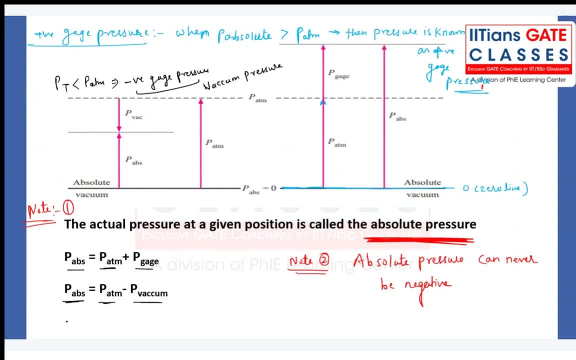 When we said P-absolute might have P- 그래서 proof is different from: But P-absolute is a bungalow. How can I clear this? You know P- irreversibly low, I assure. done all of you. all of you have noted down. 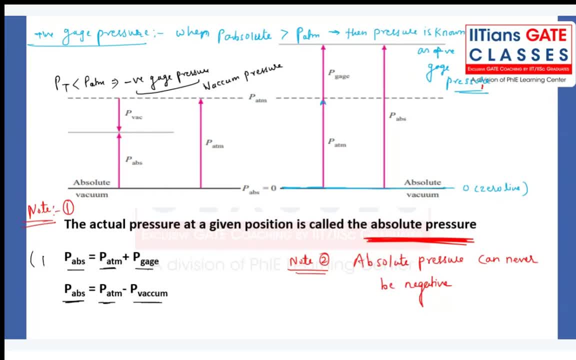 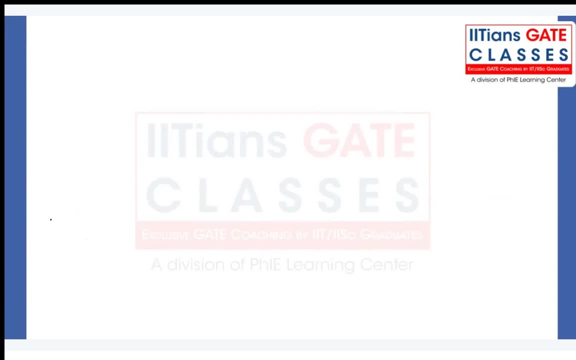 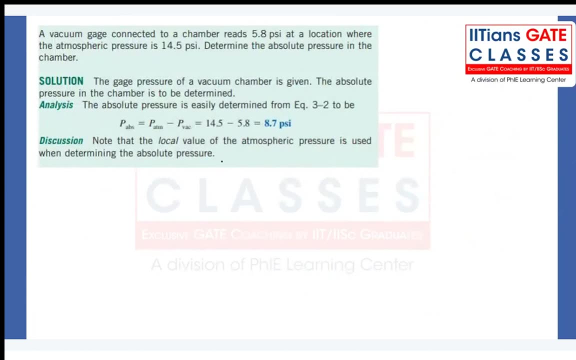 so we also sometimes, sometimes we say total pressure. this is to be as total pressure. now, for example- you will see the example here. one example: a vacuum gauge. a vacuum gauge is connected to the chamber right, a vacuum gauge which is connected to a chamber. let's suppose there is a chamber and i am connecting one gauge which shows me the reading of how. 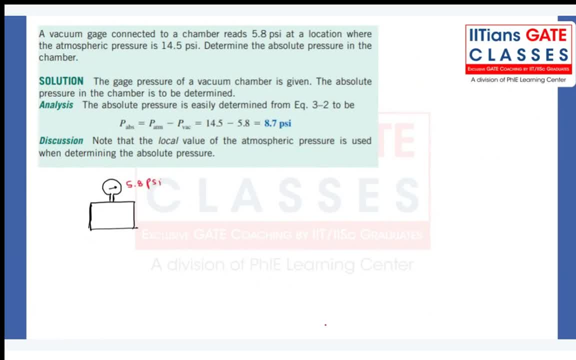 5.8 pascal square inch. that is something you know other than you know. in america they used to follow this unit of pressure. here we deal with the kilopascal or megapascal, something like that. a vacuum gauge connected to the chamber reads the pressure value 5.8. 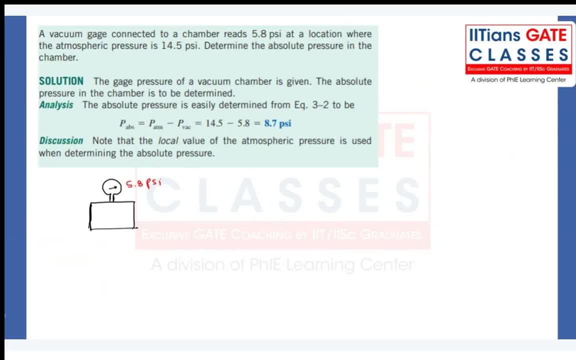 pascal square inch at a particular locations, right where the atmospheric pressure, right where the atmospheric pressure, whatever the atmospheric pressure is there, p atm that is given as 14.5 psi. they are asking what is the absolute pressure in the particular chamber? tell me, guys. so, whatever the vacuum gauge is there, remember vacuum gauge will give me. 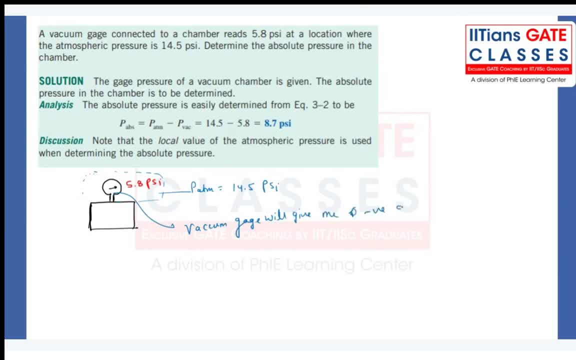 the negative gauge pressure. whatever the vacuum gauge is there directly will give me the negative gauge pressure. what is the gauged pressure here minus five point eight psi? so what is the total pressure or what is the absolute pressure, p atm minus P gauge pressure. so what we can write p atm is what? fourteen point five minus five point. 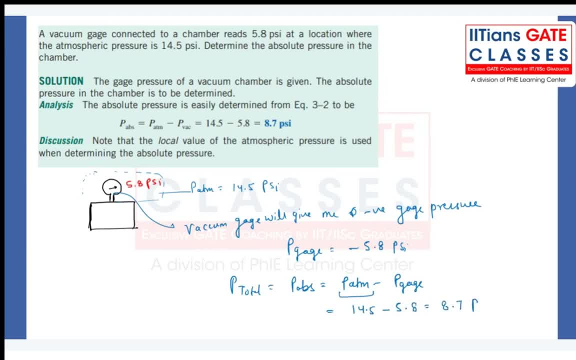 point eight. when you calculate you will be getting what? eight point seven pascal square inch. and that is so obvious that absolute pressure at a particular location, at this location, the absolute pressure, absolute pressure, my different- is less than p atm. that's why you have the what. 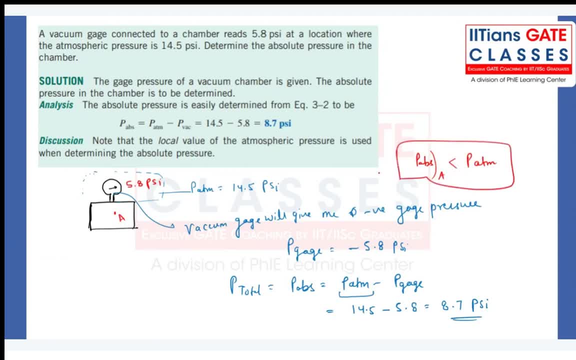 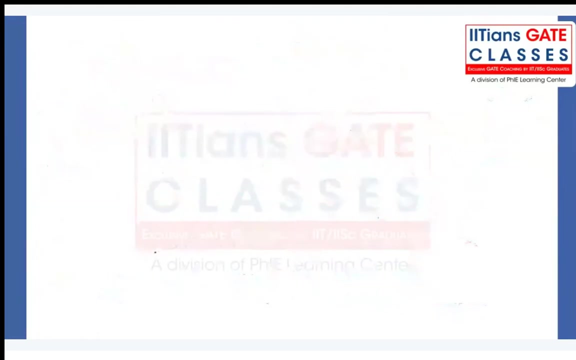 negative gauge pressure. that's why you have the what vacuum. so remember that absolute pressure cannot be negative, even though gauge pressure can be negative, but it absolute pressure cannot be negative. then all of you have noted down. can i move to the next one? so here we will try to see the pascal law. no doubt. 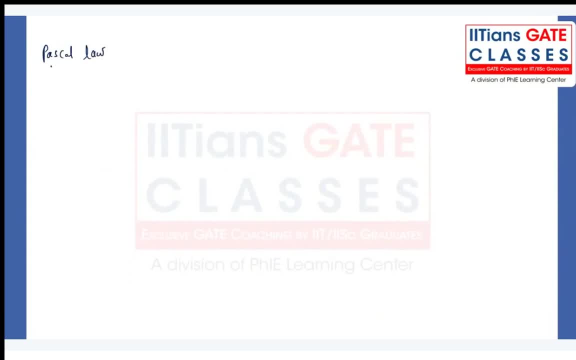 pascal law. note on this statement. according to pascal law, according to pascal law, pressure at a point, pressure at a point in a static fluid, pressure at a particular point in a static fluid is equal in all directions, is equal in all the directions. that means at a particular point the pressure might be acting. here p3 pressure might be. acting over here: p1 and p2 and p3 and p4 and p4 and p5 and p6 and p7 and p8 and p9 and p10 and p11 and p12 and p13 and p14 and p14 and p15 and p17 and p18 and p19 and p19 and p20 and. 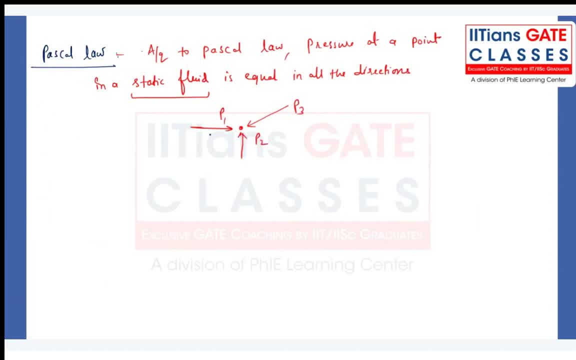 p22 and p23 and p19 and p20 and p21 and p23 and p19 and p20 and p22. so according to pascal law, if the fluid is static, for a static fluid, p1 equal to p2 equal to p3, that will be equal. 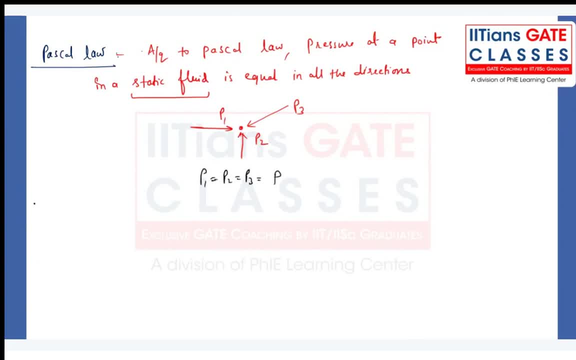 to directly p. we can write right. so my different. in a static fluid, what are all the forces will be acting in a static fluid? in a static fluid, what are all the forces will be acting? So there will be some pressure forces, Px. let us suppose this is Dy, this is Vx and 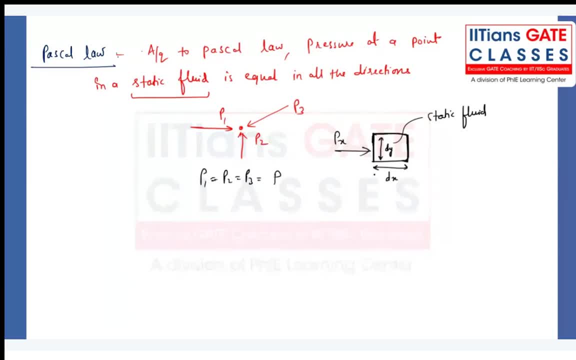 width. I am considering one unit that is perpendicular to the laptop screen. the width I am considering as one unit width. I am taking it as one unit, for example. so what is the volume of that element? the volume of that element will be dx, dy into 1.. 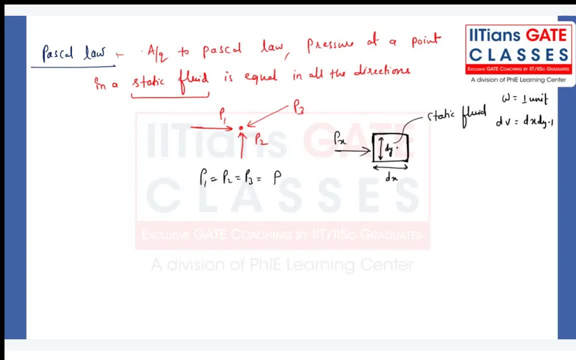 So definitely there will be some body force will be acting. the body force will be acting like this: rho. what is the body force? body force, we know that body force. we know that mass: into g, so rho. into dv, into z, so rho. into dx, into dy, into g, so pressure force. 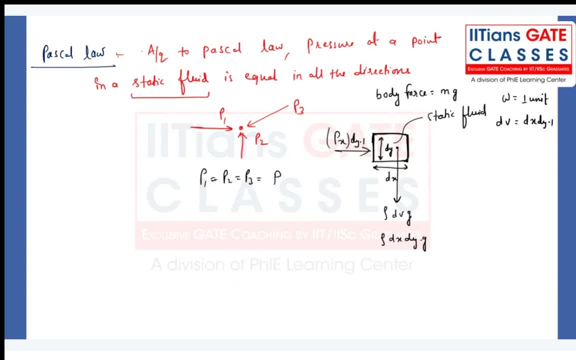 Px into dy, into 1.. Width will be 1, and here what will be the pressure value? Px plus dou P by dou x into dx, into dy, into 1.. There will not be any safe force, right, there will not be any safe force. getting my point. 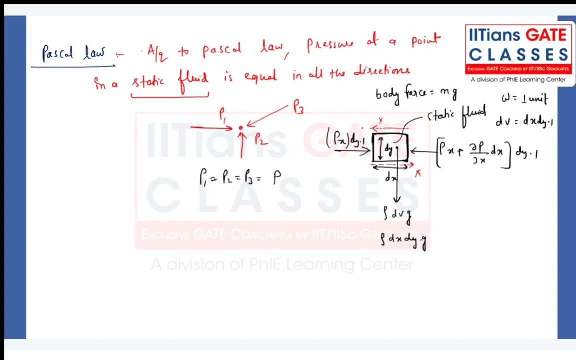 there will not be any safe force, agree with me or not. if the flow is not happening, why the safe force will be due there right now, But my different? This is the condition about this static fluid. this is the condition about this static fluid. 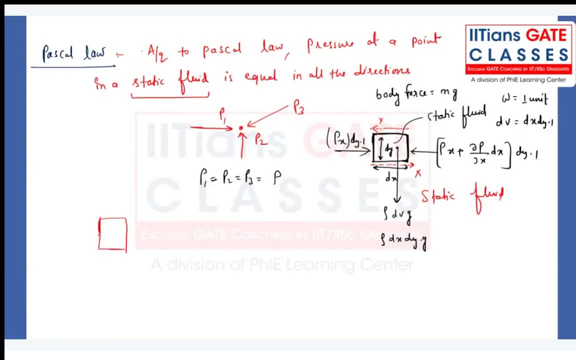 but if I will be talking about certain cases where the fluid element is subjected to some kind of torque, for example, right, that means the fluid is whatever. the fluid element is there in a container. this fluid element is undergoing certain motion, for example this: 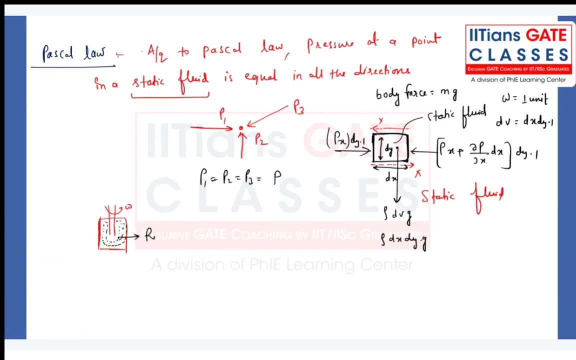 fluid element is undergoing certain motion, Rigid body motion for example. during that case also, you know, any shear deformation will happen. see that rigid body deformation means pure rotation. pure rotation case means you will come to know in fluid kinematics when I will discuss about that. you will come. 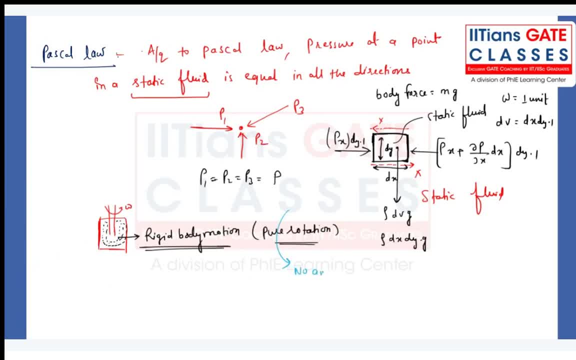 to know there will not be no angular deformations, no angular or shear deformations. Okay, Okay, Okay, Okay. When there is no angular deformations, my different, then what the safe force will do there? that is also zero. 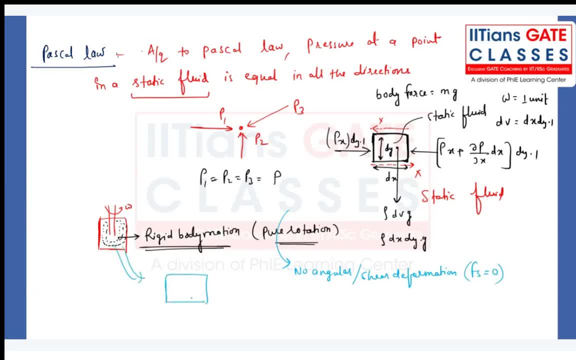 Once again, if we just draw the fluid element, once again there will be pressure force into dy px plus dou p by dou x into dx, into dy, into one. that will be acting. once again the share, what we call the share stress, that's again that is going to be absent. 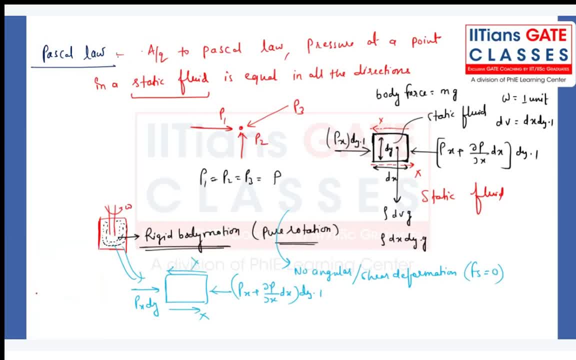 So once it once again it is going to be absent, Then what we can do? once again, the pressure will be same in all the directions, right? So this picture, whatever we have drawn for the static fluid, that is also applicable. 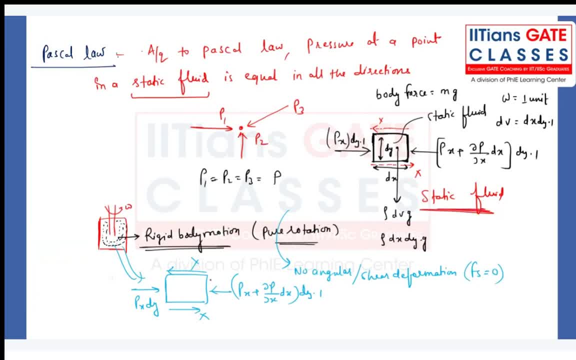 for a body fluid element which is undergoing a rigid body motions right, Make a note of it. Fluids are incompressible, so there can be no deformations, no incompressible fluid We can have. still, we can have that say deformations, you know, when it is under motion, getting. 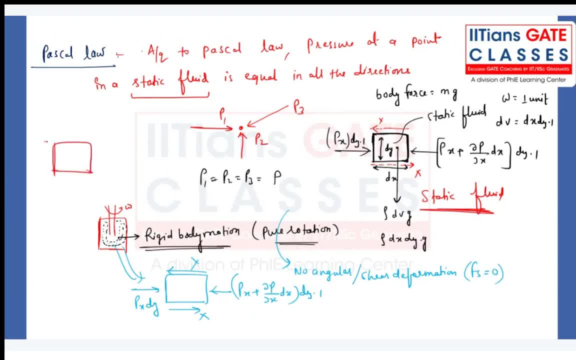 my point: whenever any fluid is there, when you apply a little bit, of say, force, it will start deforming continuously right See, in a fluid element there is a two types of. there are two types of deformations. Remember that one is a volumetric deformations. 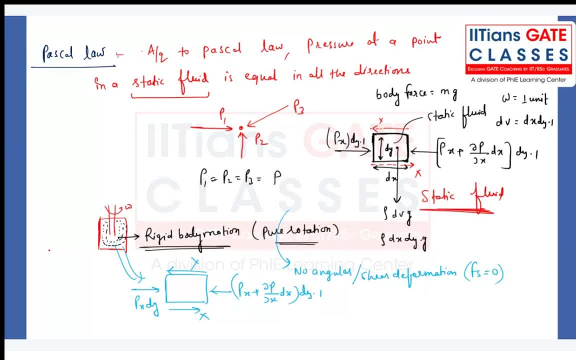 Volumetric deformations are happening because of the what? Equal amount of, say, stress, equal amount of normal stress, which is being present there, right? Or we can say, because of the normal stress, what is going to be happening there will. 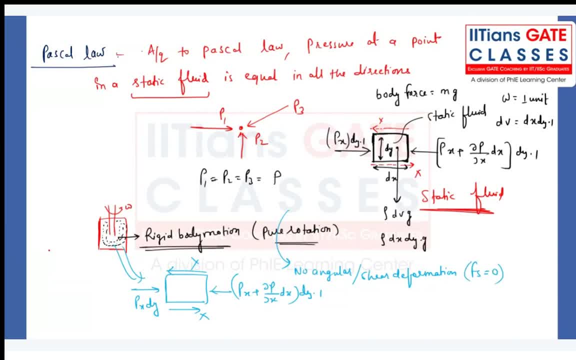 be some volumetric deformations Will happen. Second, there will be some say deformations right. Whenever we do the derivation of the Navier-Stokes, you know what we used to tell. whatever the normal stresses are acting in a fluid element, we try to denote it, basically categorize. 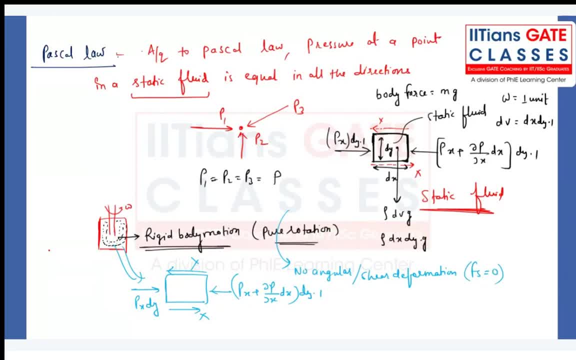 into two components. One will be volumetric deformation, Second will be, say, deformations. That's why you have, do you know the Stokes hypothesis? Tell me, guys, Any one of you know about the Stokes hypothesis? Till now, we discuss only first coefficient of viscosity, that is, dynamic viscosity, right? 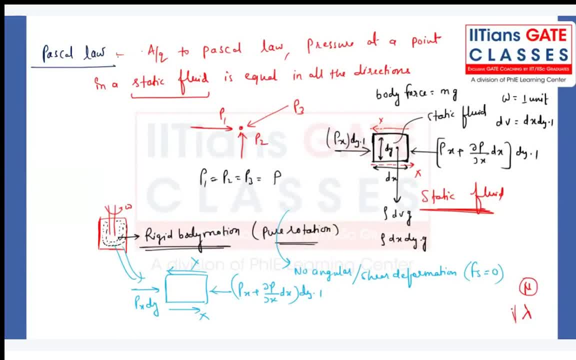 We have not talked about what Second coefficient of viscosity that is lambda, right? That is basically denoting this is denoting the say deformation. This will denote volumetric deformations of the fluid element, right? So this basic concept and understanding must be there when you're basically dealing with 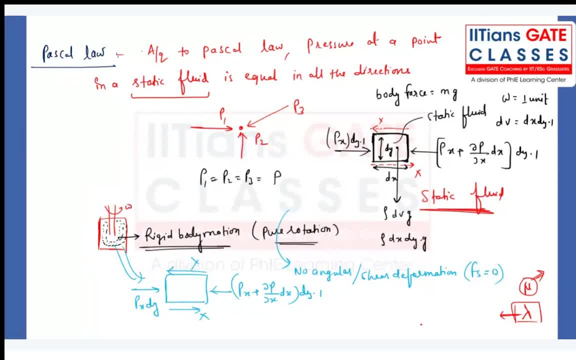 the derivation of the Navier-Stokes, The derivation of the Navier-Stokes or basically what Any other equations, right? So remember, any fluid element. you say you take any fluid element and whenever you just apply, let's say the, this fluid element is under what motion? right? 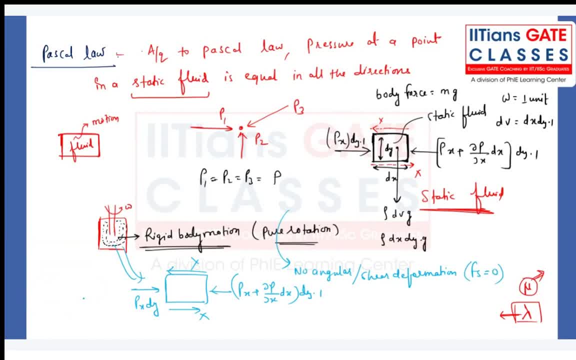 So what we used to do, we used to categorize into two things. One will be: we treated like there is a hydrostatic state of stress, where it is being subjected to equal amount of pressure value in all the directions. Second, we say it is undergoing volumetric deformations. 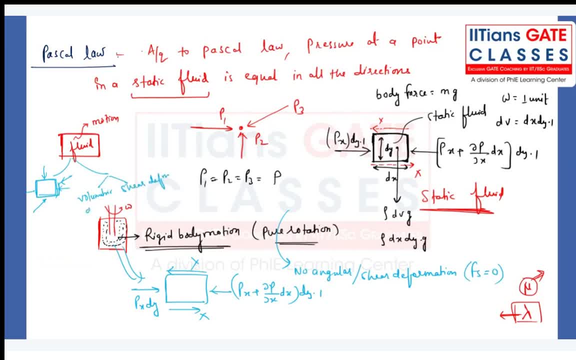 It is also undergoing shear deformations, right, And likewise we used to determine the Navier-Stokes equations, right? But again, volumetric deformation will be zero. for which case, tell me guys? Volumetric deformation will be zero. for which case? 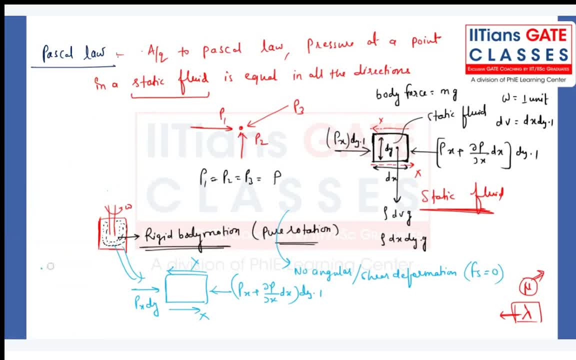 That is a very, very obviously right, Right. Okay, That is a very, very obvious answer. Right, Very, very obvious answer. All of you can answer that, Whatever the fluid is incompressible, there will not be any volumetric deformations. 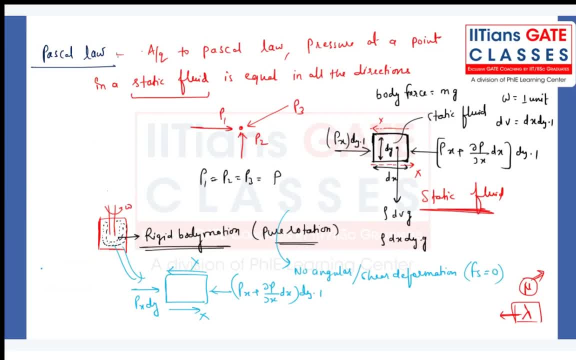 They can be only shear deformations. right Volumetric deformation means what dv by v, that is minus d rho by rho, Incompressible means this will be zero. This will also be zero For a fixed mass volume into density. when you differentiate that, this equation we are 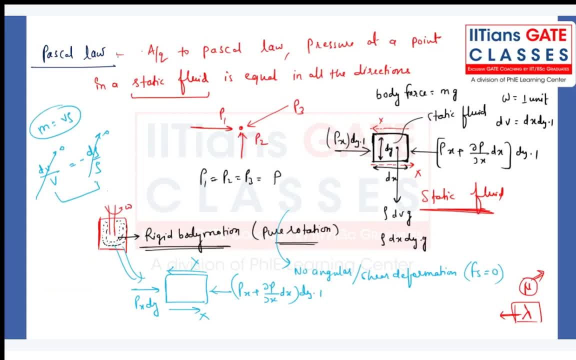 going to get So totally. we can say, for an incompressible fluid, Right For an incompressible fluid, the volumetric deformation will be zero Again. you might be thinking, sir, you are talking right now in the air. you are not. 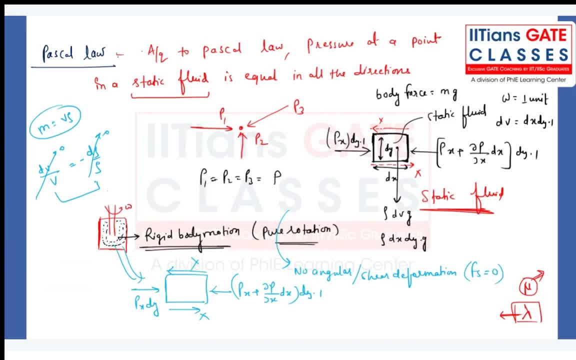 writing anything. So what the hell we are going to do that, How we can learn that, No need to worry, Include kinematics. Once again, I will discuss and maybe, if I will not do the derivation of Navier-Stokes, other aerodynamic faculty will do that. 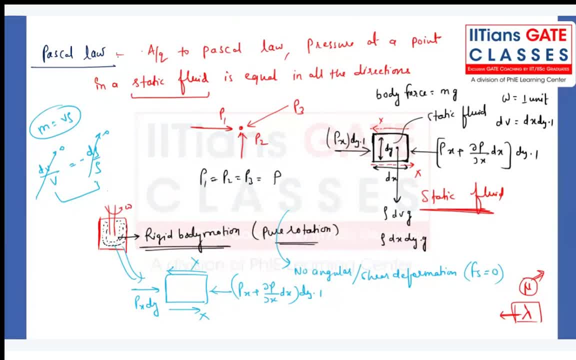 But you must understand what are all the steps involved there while doing the derivations. Not only we have to learn the derivation, we have to understand fundamentally also why these terms are coming, why that term is not coming. Because for a compressible fluid, whatever the Navier-Stokes equation, you know right. 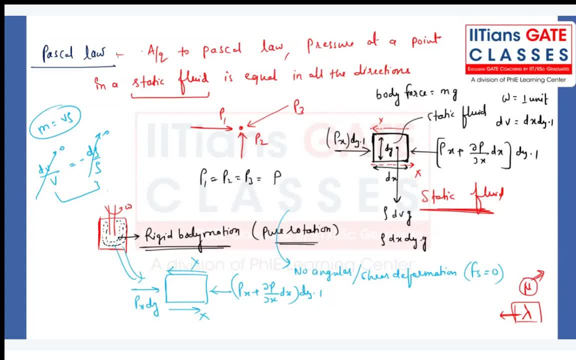 now that may not be true, Right? Because in that case we have to again for a Stokes hypothesis, even for a compressible fluid, we say this compressibility effect will not be considered. Right? There are many situations. 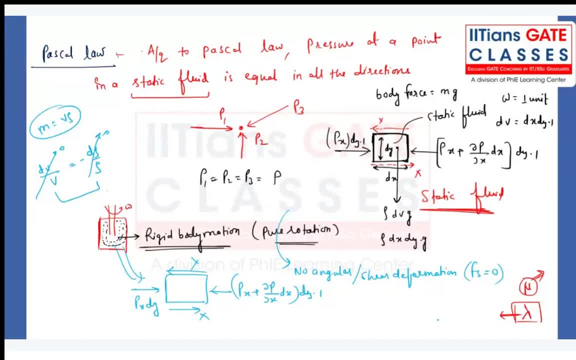 I will discuss that separately, You know. So maybe if extra class will be permitted, I will take that derivation also, Because that is a very, very important for being a fluid mechanics expert that we should know about the Navier-Stokes fundamental things. 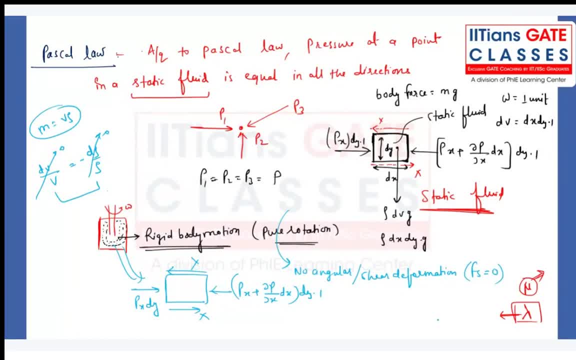 Right Fluid rotation, we are saying the rigid body motion. because here see, understand rotation is not only right now what you are understanding by rotations. tell me, guys, what you are understanding by rotations. Rotation means whenever the fluid element you take, for example, when you take the fluid, 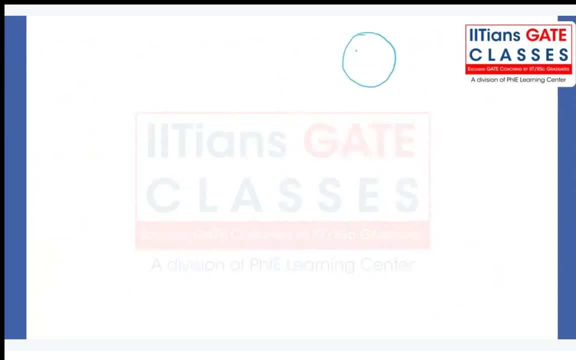 element like this, For a fluid element. suppose, and on a fluid element you are applying shear force like this, And when you take the radius, you know there will be some kind of torque onto this fluid element that is forced into radius. My dear friend, not this shear force is acting. 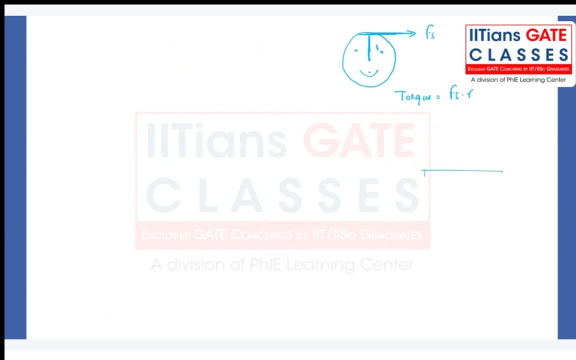 And you know that whenever the fluid is flowing, for example flow over the flat plate, there will be some boundary layer formation. There is a some boundary layer formation on the sociedade. So let me just, if I had an example here, I could say that let say a fluid is going. 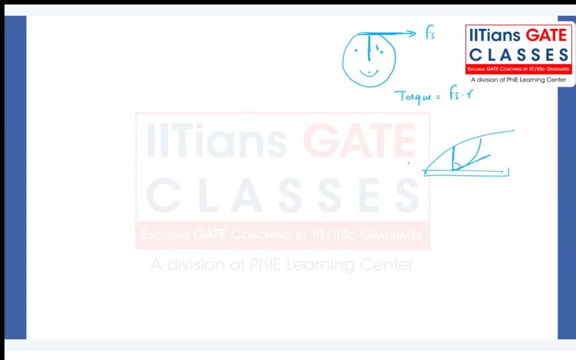 velocity gradient. as you can see over here right now, even though fluid is having viscosity, even though it is having what du by dy right, so definitely there will be some shear force, mu into dou u by dou y into area, so definitely shear force is there and radius of that fluid. 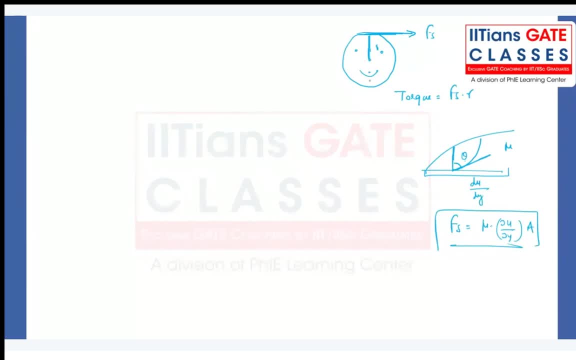 element will be there, so that will create the rotations. so one thing you are so sure about the rotation is that viscosity is responsible. what will happen? but that is a wrong statement, that viscosity is only responsible for the rotation of the fluid. the fluid can also have the rotation. 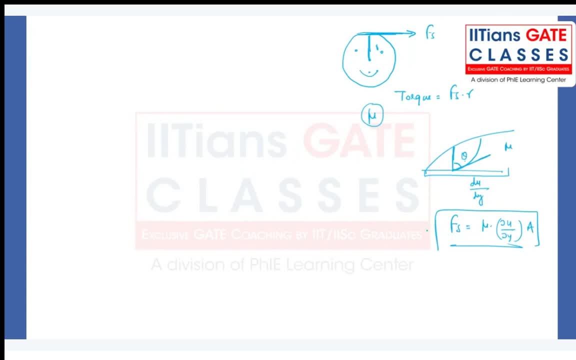 is still. the shear force is zero because- see what we are writing, even though fluid is having viscosity. but dou u by dou y will be zero. why it will zero? pure body rotation. suppose fluid element is there in a container and i have just applied some torque like this, with the help of this: 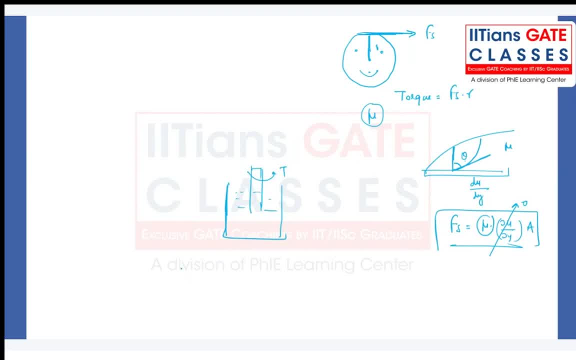 one. what will happen? externally? we are rotating, even though the region of the fluid element is not having shear force. that is zero, because not the viscosity is zero, viscosity is present, but dou u by dou y is zero. pure rotation means there will not be any shear deformation, only rotation. 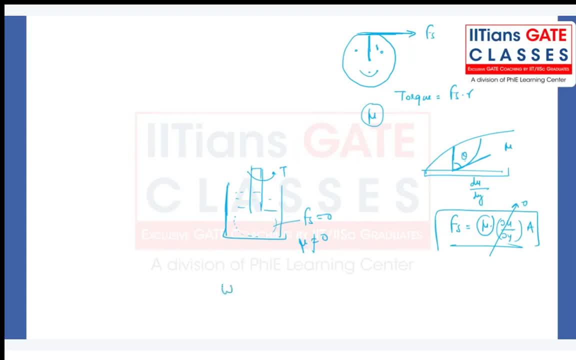 will be there, why and how, with the help of omega formula and all i will discuss separately in the fluid kinematics. if i will discuss right now, you will say, sir, fluid statics, you are discussing fluid kinematics, you are mixing, you are confusing. so that's why i'm not giving you. 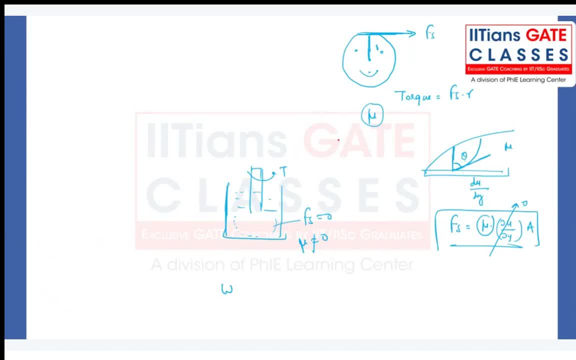 any information about the rotation of the fluid element and all i will discuss separately in the detail. i'm telling you, even though i'm telling you that the viscosity is not the only parameter which is responsible for the fluid rotations, even though you have the viscosity but you don't have 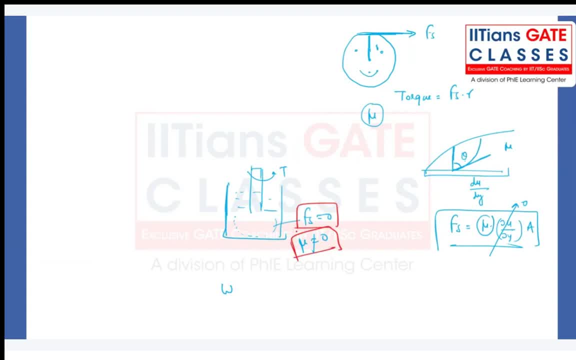 this air force. you know then what will happen? still, you have the rotational effect in the fluid element. because of what? external torque, externally, you are providing some kind of rotations inherently by the nature of the fluid, he, he, the particular fluid element is not able to rotate. he is saying that i am not able to rotate by 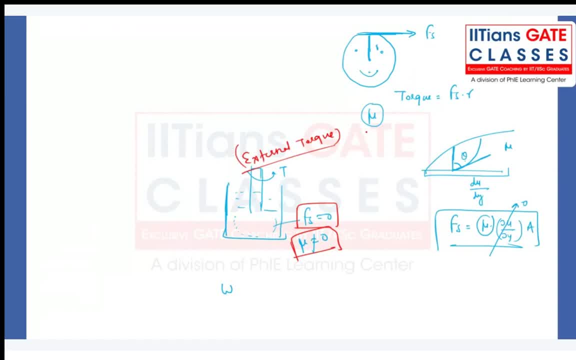 by my own. so what, what? you will say: no, no, i am rotating you. you need not to rotate yourself, i am rotating you. so that is what the rotational effect will be: coming into the picture. this is nothing but something like a you know, uh, what we say? pull is there, or any ball is there which is. 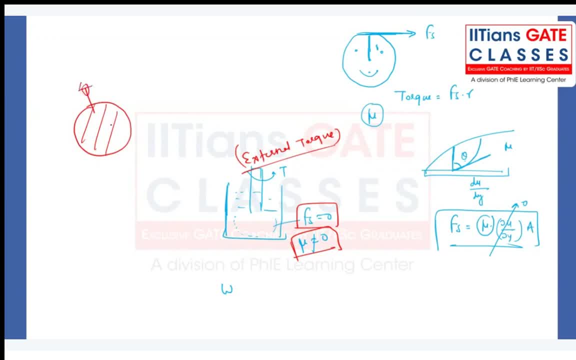 being hanging, for example. you know, and we are just applying some kind of- or maybe we can just think of something like this- we are applying some kind ofity into the 5 J To the disc, we are applying some kind of torque. So this is a solid body, this is a fluid element. that's why we say solid body rotation case. 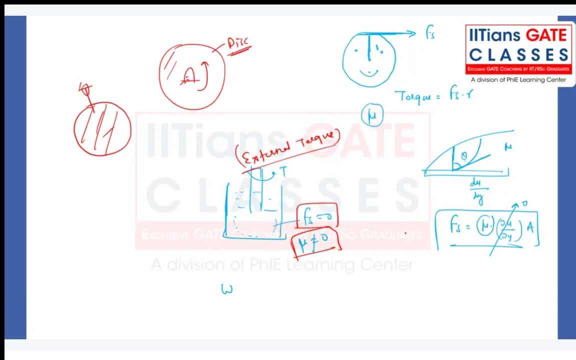 The pure, whatever the pure rotation is there, or that's why the name itself is there. What is the name Rigid body rotations? because disc in engineering mechanics we are dealing with the rigid bodies, So that's why the name is has been mixed there. that rigid body motions is a clear all of 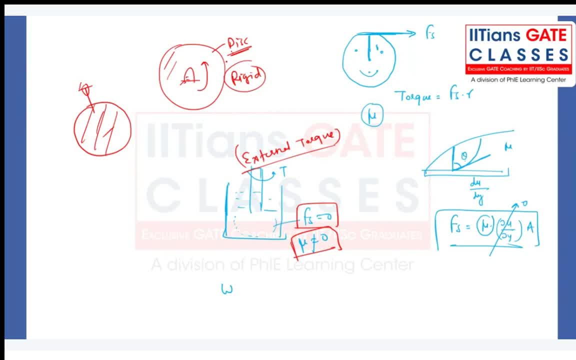 it. We are not. we are treating the, whatever the fluid element just like a solid body. Not exactly they are solid body, but we are treating like that. is that clear all of you? Because until unless we talk about the fluid element, we say there has to be some shear. 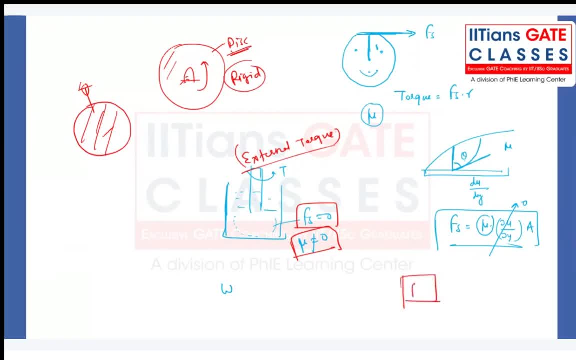 deformations. That's why the flow is happening. See that this is a fluid, this is a shear force we are applying and we are saying there is a continuous deformations and that's why we are saying there is a flow right. So again, you might be thinking so, if you are talking about the fluid we are talking. 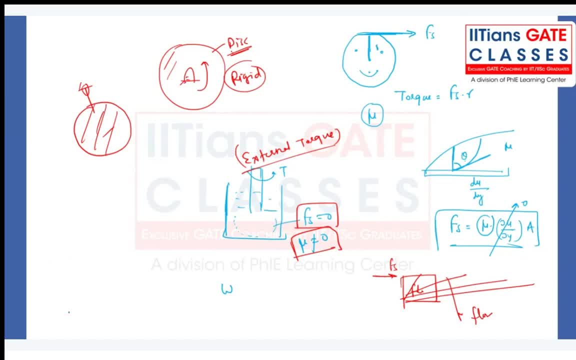 about the motion, We are not talking about the flow, We are not talking about the shear force. Then why the hell we are discussing in the fluid mechanics? We are applying some kind of external torque, just like a solid body. That's why the name has been given solid body rotations, solid rigid. getting my point? 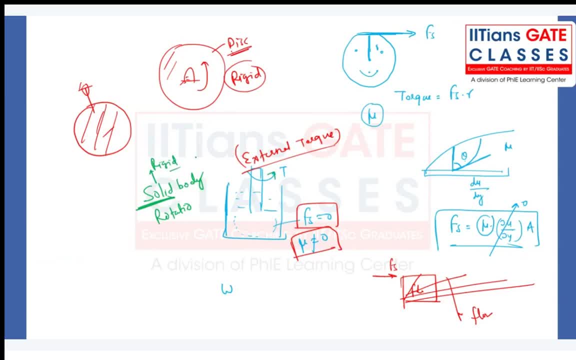 Is that clear, all of you? Okay, Thank you, Bye, Bye. See you in the next class, Bye, Bye. So yes, make a note of it. So remember: for any fluid there can be volumetric deformation. There can be a shear deformation for an incompressible fluid, straight away. 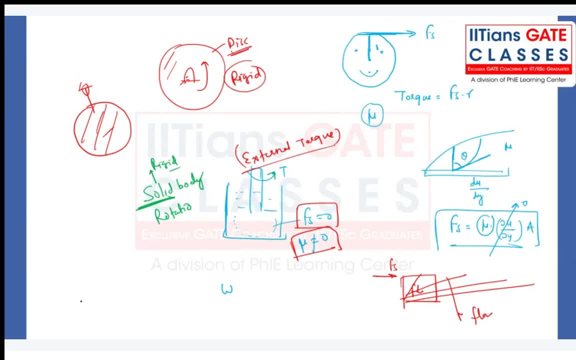 We disregard the effect of volumetric strain rate or volumetric deformations. Getting my point? See the solid body. you are talking about volumetric strain rate in a pure rotation. pure rotation once again. which kind of fluid? whether it is a compressible fluid or incompressible. 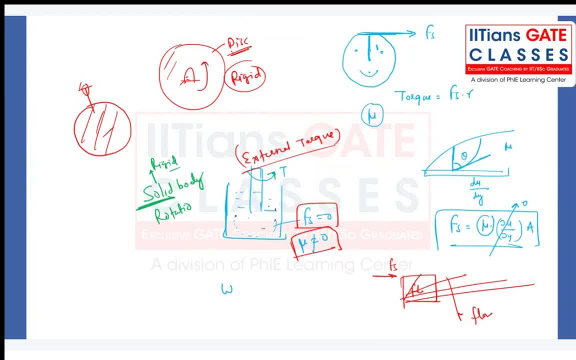 incompressible. again, that is zero. getting a point now. so please make a note of my each and every word, because at the time of fluid kinematics or fluid dynamics, little bit i will discuss, not in detail, because i am putting my here time. i am giving some time to this topic. that's why i'm gonna put some less amount of time during those. 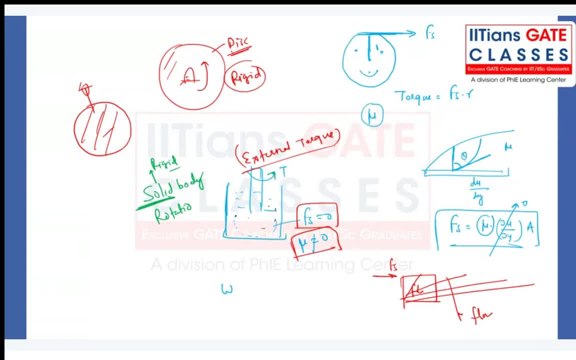 basically topics. now let's discuss some of the fundamental of fluid mechanics. by newton's second law, what are all the forces that is being encountered by the fluid element when it is being subjected to different, different types of forces? so i'm not deriving navier-stokes right now. i'm just giving you little bit of hint. 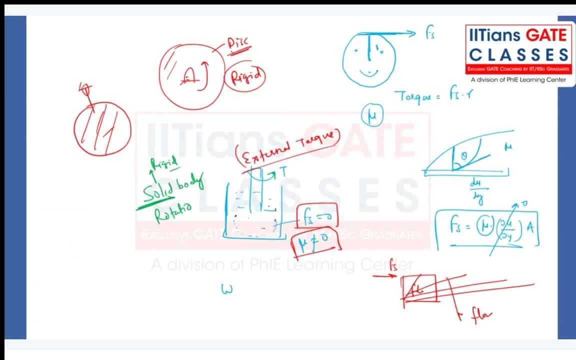 so that you understand each and every terms in that equations. because when you know navier-stokes equation your life will become very easy. if you don't know, very complicated life will be. any problem you will face very difficult to solve by without solving the navier-stokes equations right, with the navier-stokes automatically. 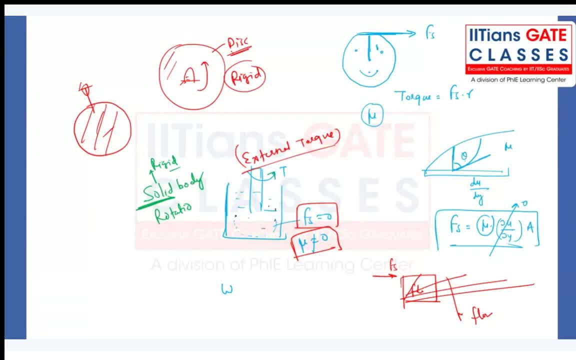 problem comes out of the equation. so i'm not deriving navier-stokes right now. i'm just giving you a chance to watching this video and try to assume. maybe you can solves in three steps or so. tried being from this page only. there is a one statement. you know: inviscid flow. 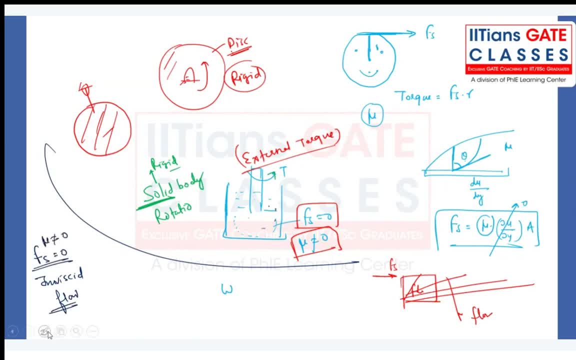 what is the meaning of inviscid flow? share force is zero. viscosity is not equal to zero. inviscid flow always be irrotational flow. there is a one statement, they used two. they already know the pepp brand from pepe, from Johannes sites, nick zeppelin from precis's. 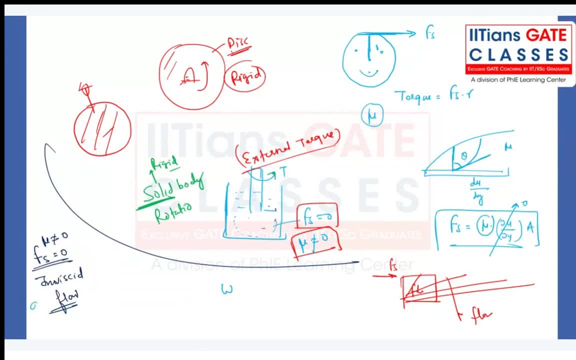 to give in examination that: do irrotational flow do all inviscid flows? do inviscid flow always gives irrotational flow? Irrotational means omega will be zero. omega will be zero. that means no rotation. right Fluid element is not being rotating. That is the first statement. 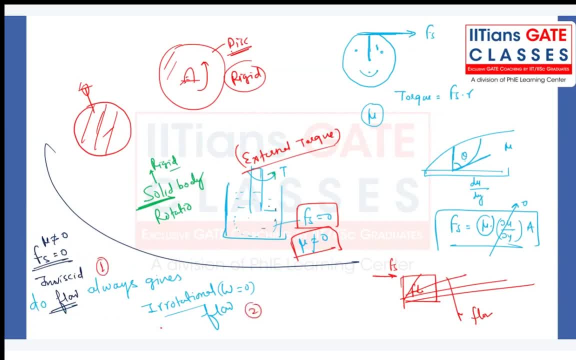 right. Second statement you will encounter that do all irrotational flows gives inviscid flow. So for this two question, we have lot of motivation to study fluid kinematics. right, because for every topic you are studying, you are investing your time, you are attending the classes. definitely some motivation is there. 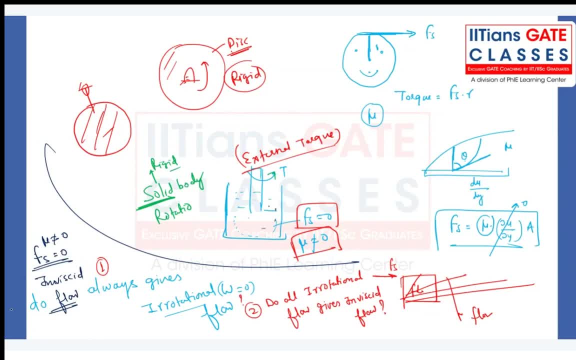 right behind that. you are not coming just for seeking the formulas, seeing the particular, noting down the derivations, noting down this definition, because that is all there in the textbook. I'm telling you you go and read that, but you may not be able to understand even single line also, but after my classes, definitely you. 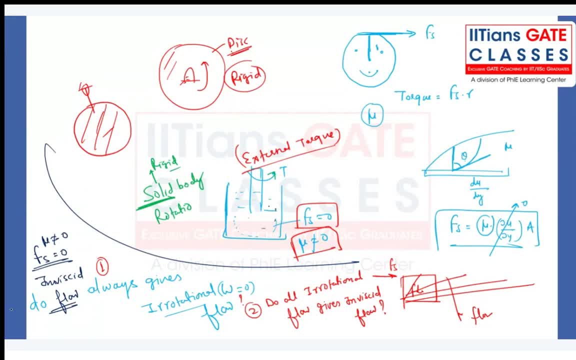 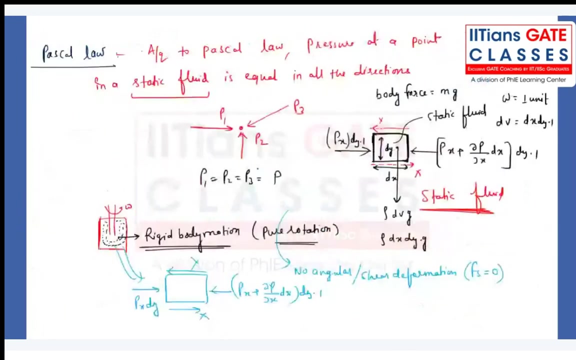 will enjoy learning those paragraphs. within fraction of second, or maybe hardly any time you will put from your end, you will be able to finish one complete chapter of that book right now. so, after noting down this thing, is it complete? all of you have noted down. so we have discussed the Pascal law. we have discussed the rigid body motions. 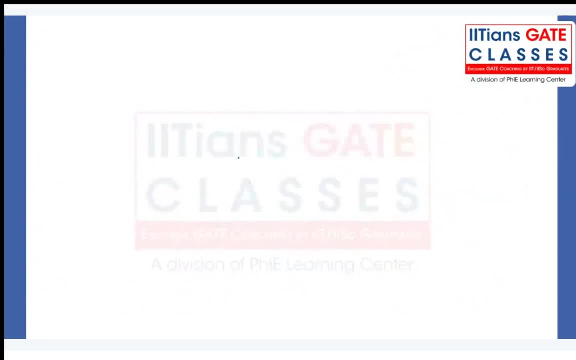 now just note down the fundamental of fluid mechanics. now the fundamental fluid mechanics which I'm going to tell you is that suppose there is a fluid element which is being subject to do different, different poses. this is a liquid molecules. no, every inviscid flow will not be irrotational flow. inviscid flow can be. 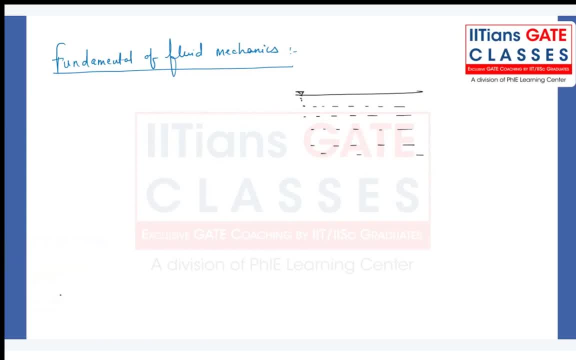 can be rotational flow also, just like a solid body rotations right. we have discussed that. inviscid flow means shear force is zero, but it's still be externally we can provide some rotations. right, inviscid flow means when shear force is zero, we say inviscid flow. 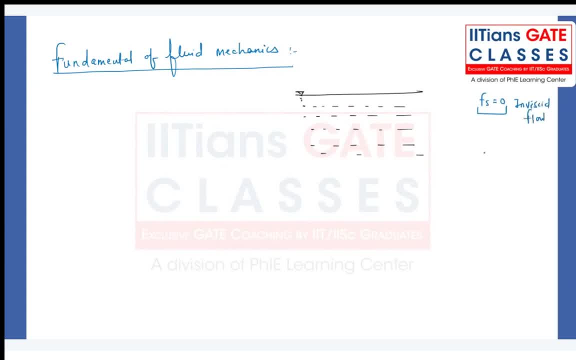 When viscosity is zero, we say in, we see fluid, No viscosity. In means what? No viscosity. We also say ideal fluid, This we say ideal flow. Ideal flow may be possible, but ideal fluid will never gonna exist in real life. 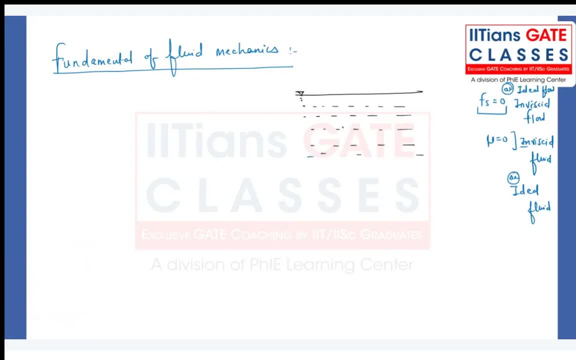 Now let me draw the fluid element. If I just draw the fluid element from here and if I zoom it, then I will be basically taking one cubical element, because that is a very easy save in a Cartesian system. So those who are having confusion about the solid body rotations and whatever I have discussed, 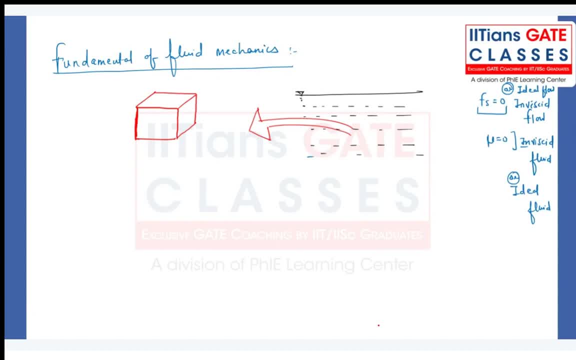 volumetric deformations, Seyer deformations- all those things will clarify automatically as we progress towards this levels. No need to get panic at all over here in the fluid hysterics or why we are discussing about those things. I would like to give you some idea about that and whenever we are discussing any topic. 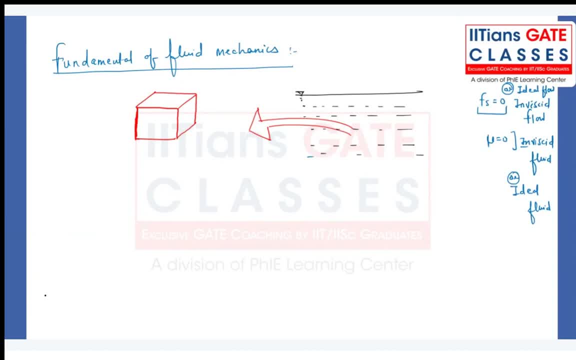 it is not necessary. It is only that you should be stop thinking about some other topics or maybe other zone, that is, fluid dynamics or fluid kinematics, Because after fluid is statics, which picture will be started? Fluid kinematics only it will be started. 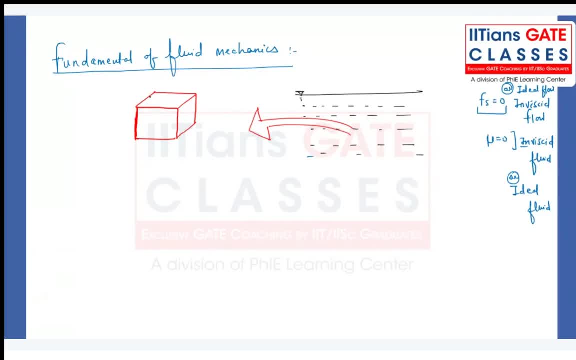 Fluid dynamics only. it will be started Now, because when I say about your aircraft, which is flying at a particular altitude, you will never say how the motion is happening, right. You will always deal as a aircraft. You will never say how the motion is happening, right. 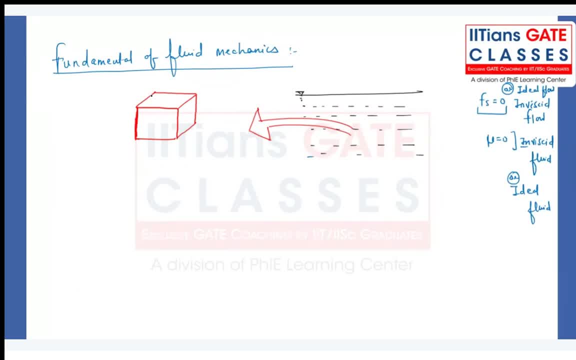 You will always deal as a aircraft aerospace engineer. what are all the forces will be acting for that? only you will be paid. you know you are not going to be paid, sir. how you are not going to be paid, how the diagram will be, whether it is a delta wing, whether it is a diamond wing, whether it is a some aerofoil shape, whether it is. 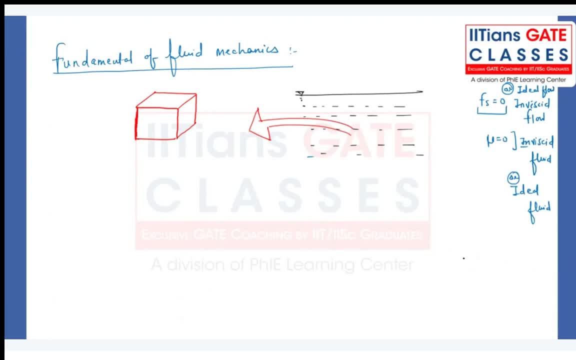 some normal uh subsonic airplane or maybe supersonic. you will not be there for that purpose. you, as an engineer, you will be there. what are all the forces you will be encountered? that that is what we are discussing right now. now, so any body fluid element will be subjected to. 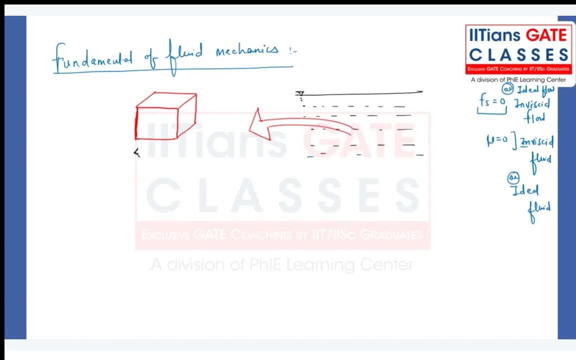 different types of forces. let's say: this is a dimension dx, this is dy, this will be dj, this, this, this will be my x-axis, y-axis, this will be my z-axis, any forces you will encounter here, net force, whenever you use to write mass into acceleration. 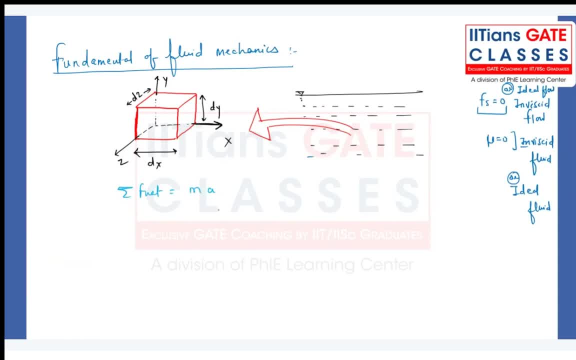 acceleration can happen in x, y, z directions. right now, what are all the forces will be acting? the first one will be surface force. second one will be body force. first force will be discussing here is that surface force. what are all the surfaces forces will be acting on a particular surface. 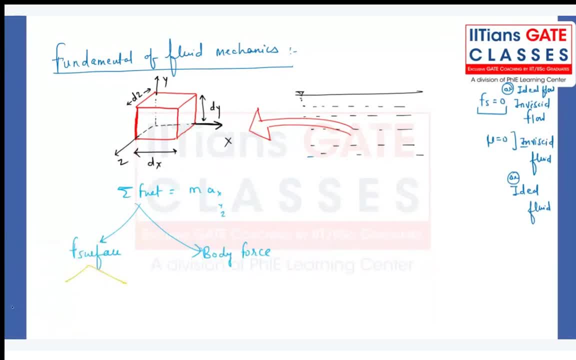 tell me guys, one will be pressure force, second, one will be viscous force. and what are all the body forces? of course, weight of the fluid element. and what are all the body forces? of course, weight of the fluid element right now, as far as the fluid is under basically what? in a motion conditions, we, and in a month, 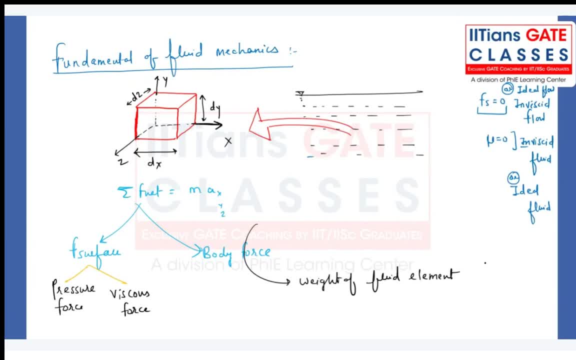 basically what you know: motion conditions. we are dealing with these types of forces. one is the pressure force, second will be viscous force and third will be body force. know what is the body force? the body force. we are dealing with different types of forces. v digeste. 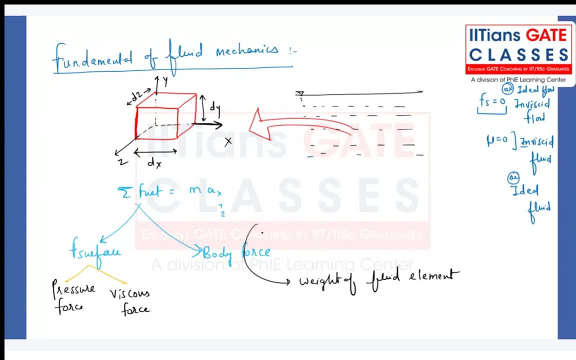 force. now, what is the body force? so body force we are denoting by mg, that is equal to what rho into what is the volume of that element? what is the volume of this element? i am considering a small volume of dv in a whole liquid molecules. volume of this element will be what? 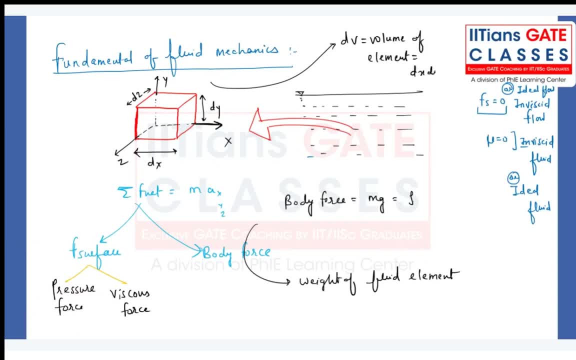 dx, dy, dz. right. so volume of that fluid element will be dx, dy into dz, right into g, right. so my different, what i can say: body force per unit volume. if i want to write, then what i can write: dx, dy, dz. this will cancel out. so what will be my body force: rho into g. 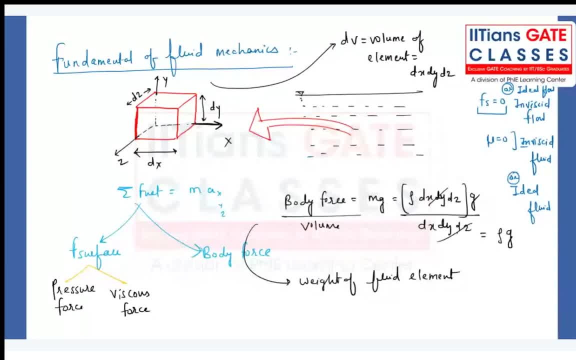 is that clear, all of you? now? body force that can be acting in x direction, of course, as of now, whatever the figure you are looking right now, definitely the body force will be acting only in the y directions. right, there will not be any body force in x or z directions. but for the sake, 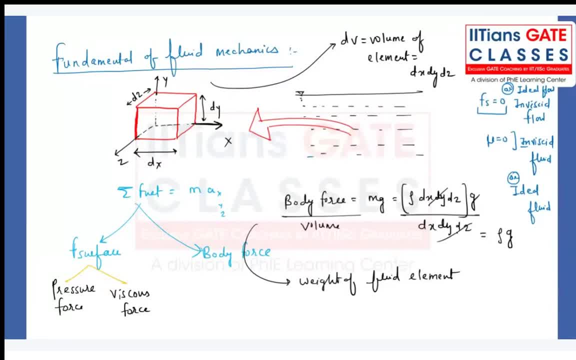 of generalized case. i am just telling you: the body force can be acted over here in x, y and z direction. let's say the fluid element is in an inclined plane, for example. in that case this is the body force: rho into g. but if you just draw the component, both the components will be acting. 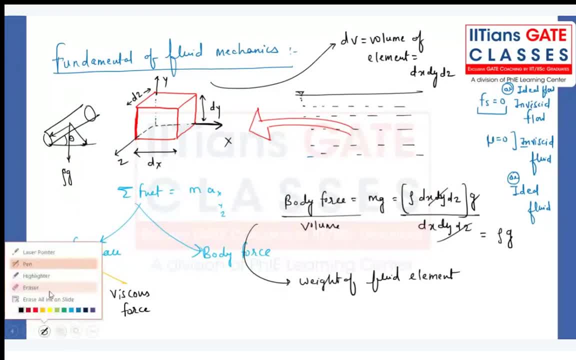 you know. so, for a very generalized case, i am talking about the body force that can be acted in the y, z and x directions. make a note of it. so all of your understanding, or not? tell me, guys, is that clear? all of you, the forces which is being subjected to. 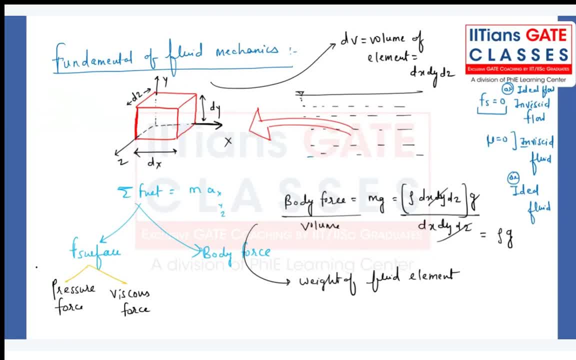 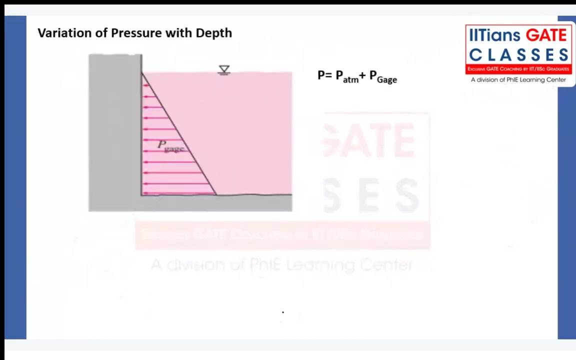 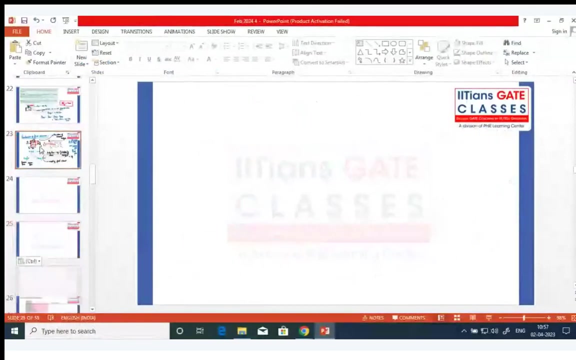 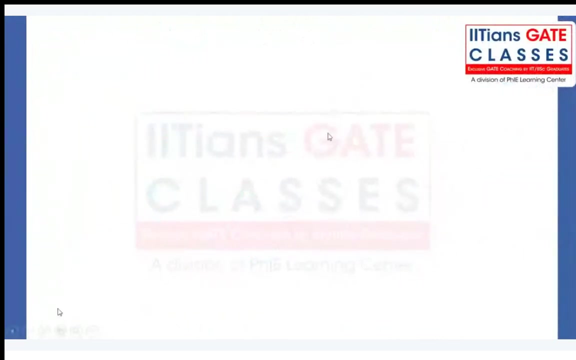 which is being subjected by the fluid element, because you will be having only pressure force and this air force. you know that viscous force. only in later part of the discussion, in the fluid dynamics, we say that drag force. then can i move to the next segment, the fluid element which is being subjected to. 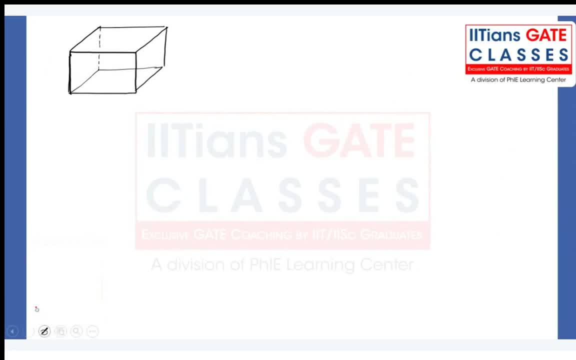 body forces. that is sorry. pressure forces will be what? in X direction? if I just write that is P into dy, into dz, because this is what dx, dz and this is what we have dy. so what is the area on which it is acting? dy into dz, and what is the pressure force in this direction? P plus dou P by. 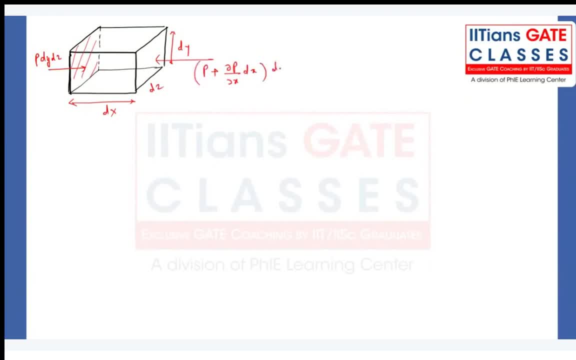 dou x into dx, into dy, into dz, pressure into area that will give me the force right. and what are all the sales stresses? what are all the sales stresses- my different- in a particular fluid element. what you have observed above the plate is there which is being subjected to force F, and there is a fluid element. 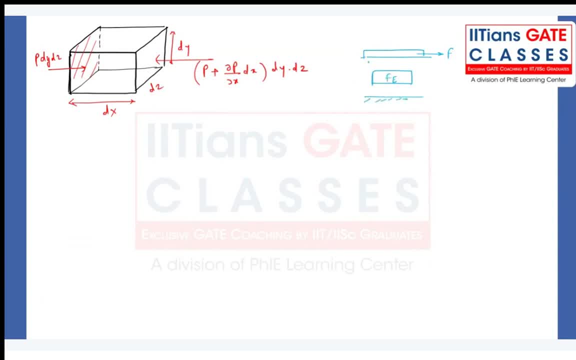 so, generally what you have encountered, generally what you have seen, that when the force is acting like this opposite direction, there is a one force onto the fluid element, here like this, and here it is like this shear force. Once again, here it is shear force, here also shear force. 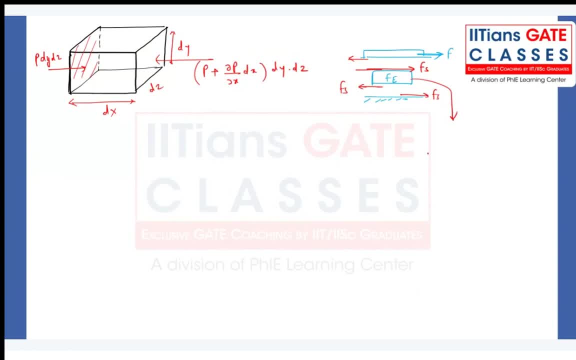 So if you just take only fluid element and if you draw the free body diagram, so what are all the forces will be acting: Shear force. how to write this shear force? So one will be this one right. Second one will be this one, this one. 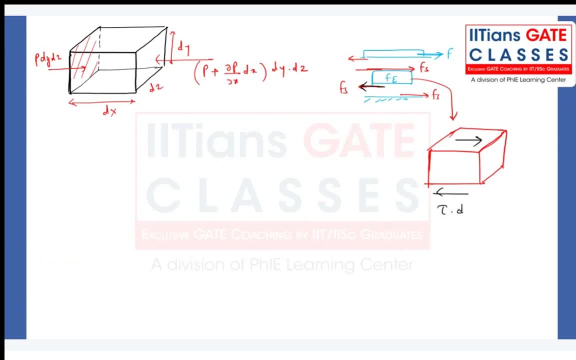 What is that? Tau into area, tau into area dA, What we can write On which area it is acting. On this area it is acting. What is that area dx into dz? and on the top of that, when you just move towards the distance of dy, what? 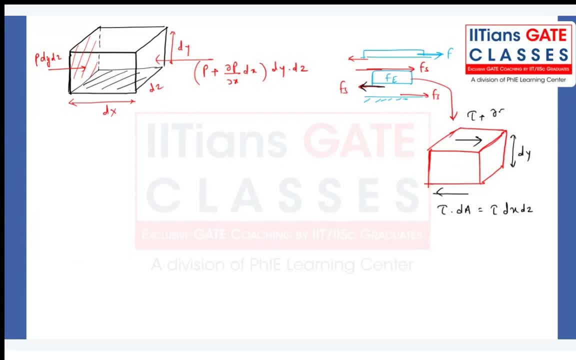 are all the forces will be acting: Tau plus tau t by dou y into dy, into area. What is that? Tau plus tau t by dou y into area, dx, into dz. Now, why the direction is different, It is being clear by the free body diagram. 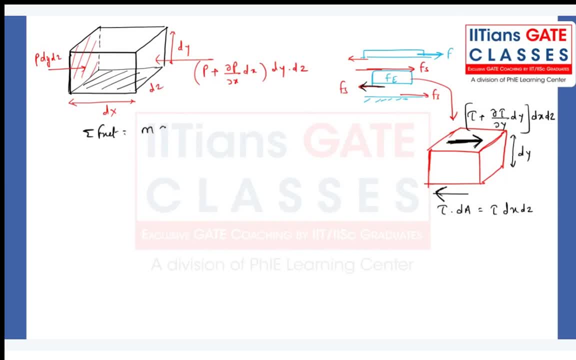 So the net force in the direction of motion that is equal to mass into accelerations. I am writing x momentum equation In the direction of motion. what is the motion? Let us suppose in these directions, So p into dy, into dz, Minus p plus dou, p by dou x into dx, into dy, into dz. 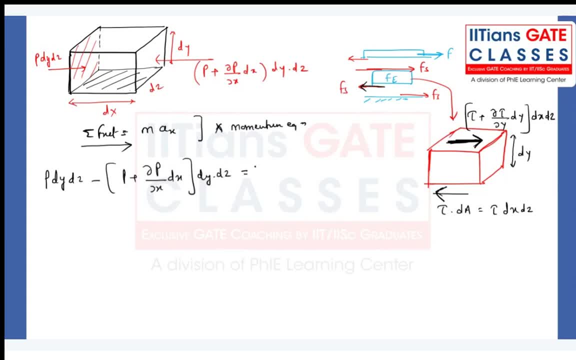 That is equal to mass, into acceleration. But mass, I have told you that. what is the mass value we can write. And one more force is there, shear force right In the direction of motion, plus tau, plus dou t, by dou y into dy, dx, dz, y plus, because 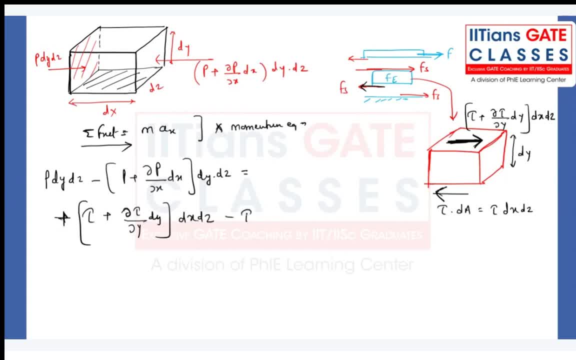 it is acting in the direction of motion. Minus tau t by dou x into dy, into dz. Minus tau into that can be written as that can be written as mass into accelerations. So mass can be written as rho into dv acceleration in the x directions right. 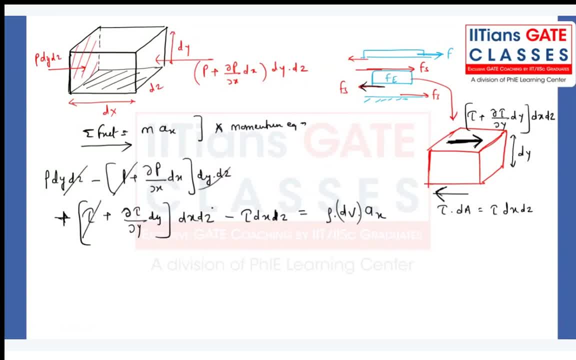 So this will cancel out, Right, Okay, Okay. So this is going to be left out. Minus dou p by dou x into dv, plus dou by dou y of mu into sorry. here we can write directly. I have written. 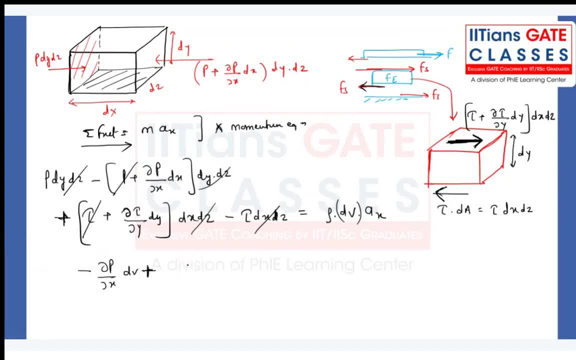 We can write dot u by dou y into dv. Okay, Okay, Okay, that is equal to rho into dv, into ax dv. dv will cancel out. so what we can write. we can further write minus dou p by dou x plus. now, assume some body force also in x direction. assume some body force also. 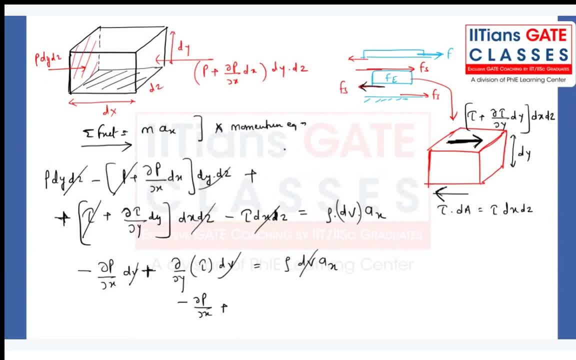 in x direction. what is the body force? tell me guys, what is the body force? rho into what we can write, because we already- only we- have considered the pressure force and the shear force, not the body force. what is the body force we can write, my dear friend? 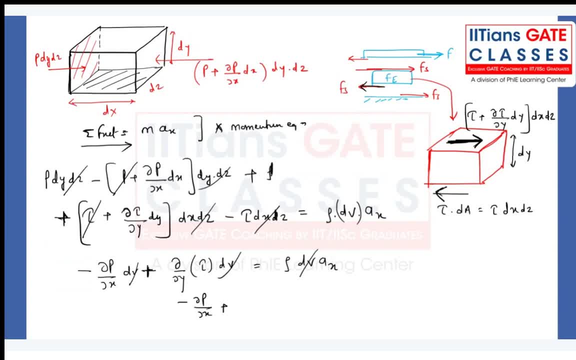 the body force. for example, we can write bx into dy, bx into dv, so here we will be having bx also plus bx into dv. this will cancel out. so dou by dou y of tau plus bx. that is equal to rho into ax, where bx is what body force per unit volume. 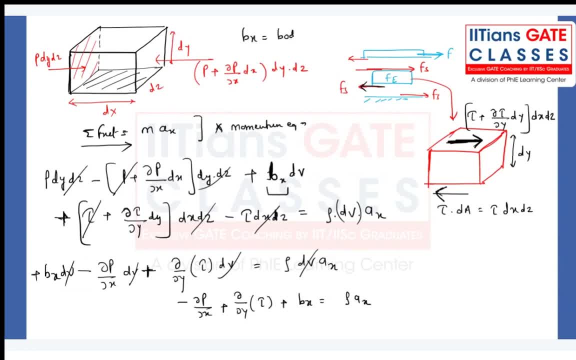 body force per unit volume correct. so what you are getting, my dear friend? and here we are discussing about the newtonian fluids. so tau will be what mu into dou u by dou y directly. we can write du by dy, or we can write dou u by dou y. 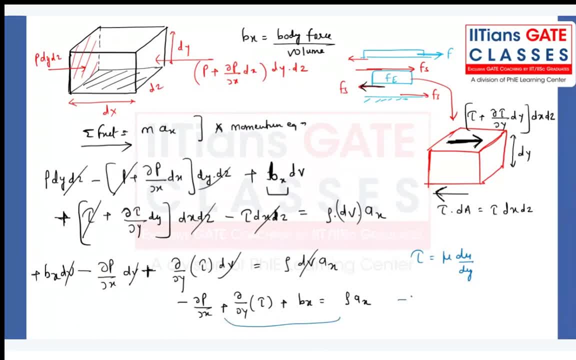 So here you can write further this equation: when you simplify minus dou p by dou x plus dou u by dou y mu into dou u by dou y plus bx, that is equal to rho into acceleration. So you are see, I am not deriving any momentum equation or Navier-Stokes equation. 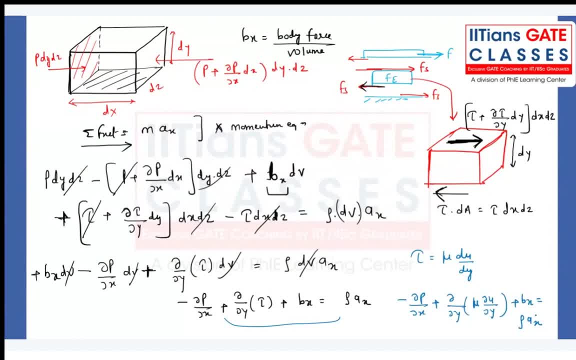 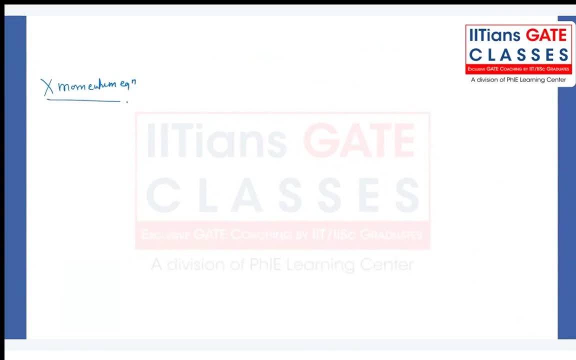 I am just telling you at least how you are getting terms and terminologies into that equations. At least you can feel that For that purpose. I am telling you right, In a bigger picture. when you write the x momentum equation right, when you do the complete derivations, you will be having this equation: minus dou p by dou x plus mu, dou square u by dou x square plus dou square u by dou y square plus dou square u by dou z square plus bx, that is equal to rho into acceleration. 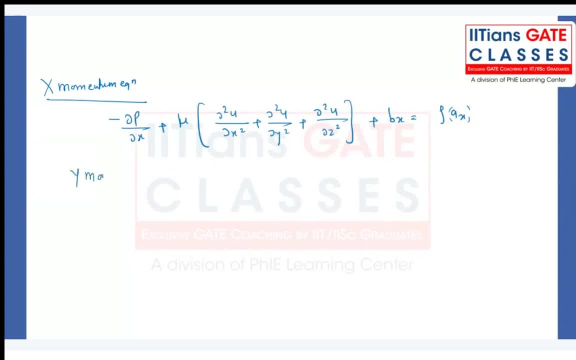 Right Right Y momentum equation when you write minus: dou p by dou y plus mu into dou square u by dou x square plus dou square u by dou y square, dou square u by dou z square plus b y rho into ay Right. When you write the z momentum equation: 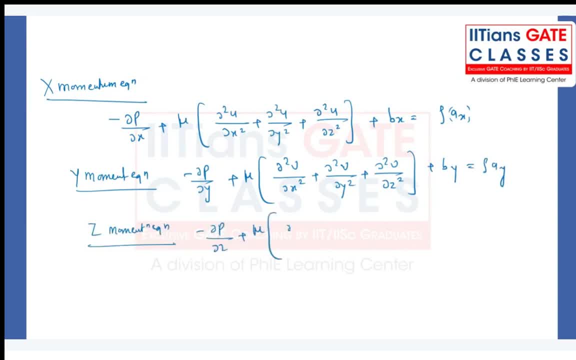 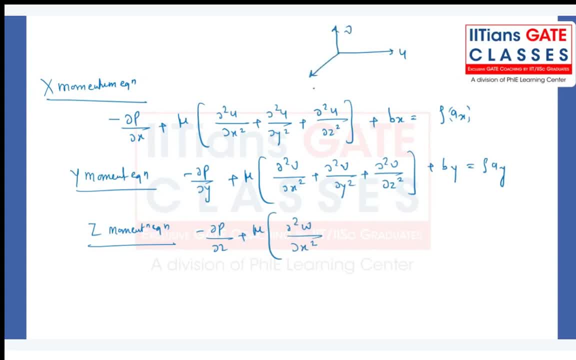 v is the y component of velocity And o is z component of velocity, Plus bz, that is equal to rho, into acceleration in the z direction. So you might be thinking, sir, you have done the derivation, right now only we are getting this term, this term, this term. 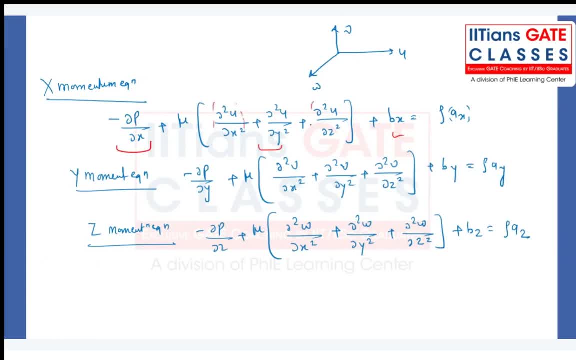 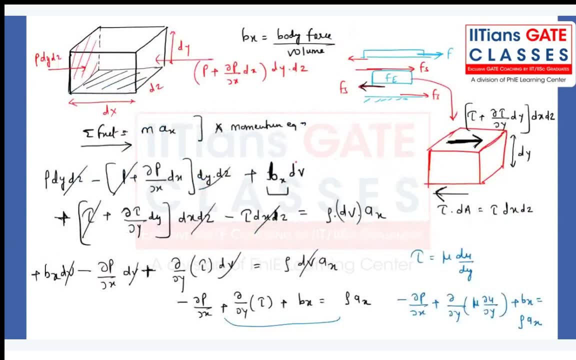 and this term. what about this term, sir? see, I am telling you, when you do the full derivations, then only you will be getting the, you know, complete terms of Navier stokes equations. right now I have derived only few terms you know, so that at least you will be getting. 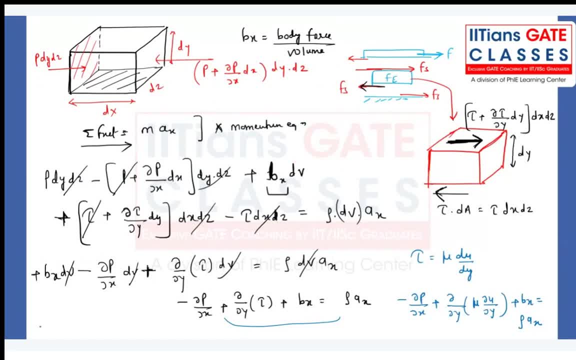 idea how those terms are coming right. my purpose is to tell you that this is nothing but pressure, this is nothing but viscous force, this is nothing but body force and the right hand side. this is nothing but actually telling you the acceleration mass into acceleration or inertia force. just make a note of it. 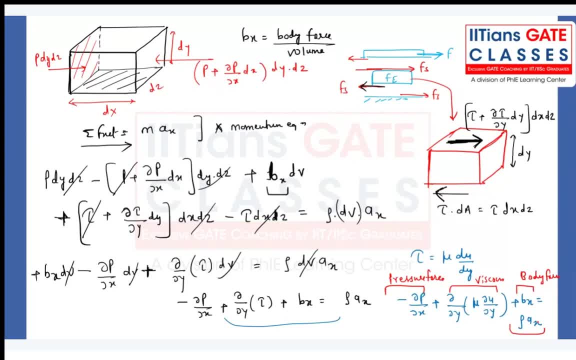 you. it is just that we are discussing pressure force and all per unit volume, per unit value, per unit volume. is that clear how the terms are coming? when you do the actual derivations, you know a big five page derivation is there in that you will be getting each and every term. but right now, for the sake of understanding little bit about, 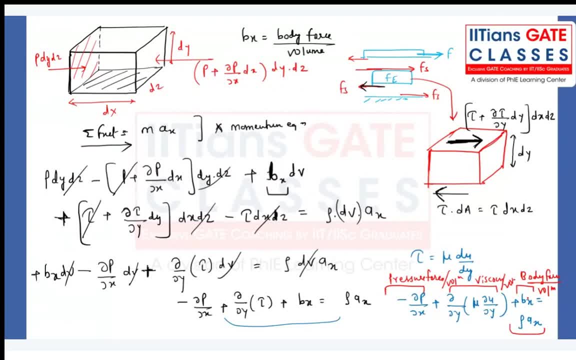 the nearest stokes i have taken about these cases. and now, what are all the assumptions? first is: concept of continuum has to be valid. second is: we are assuming, we are assuming whatever the equation we have written, that is only valid for newtonian fluids, because we have replaced this tau with this. 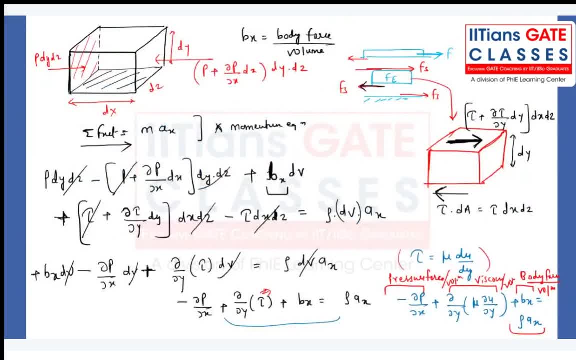 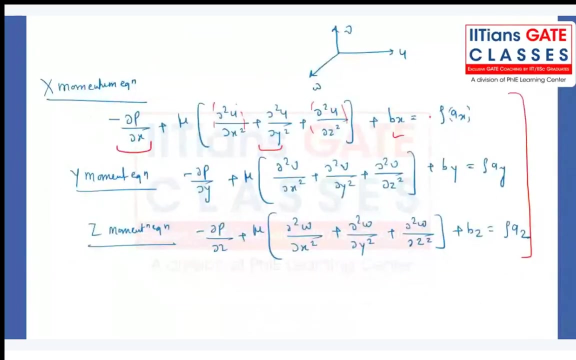 one, and that is only applicable for the newtonian fluids, not for the non-newtonian fluids. now all of you have noted down, can i move to the next one? done so, note on this equation very easily, quickly. now we will discuss each and every separate cases of inviscid flow and for the you know. 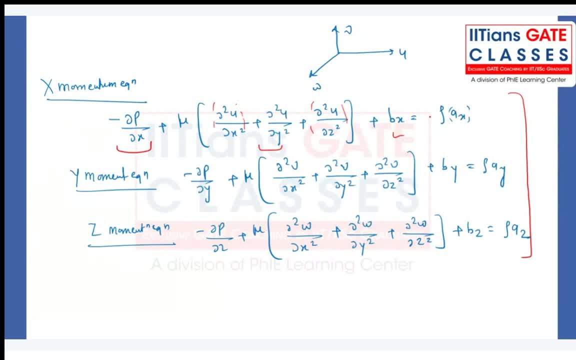 for a hydrostatic when the fluid is at the rest conditions, then also we will discuss these things on the next class done, is it over? see dou p by dou y. what is the unit? newton per meter square per meter. So Newton per meter cube. So that is the force, pressure, force per unit volume. And 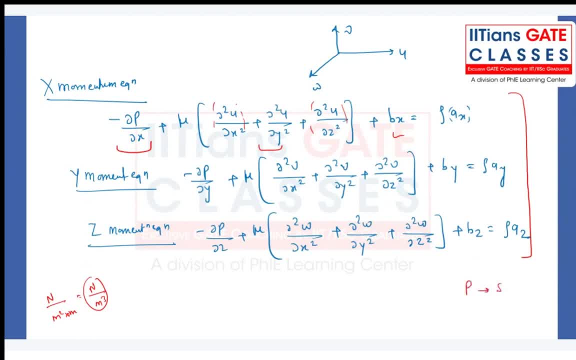 remember my dear friend, P is a scalar quantity. But what about dou P by dou x? Is scalar quantity or vector quantity? What is the dou P by dou x Or dou P by dou y Or dou P by dou z Is? 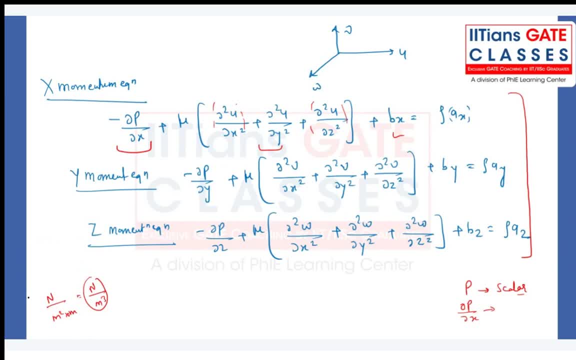 scalar quantity or vector quantity, Because whenever you take the gradient of any scalar quantity you will be getting the vector right from the mathematics. So definitely pressure is a scalar quantity. that is not give you anything about the directions. but dou P by dou x, How the pressure is there, You know in a diverging section when you 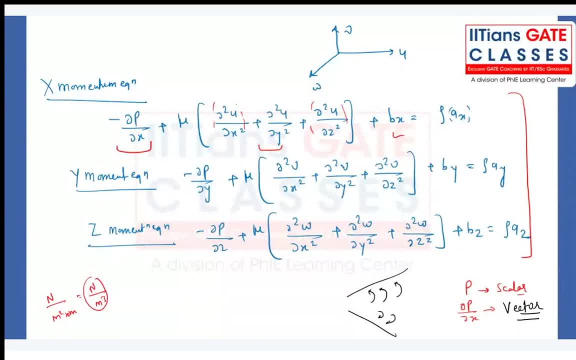 see that there is a ed formations and flow suppressions from a certain particular edges of the diffuser. So what you are observing, actually, that is giving you the dou P by dou x as what This will give you the dou P by dou x greater than 0, right, So that dou P by dou x is. 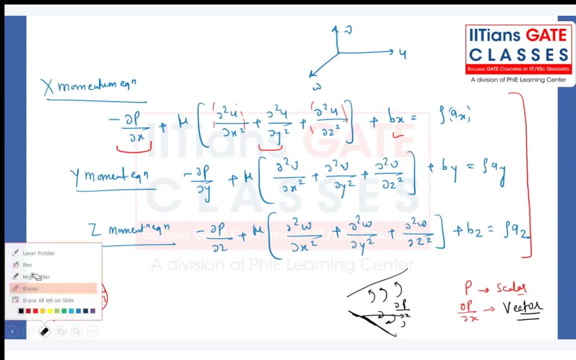 basically what Greater than 0 means what? What is going to be happening When this is going to be there, then what we can say? Adverse pressure gradient correct, So actually dou P by dou x. So we can say that you are able to identify the directions where the flow is happening. 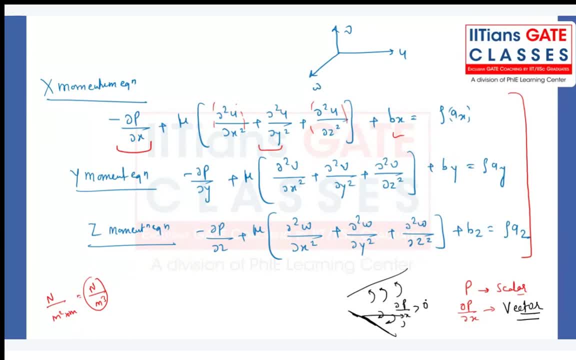 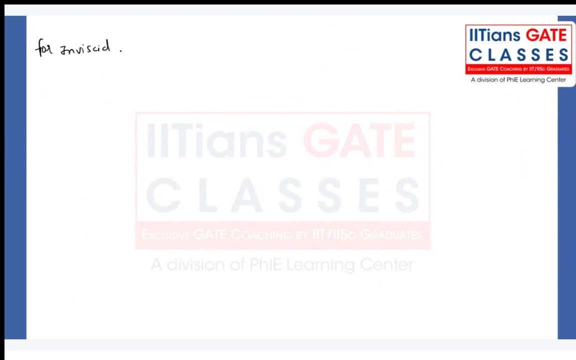 So that is the vector quantity. Now, for an inviscid flow, viscous force will be zero. Viscous force per unit volume: that is also going to be zero. So which term will be zero? X momentum equation. 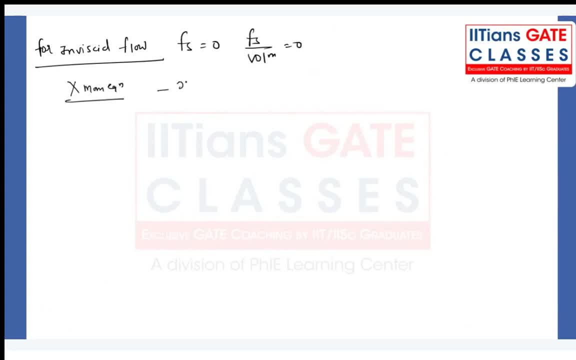 Minus dou p by dou x plus 0 plus b x. rho into a x Y momentum equation, my dear friend, what you will be writing minus dou p by dou y plus 0 plus b y. rho into a y Z momentum equation, my dear friend, what you can write minus dou p by dou z plus 0 plus. 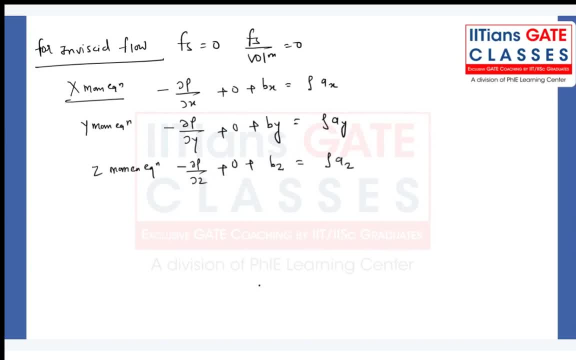 b z rho into a z. This is nothing but Euler equation. Make a note of it. Suppose only gravity force is present, Suppose gravity is present as a only body force, Gravity only presents As body force, then what we can write b x will be 0, b z will be 0, and what we can write b. 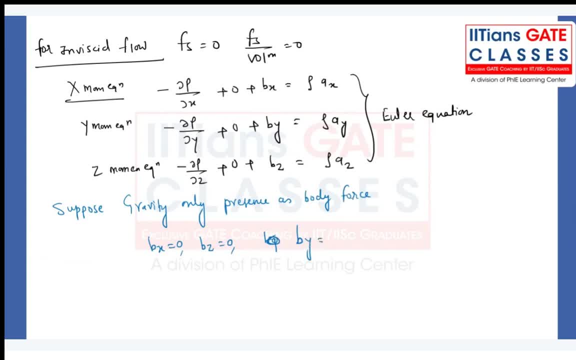 y, the body force in the y directions will be minus mg divided by volume. so that is equal to minus of rho g, because see, actually standard coordinates is what x, y, z, but gravity will be acting in the negative y directions. that's why minus rho g. 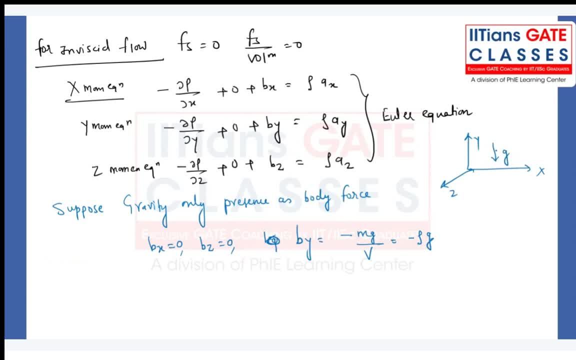 According to our standard Cartesian system rotations. you know, no, no, no, we have not started fluid kinematics I am discuss, I have discussed only little bit about the discussion on the some rigid body rotations and those things. So that is it. Is it done for all? can I move to the next page? 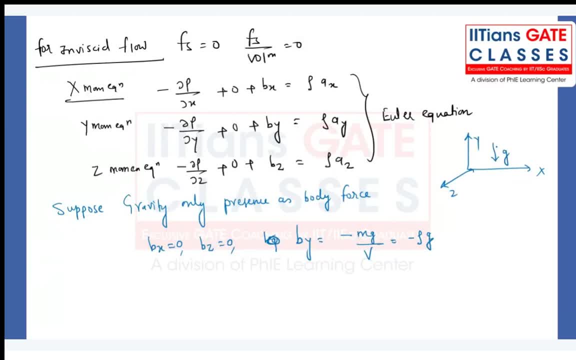 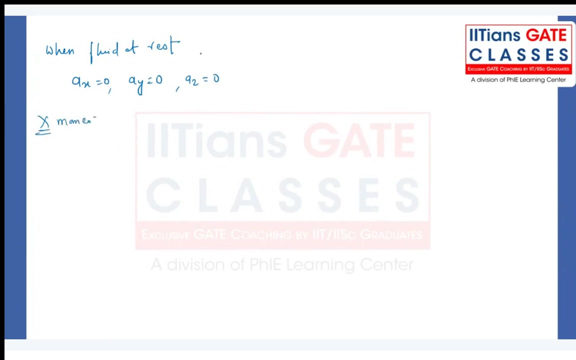 Now what here we are discussing? when the fluid is under rest condition, when the fluid is at the rest, acceleration will be zero, either in y, z or x. What about x momentum equation? Yeah, and fluid at the rest. so automatically shear force by default: zero per minute volume. 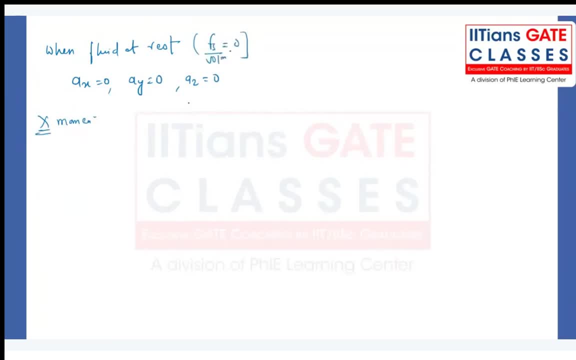 or absolute shear force, that is also zero. So minus dou p by dou x will be zero. y momentum equation will be: minus dou p by dou y minus rho g, that is equal to zero. C minus dou p by dou y plus b? y, that is we are writing as zero, but b? y is what? 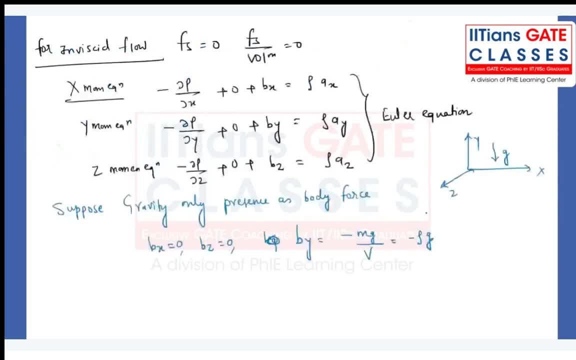 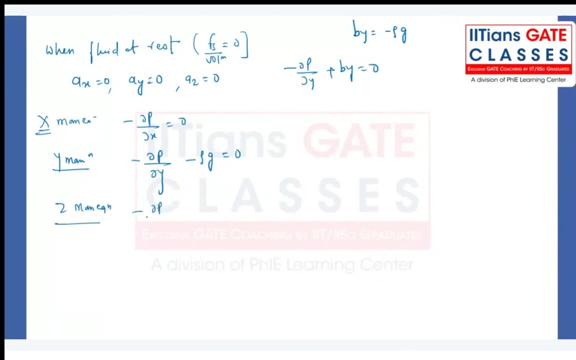 Minus rho g. just now we have seen that. And what about z momentum equation? That is zero. So from here what we can conclude? so pressure is not the function of x, pressure is not the function of z. that means pressure is only the function of y. 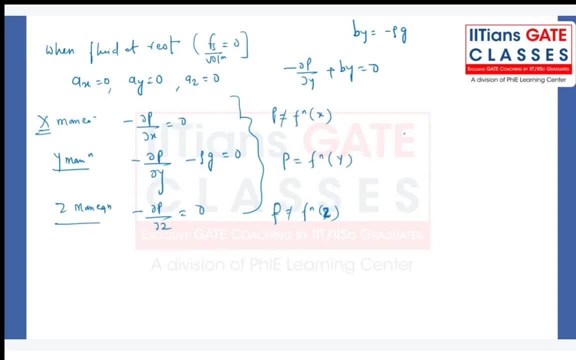 So in a horizontal, So in a horizontal fluid system there is a fluid suppose and both are at the same level, so in the x direction- at point number 1 and 2, the pressure will be same. If the fluid is continuous, then pressure will be same. that is the consequences of. 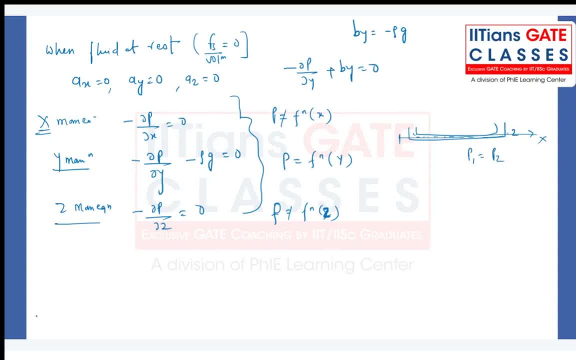 dou p by dou x, equal to zero, And that is the basic principle of. that is only the basic, fundamental thing we are applying in the manometer Right. The fluid, Yes, Yes, Yes, Yes, Yes- Which are continuous at the same horizontal level, directly, we equate the pressure. 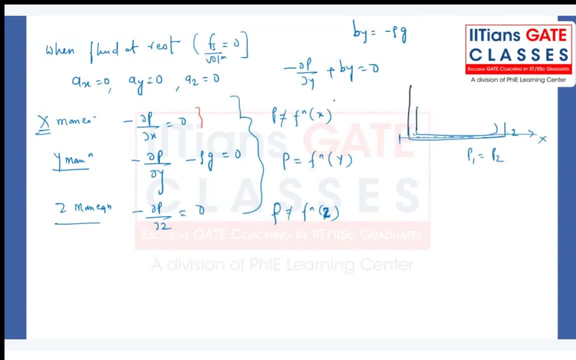 Right, So we are connecting this to one limb, this connected to other limb. suppose tank, we want to measure the pressure. we place it certain liquid called the manometer fluid, and whatever the height that is being raised will give me directly pressure value. 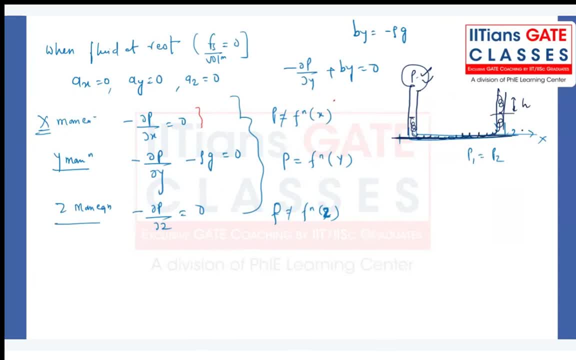 Because at this point we are just equating the pressure Now. so what is the total value you are getting Now? now, my dear friend, when the pressure is not the function of y- and sorry- x and z, can we write dou p by dou y? that can be written as dp by dy. 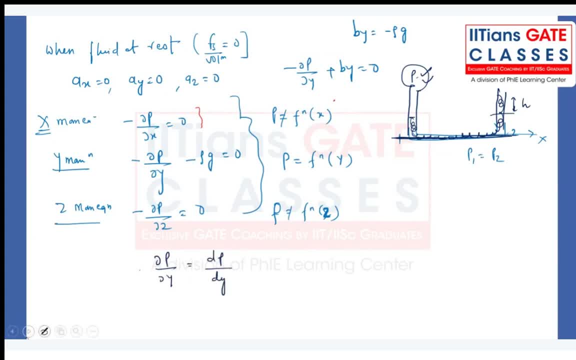 Tell me The partial differentiation. we can write it as total differentiation, Right? There is no harm in that, Right? And if we can write like that, so I can just write this also: dp by dy minus of rho g, And that is what you are arrived to. hydrostatic law. 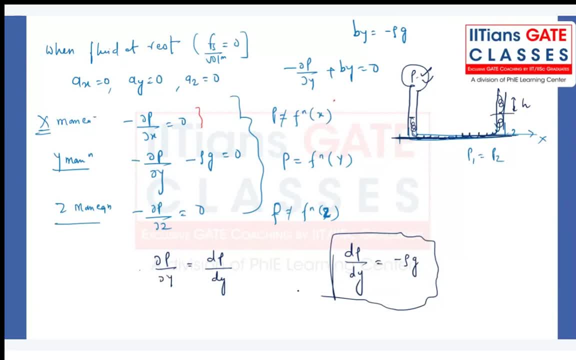 So what is the hydrostatic law? This law, it states that the rate of, yeah, the rate of increase of pressure in a vertical downward direction, In a vertical downward direction, at a point in a static fluid, of an incompressible fluid. 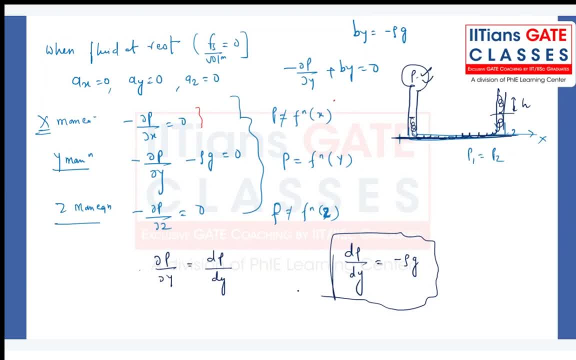 of maybe compressible fluid. it need not to be compressible and incompressible. we will see that That must be equal to a specific weight of the fluid. Because what is that specific weight? Weight per unit volume. That is the logic. 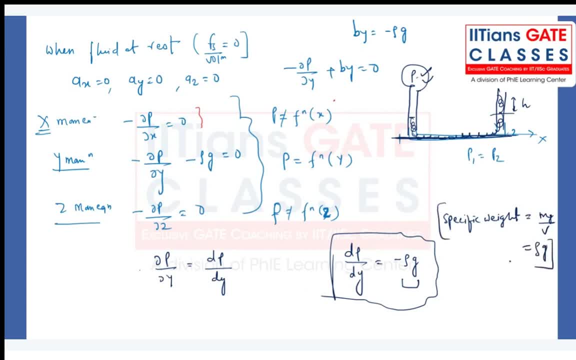 Yeah, Yeah, Yeah, Yeah. Okay. Now, once it is done, let me know This particular slide. So, even though basic understanding we can derive from the Navier Stokes equations- Right, Please note down Navier Stokes equation. 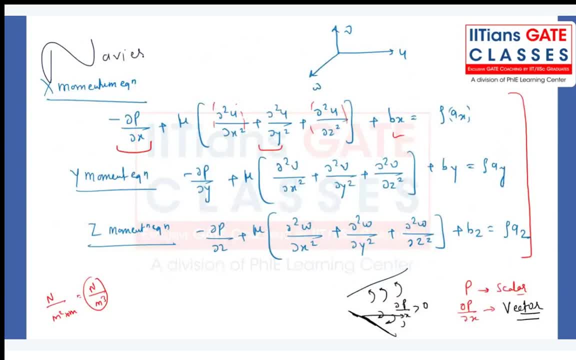 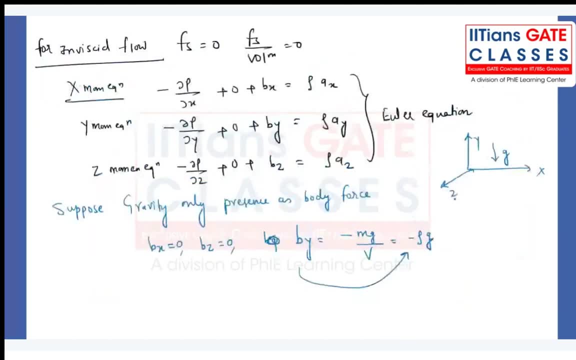 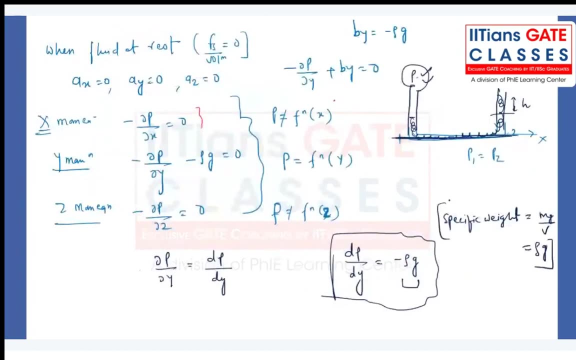 These are the Navier Stokes equation. Don't think that Navier Stokes is of something like a rocket science of things and we are only discussing in the fluid dynamics. See, we have arrived to the fluid dynamics, arrived to the conclusion of fluid statics law with the help of navier stokes. so when? 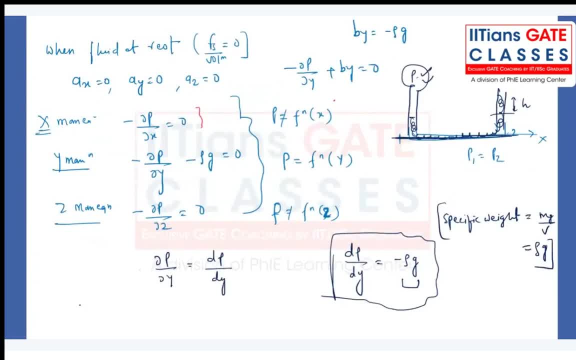 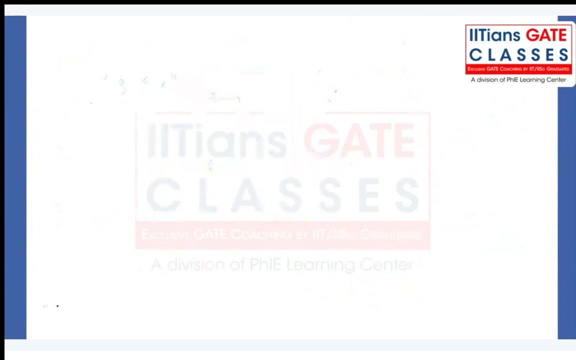 you play with the navier stokes equation. you do not to worry so much about the fluid mechanics, or maybe i would say, up to some extent, aerodynamics. you know done all of you have noted down. note down, guys. yes, correct, so note down hydrostatic law. 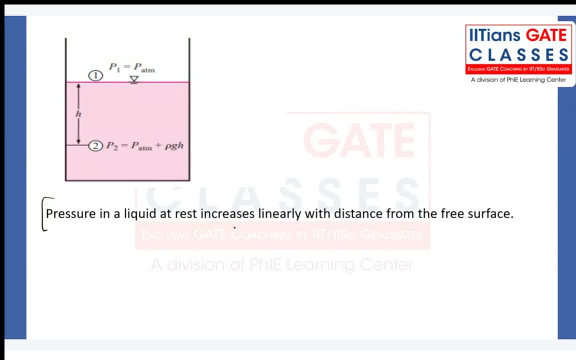 pressure in a liquid at the rest increases linearly with the distance from the free surface. that we will arrive to the conclusion of this one, but before that you note down hydrostatic law. this law, it states that the rate of increase of pressure, the rate of increase of pressure in a vertical downward directions, 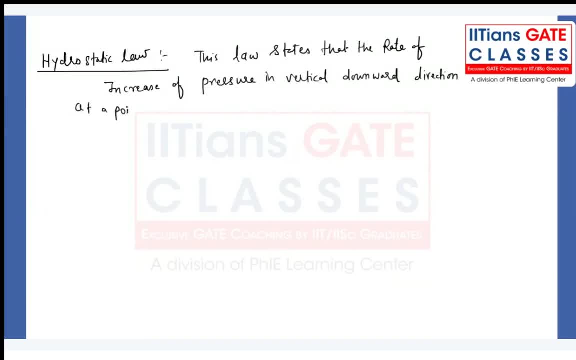 at a point in a static fluid must be equal to local specific weight of the fluid. That means dp by dh must be directly proportional to rho d. So when you know the RTT equation you know Reynolds transpose theorem. even most complicated problem you can solve by that equation. 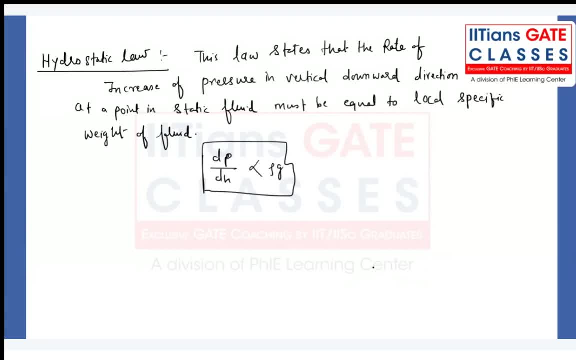 But why students face difficulty in solving the problem by RTT. you know the complexity involved in that equations, whether we have to consider reference frame that is stationary or that is moving right. That is actually the difficulties in that. And one more assumption is there. 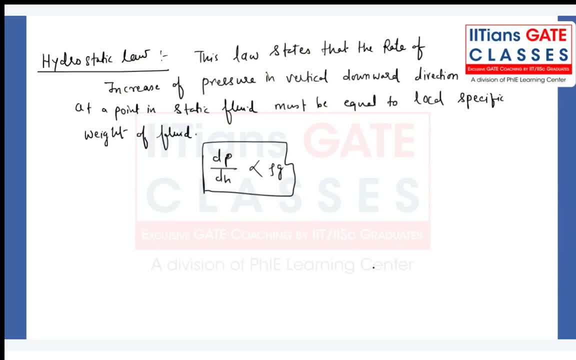 In that Navier-Stokes or RTT derivations. what is that? regarding frame of references, Tell me guys, That should be inertial frame of reference, right? That should not be non-inertial frame of reference, That should be inertial frame of references. 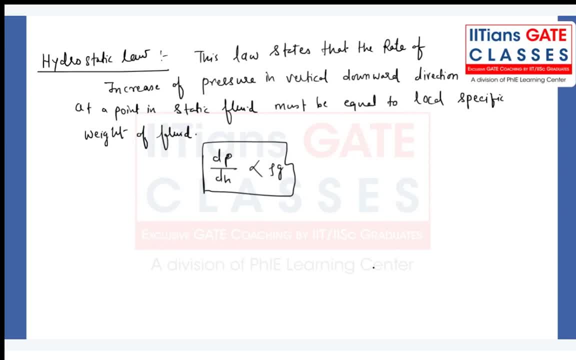 That means you are as an observer. yeah, you are as an observer. Yeah, they will be directly proportional. you know, or they will be directly what we can say? Yeah, Sorry, Here I have written. Yeah, you can write dp by dh, something like this: 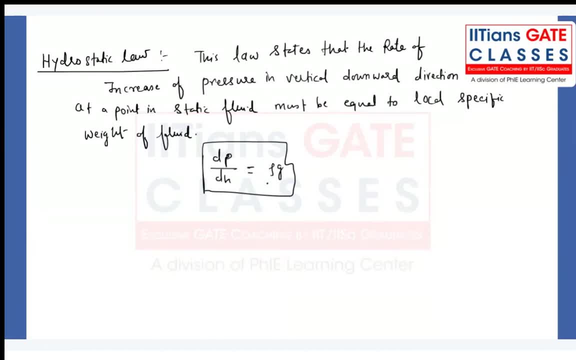 Now, regarding sign, whether it is a minus rho g or plus rho g, that will be clear when we discuss about further. you know further if you simplify dou, p by dou y, you know. or dp by dy, Okay, This we have written is equal to minus of rho g. 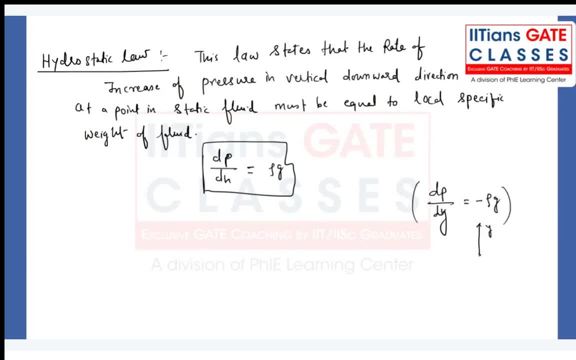 That is according to sign convention. this one Plus you can write: when you write the y direction like this, You are taking downward direction of y as positive. then you will be getting the equation dou p by dou h or dp by dh as rho g. 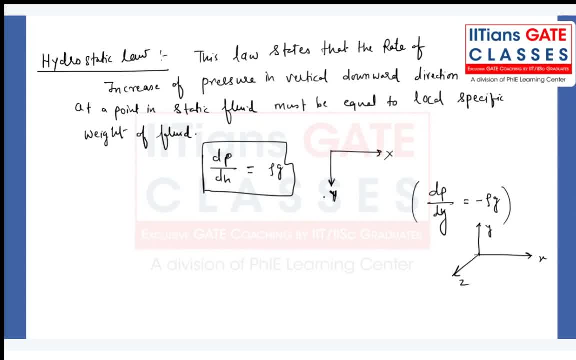 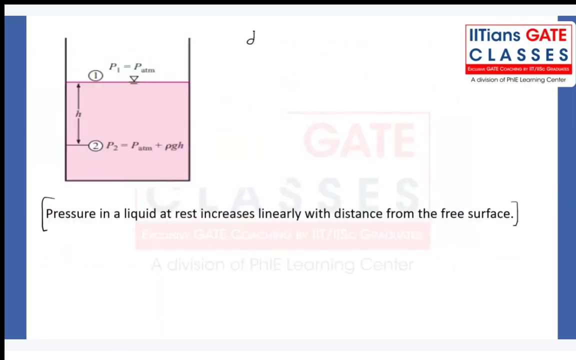 Anyway, any sign convention you follow, you will be getting pressure equal to rho g, h. Okay, Let me prove that. Now, once it is done, let me know. See guys understand Here when you try to observe what is the equation. we have dp by dy minus of rho g. 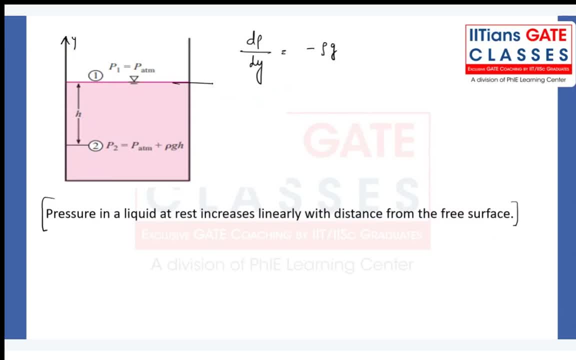 Yes, This is my y direction, This is my x direction. Or maybe I can write over here, At the bottom one: I can write here something like this: And this is my point number one and this is my point number two. for example: 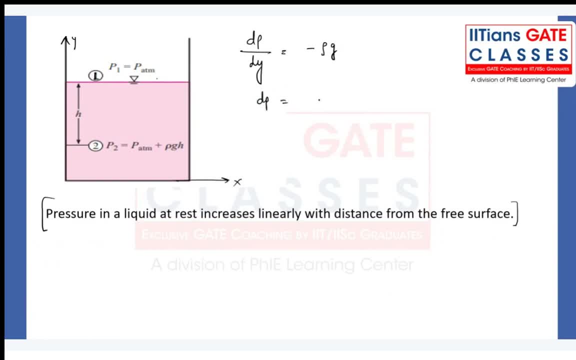 So can I write dp equal to minus rho g into dy And can I do the integration from one to two? What should be my limit? Suppose this I am taking as a reference that is a zero value of y right And I am moving in the downward directions. 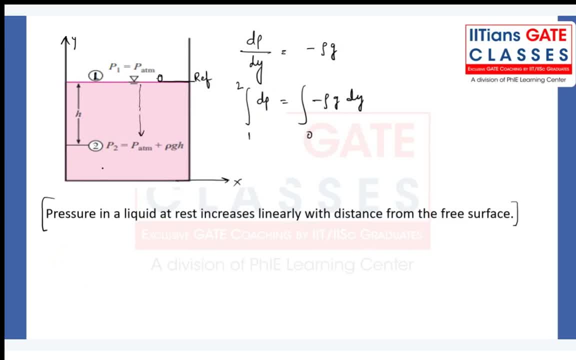 I am moving in the downward direction, towards the point two. Actually, I am moving towards the downward And my sign convention is that if I move upward, then I will take positive h, But if I move downward I will take minus h. 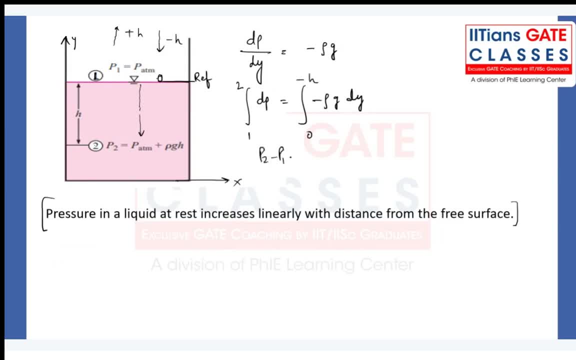 Right. So what we can write: P2 minus P1, that can be written as minus rho g. integration dy: 0 to minus h. Remember. Remember When only you can take the rho outside the integration, When it is incompressible fluid. 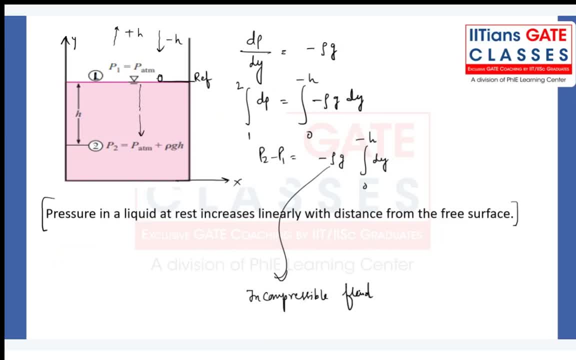 Or we can just take when the density is not varying with respect to height, Right. So what we can write, Minus rho g, minus h, you will be getting P2 minus P1, rho g, h. For example, if P1 is P atrium, then P2 can be written as rho g. 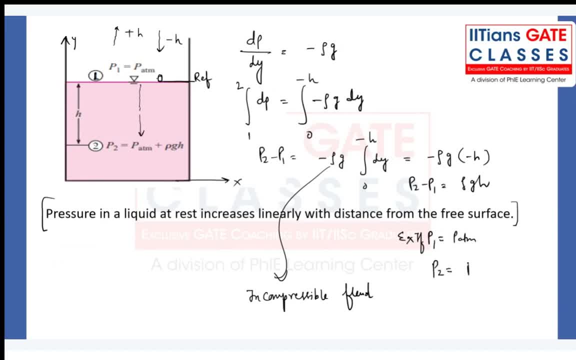 Right, Then P2 can be written as what P, atrium plus rho, g, h, And that is how you can see that pressure will vary linearly with respect to height Right From the free surface. Make a note of it, Perfect. 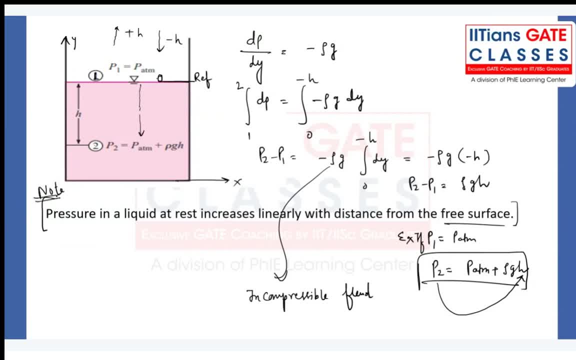 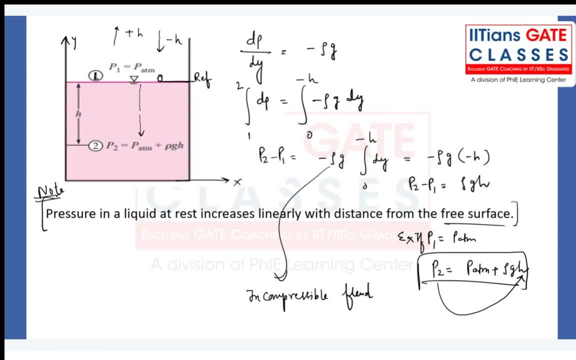 Thank you, But generally we apply RDT for converting. it is control, Whatever that you know, system approach to control, volume approach. Because whatever the Newton's Law is applicable, that is for the solid body, for a single particles, And if we want to convert those law for the fluid elements, 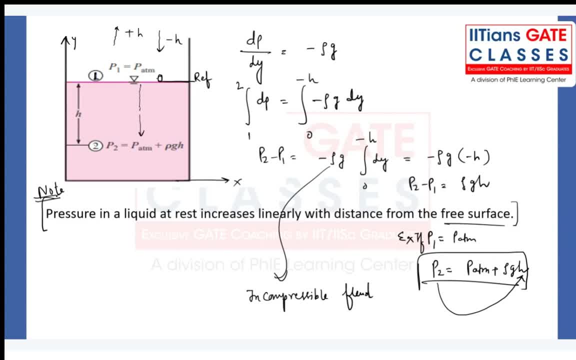 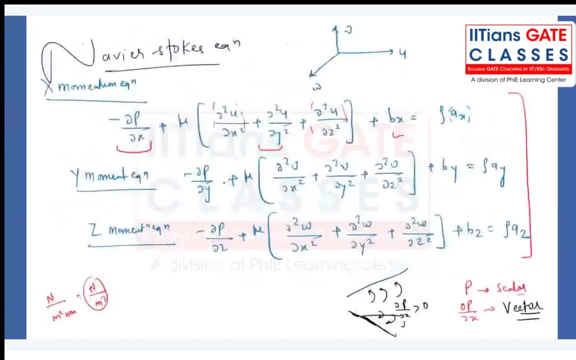 Because see, whatever the Navy stokes equation we have derived, why we have written by using the new, this one and I. but what is the condition for that? Newton's second law, that definitely has to be applied to some particles, single particles, but we are able to apply for a control volume, just. 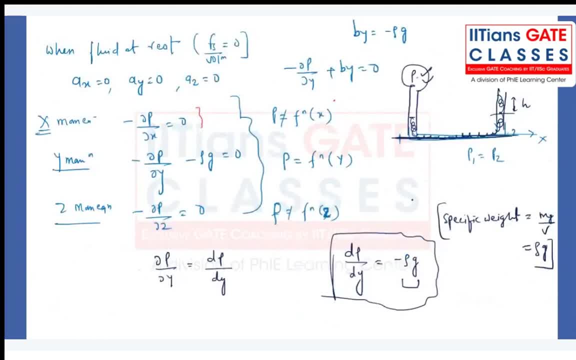 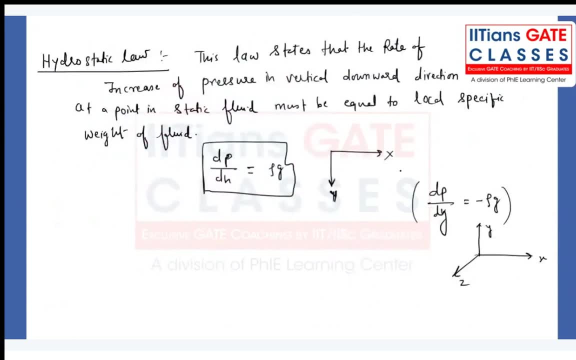 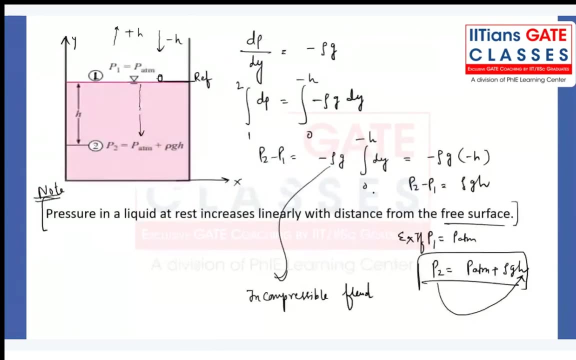 because we should be thankful to RTT that converts the, actually the necessity of basically what system to control volume right. getting my point, even you can derive the navel stokes from a RTT equation. also, that is what I told you. the conditions right. that should not be inertial, that. 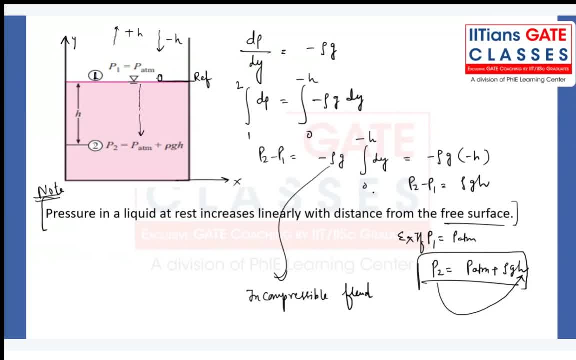 should be inertial frame of a difference. getting my point, what is the meaning of inertial frame of reference? That means acceleration should be zero, right, Is it done? Shall we see the? actually the how it is varying linearly. Let's focus on that, you know. 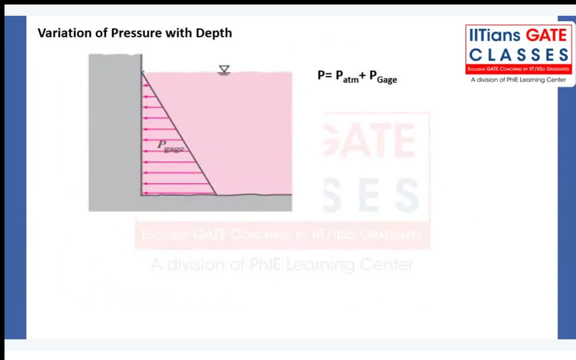 As you can see, by different, The pressure is varying from here. Actually, this should be: have the variations, something like this: you know, At this point 2, at this point 1, pressure should be, at this point should be: rho g, h. 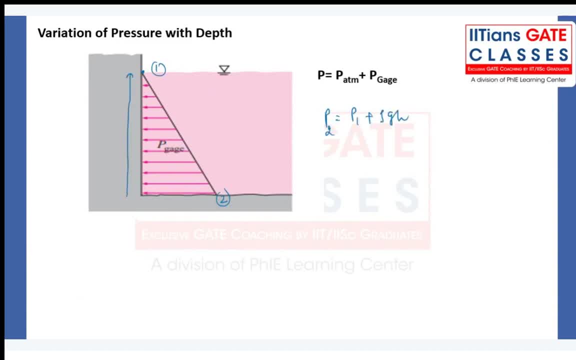 or a height h. But if I take pressure 1, equal to zero, what we can write directly? P2 will give me the values of P gauge, right, And that is what we have. They are varying linearly. Make a note of it. 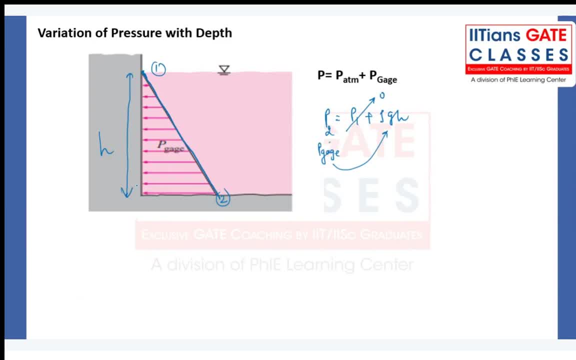 See, these are the very, very small thing, guys. Maybe directly somebody will be there who will be telling you pressure equal to rho g h. You please note down directly, without any derivations. But you only have seen with your own eyes that how difficult it is there even to arrive a very simple conclusion. 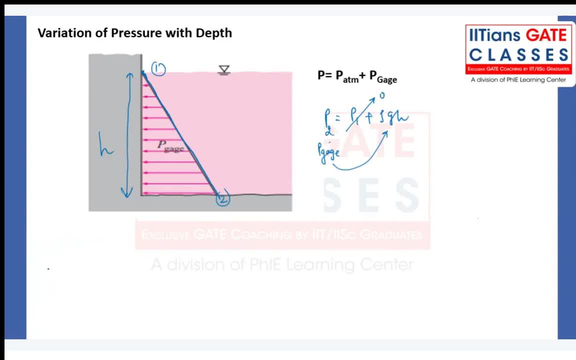 We should know fundamentally each and everything, So that any difficulty in a examinations you know in a particularly examination, Hello, hello, I'm audible. I'm audible, Yes, In examination. suppose examiner has given you something like this. You should not get panic. 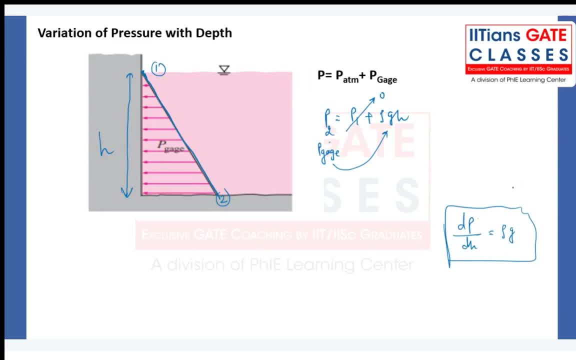 They will mention the coordinate system also. Getting my point: If they will not mention, we have to assume over the standard sign conventions, Or in a paper, Or they will directly mention. you know So, whenever you see minus rho g is not there, sir, then how we can proceed. 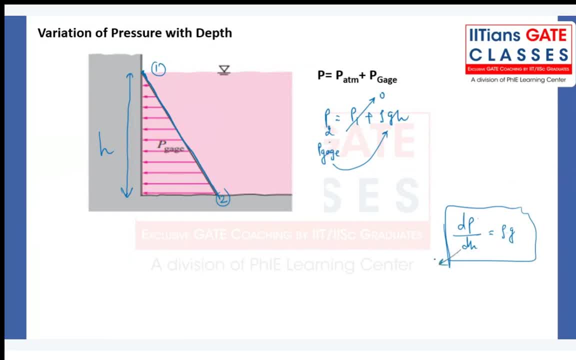 No need to panic, Because with this also you will be getting the same thing. How Let's see For this one. what is the sign conventions? This is my sign convention. That means if I move in the negative y directions, I will be writing plus h. 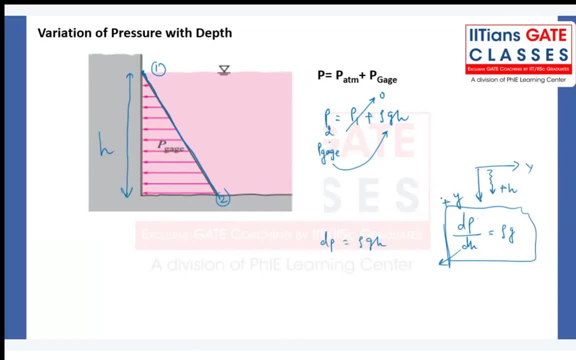 Right, I am considering this as positive y, this as negative y. So point 2,, point number 1,: 0 to h. So I will be getting what P1 minus P2.. Oh sorry, 1 to 2, right. 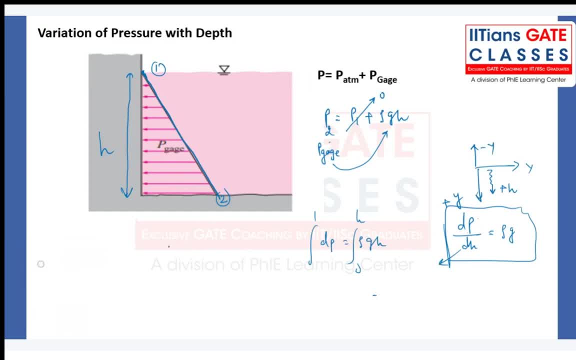 Here I need to write 1 to 2.. So P2 minus P1.. Once again you will be getting what Rho gh. It's only the matter of sign convention for a coordinate system. Getting my point, all of you? 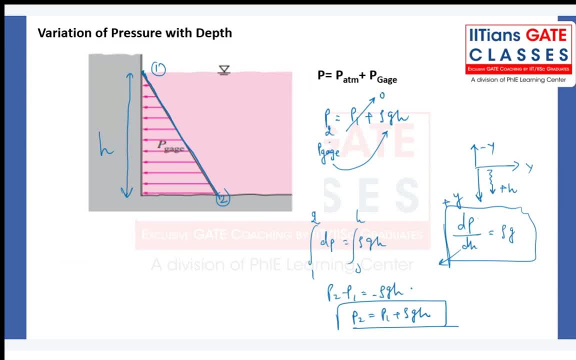 So actually, I am telling you all the conclusions. I am telling you all the conclusions of different different textbooks. When you follow any other textbook they try to mention, like this: Sometimes they used to follow different sign conventions, But our standard sign convention, which we follow from our childhood days, that this is y positive y, this is positive x, this is positive z. 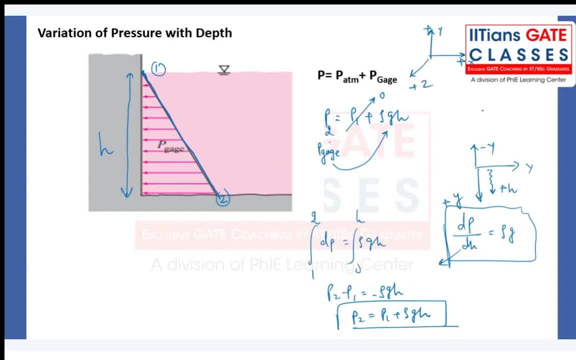 And what is the standard for the rotation angle? Anti-clockwise that is positive, Clockwise that is negative. That is our standard one. You know I am not saying that in examination Anti-clockwise always will be positive. They will mention. 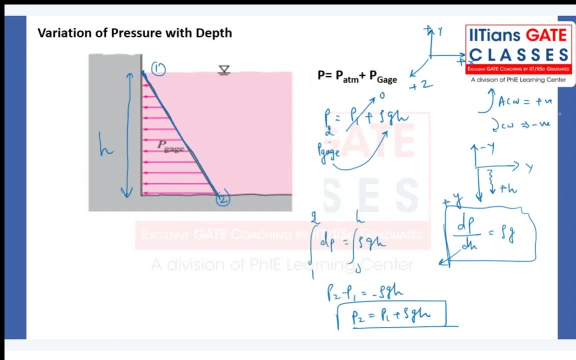 They can mention negative, But I am telling you what you actually, guys have followed from, basically what Your 10th standard or 11th standard. That is what we are considering over here Now. is it done for all? All of you have drawn this one. 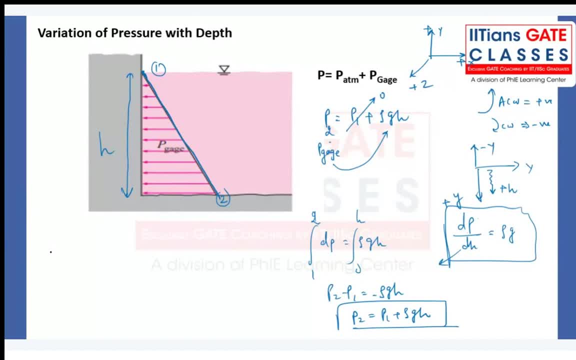 Can I move to the next segment? But do we have only a linear variation of pressure with the height? We don't have any other variations like exponential or any other variations. Tell me this: Do we have only the linear variations? As you can see, there is a linear variations. 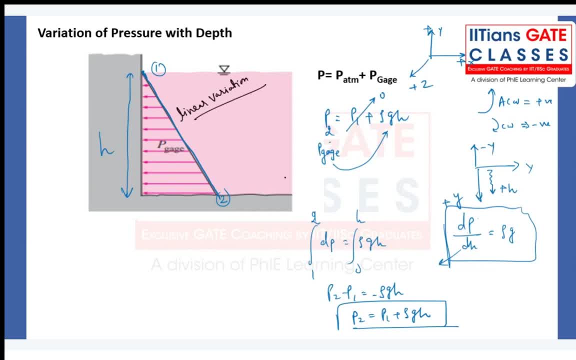 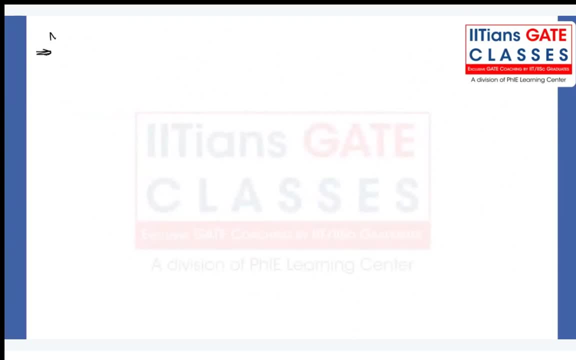 Don't we have any other variations? Yes, we have the variations. Let's focus on that. Now note down important note: ideal gas in isothermal conditions. Ideal gas in isothermal conditions- Now guys, try understanding. So, for example, you have the suppose earth's surface as you march. if you keep just going higher the altitude in isothermal layer, you know you might be having the variation of pressure. 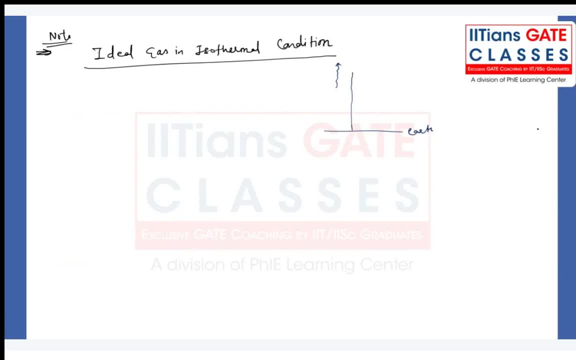 That is the ideal gas in isothermal conditions. Definitely variation in the density, but we are assuming temperature to be constant, for example. right, So, my dear friend, what we can write at the earth's surface, we have the condition like P naught P naught at, let's suppose, y equal to zero. 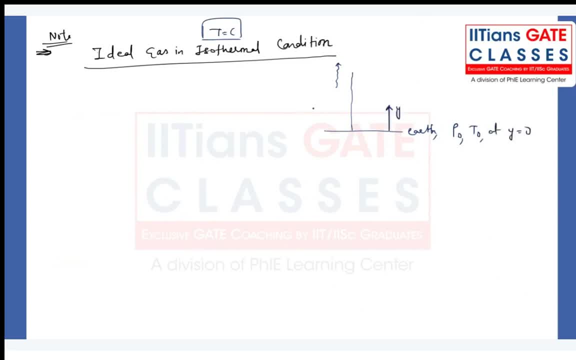 We are moving like this And we are very much interested to calculate what is going to be happening about the pressure, about the density at y equal to small h. Okay, So for that definitely we have to apply the hydrostatic law, that is, dp by dy minus of rho g. 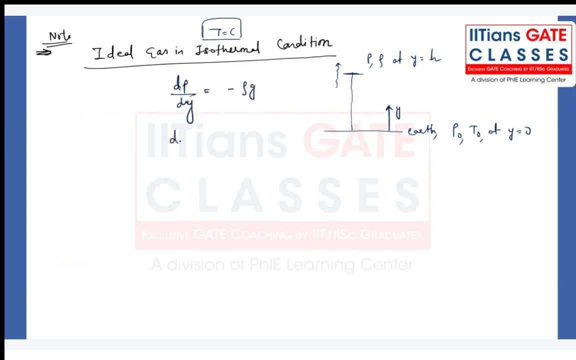 So now dp can be written as minus rho g from integration, if we do. but here you cannot take density g as constant density rho directly. you cannot take outside of the integrations, because right now from ideal gas law P is equal to what? 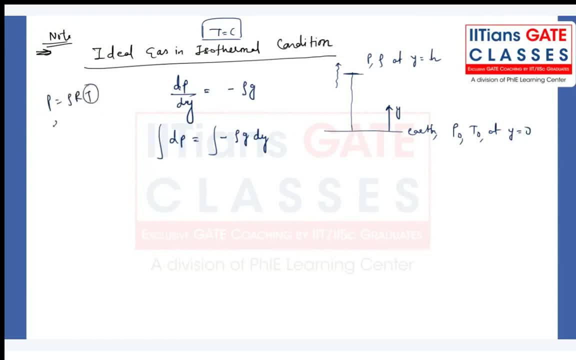 Rho rd. Okay, So rho will be constant. So rho will be what? Something constant divided by P, Sorry. So P will be what Directly proportional to rho. So further, what we can write rho. 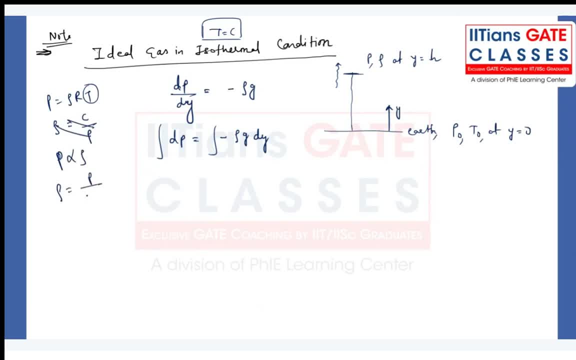 Rho can be written as P divided by what RT Getting my point. So if you just write this one into that equations and integration we are doing from P naught to P And y is varying from 0 to positive h. 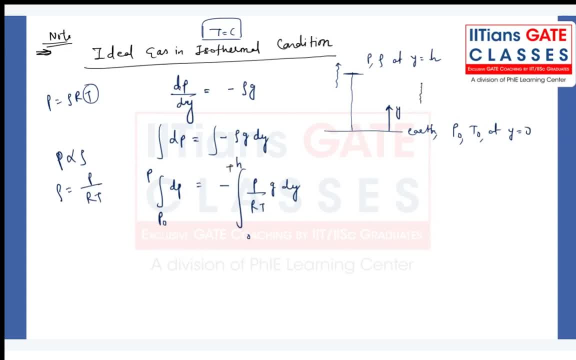 Why positive h? Because we are moving like this: According to standard sign conventions that is a positive value. So when you write P minus- sorry, here we have to perform dp by P, P naught to P minus g by RT. that is constant dy 0 to h. 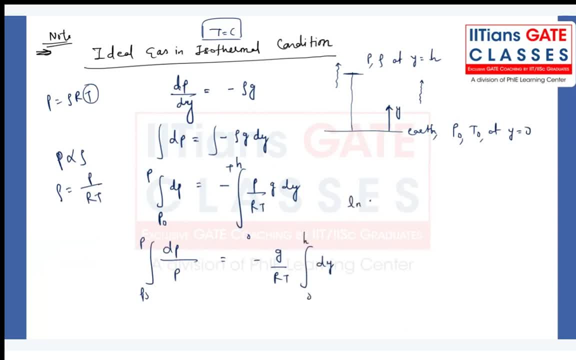 Okay, So when you just write log of P, that is from P naught to P, or maybe you can write P dash, rho dash, P dash, P dash. Now, here you can write minus g divided by RT into h. 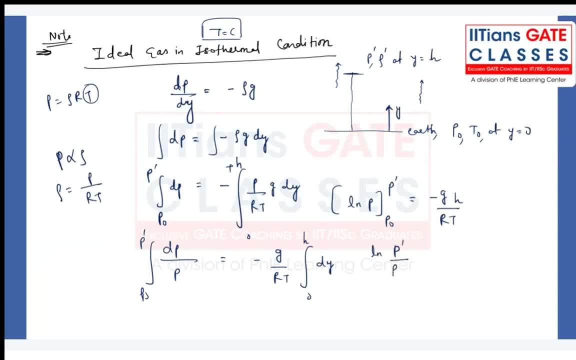 So ln of P dash divided by P naught, that is equal to minus g h divided by RT. So P dash can be written as P naught into exponential of GH divided by RT. So how the pressure is varying with the height exponentially. 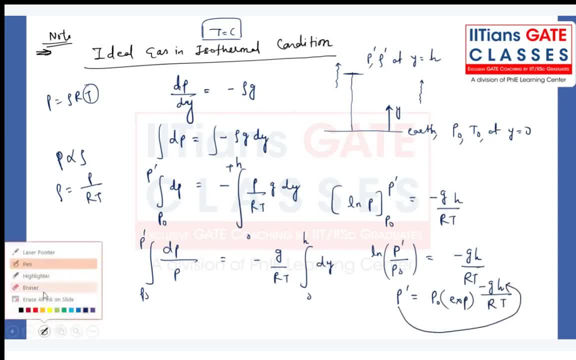 So when you just write the variations, this is varying as exponentially, This is actually varying the value. So this is actually varying the value. Okay, not linear manner, It is varying exponentially. Is that clear for all of you? Tell me, guys. 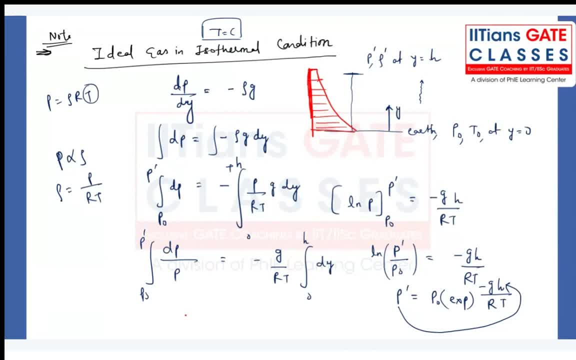 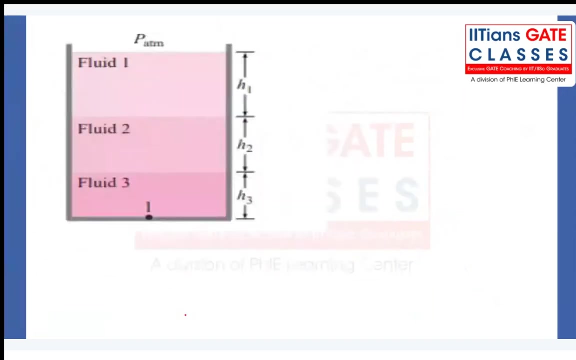 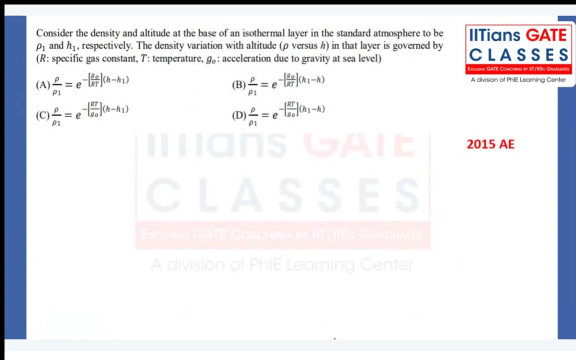 Explain again. If it is done, let me know Done Now, when you see this particular question. you know. consider the density and altitude at the base of the isothermal layer as rho1H1.. The density variation in the layer is governed. 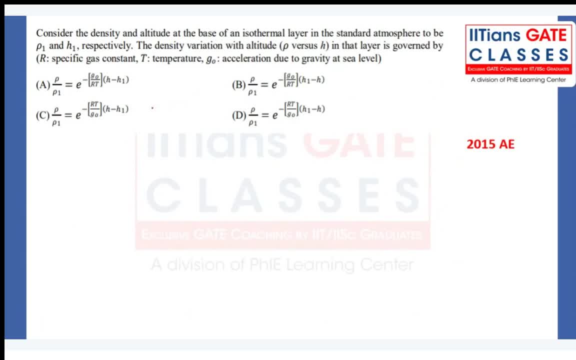 by which law Right? So what will be the answer for this question? That is a pretty straightforward, Because we have seen the pressure variation, and pressure will be directly proportional to density, So in a similar way, the density will also vary. Please try that. 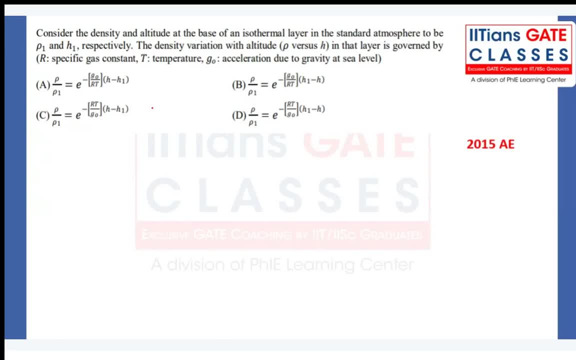 Now check it out once again Very carefully. you please observe that. So, instead of: basically, we have just now seen that P dash by P naught, P naught is equal to exponential of or e to the power of, e, to the power of minus g, y. 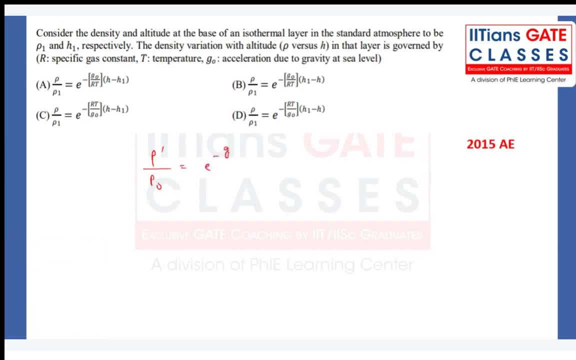 by r t. this is what we have seen, that. but here they are mentioning that, uh, particularly layer height from h1 to something h. they are asking somewhere the reference is zero. right, we have taken the reference from zero. so if you just do the integration minus dp by p, from what we can write, that is: 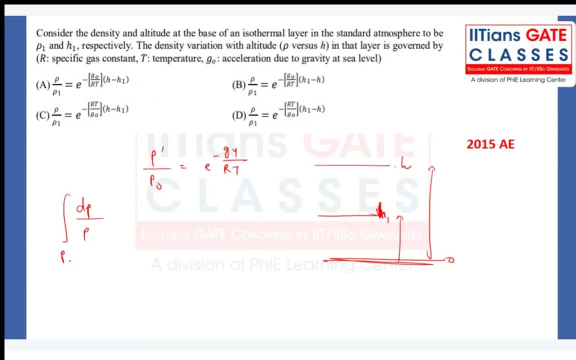 what we can write p1 to p, that is equal to minus g by r, t into dy. from what we can write h1 to h. so ln of p divided by p1 minus g, by r t, h, minus of H1, Z0 they have mentioned in the problem, So let me take Z0 only. So further, what? 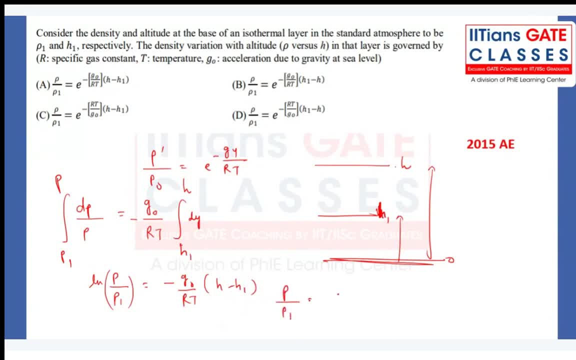 we can write my definite P by P1 minus Z0, by, sorry, exponential of Z0 divided by RT. This is the pressure variation and we know that pressure is directly proportional to density. So that will be rho by rho 1, exponential of. because P you can write rho, RT and this: 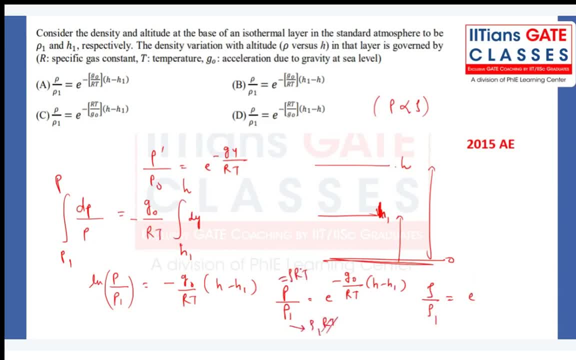 you can write rho 1 into RT. This will cancel out in isothermal layer they have mentioned. So we can have minus Z0 divided by RT, H, minus of H1.. So if you do not do that derivation, definitely you will be having challenging in solving. 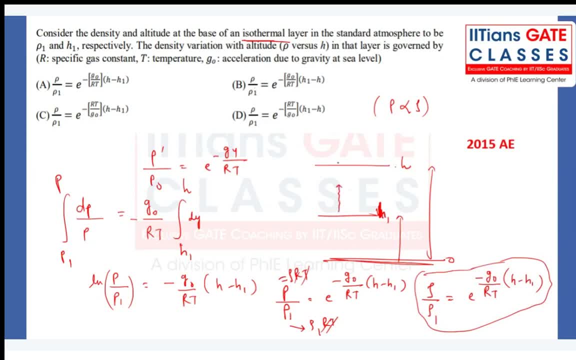 this, even though simple problem, you know whether I should be taken. So from H1 to H, or H to H1, or H1 to minus H, something like this. that is why we, if, whenever we learn any formula by the derivation, definitely it is having some advantage, and you need to. 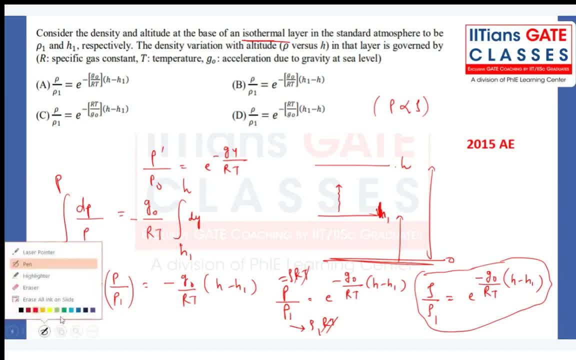 be little bit patience also, because nobody have that much of patience in understanding the derivations, then formula, then solving the numericals, They directly jump to second step, that is, learning the formulas. Apply this, So apply to the question, get the answer. that is it. 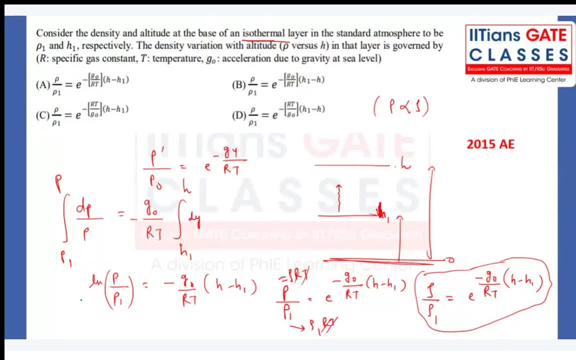 Especially when you are sitting at the examination hall. our chances of committing the mistake is very high. If you are sitting at the room- solving that there is no big deal in that. The whole problem Will be arising when you just go, basically going for the deciding day. that is actual. 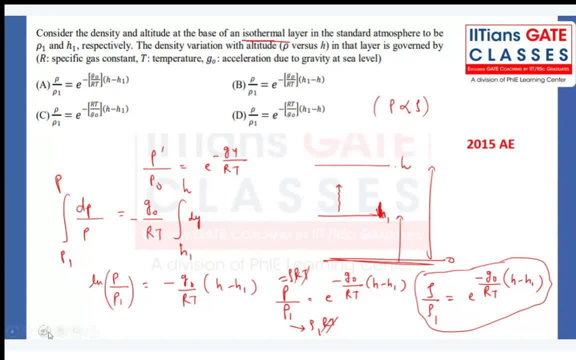 day of the GATE exam, How well you are able to perform during those three hours movie. that is the only the matter of concern. that is only matters. actually nothing matters before that day what you are doing for the past eight months or nine months, that will be reflected directly in the results. 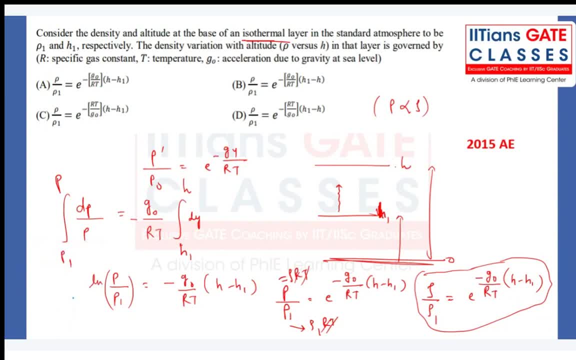 So that is. you know, they used to say compound interest as the seventh wonder of the you know maybe eight wonders. when you just do any investment and when you do the compound interest of that, definitely the return on investment will be very high. But believe me, I don't think that that that would be the correct one. of course that is correct mathematically. when you do the compounding, definitely our rate, or whatever the return on investment will be very, very high. 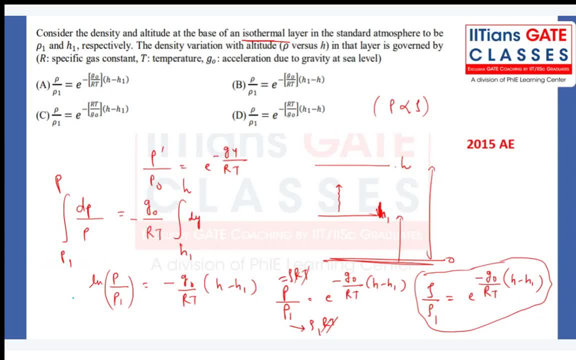 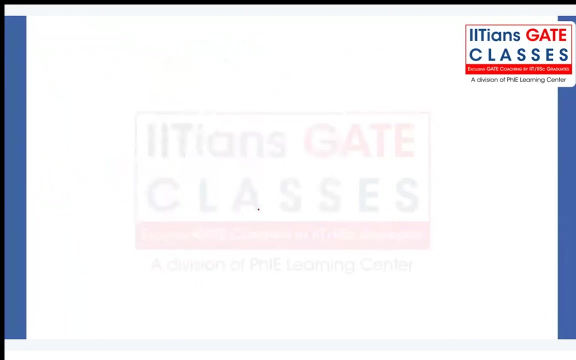 But Actual investment is this great example. when you can play with these three hours, the return is quite high. You cannot believe also. Now is it done, all of you? Can I move to the next topic Now? hydrostatic paradox. let us discuss about that little bit. now. note down the next topic. 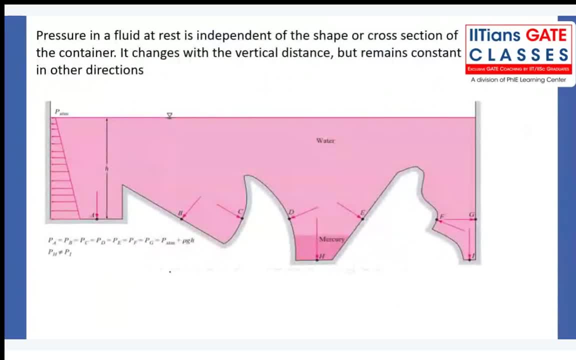 Hydrostatic paradox. all of you can see this one. note down the topic name: hydrostatic paradox. Anyone know this one. The pressure in a fluid which are at the rest condition, which is not moving in a container- it is at the rest condition, is independent of the shape of the container or the cross. 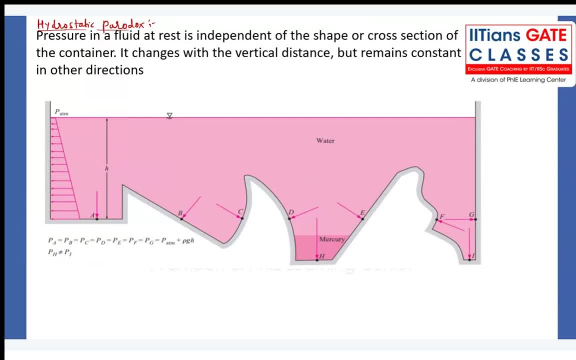 section of the container. It only changes with the vertical distance, but remains constant in other directions. you know, dou p by dou x, equal to zero right. And so now, guys, it only varying in the y directions. it will not vary in the x direction. 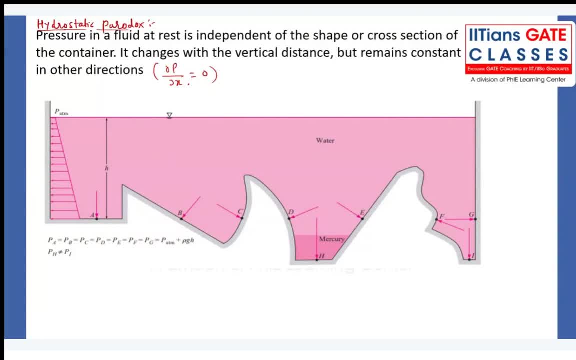 or in the z directions. That means, if you just see here, Pa, Pb, Pc, all are having the same pressure value because height of the liquid is being same, h only, Even though shape of the container: the first one is a rectangular, one second one is quite. 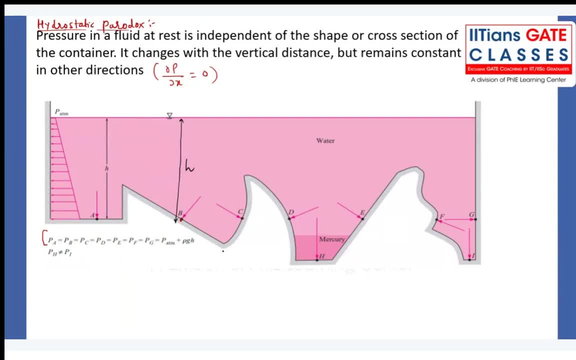 different than the rectangular one. Third one, C point is on the circular track. again D is there on a, particularly what Some other track than E point you have, but here the precaution is, the height should be same and the water molecules or whatever the liquid molecules is there, or whatever the 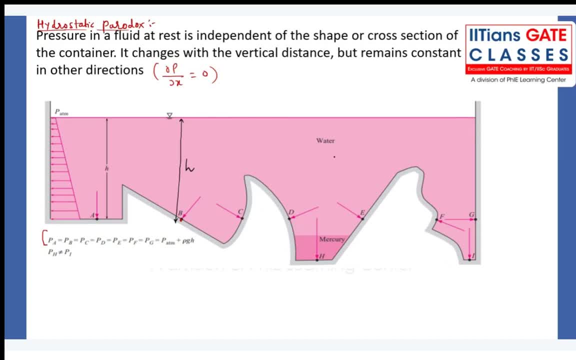 liquid is there. that should be same right, Because pressure value is not only depending on the height, it also depends on rho. The moment you are changing the density, you know, even though same height is there from here to here. So rho of water, g of height plus rho of mercury, g of h minus small h, but still pressure at. 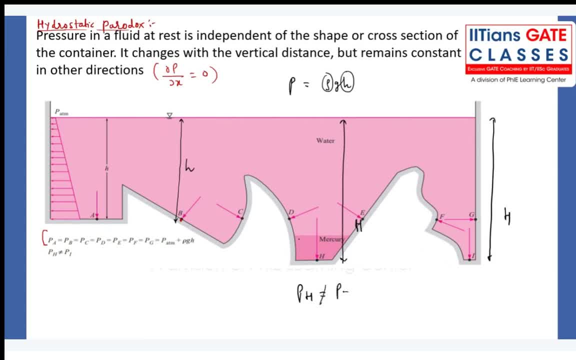 h is equal to what? Not equal to pressure at i. Why? Because pressure value at h point will be rho of water, g of height plus rho of mercury, g of h minus small h. But when you just look at the pressure at i point, what you are observing? rho of water. 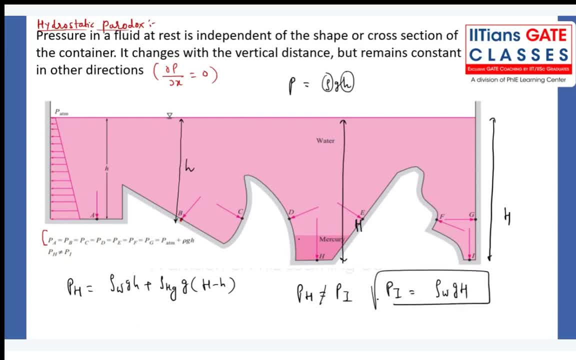 g into capital H, So rho of water, g of height, plus rho of mercury, g of h minus small h. As you can see, they are not equal, Irrespective of the shape of the container. why they are unequal right now? because of: 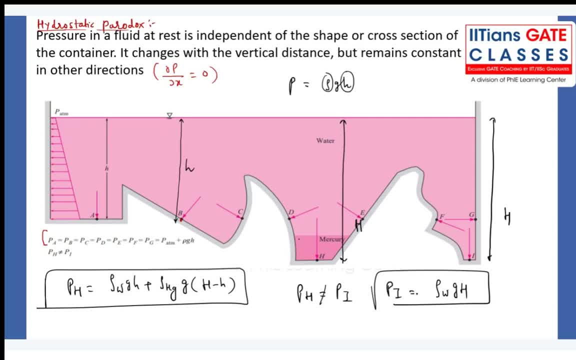 the liquid changes. So pressure value at a particularly horizontal level is equal to the pressure at a particular level. horizontal level in all the horizontal level will be same. that is equal to rho gh. is it done for all which one? which particular portion i should be repeating? 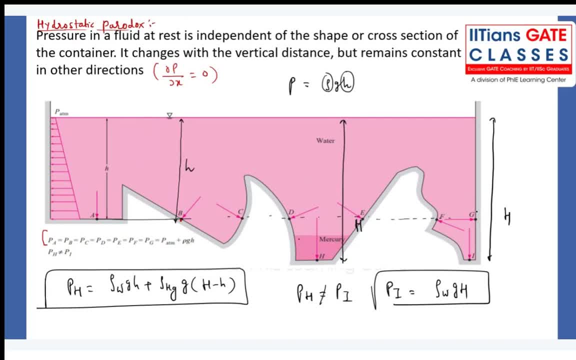 see hydrostatic paradox. it is saying that when you have the liquid that is not moving, when you place in any shape of the container of the same height, same liquid, the pressure value at the bottom of the container will be same, whether container shape is rectangular one, circular container, is spherical container or triangular container, whatever it may be. 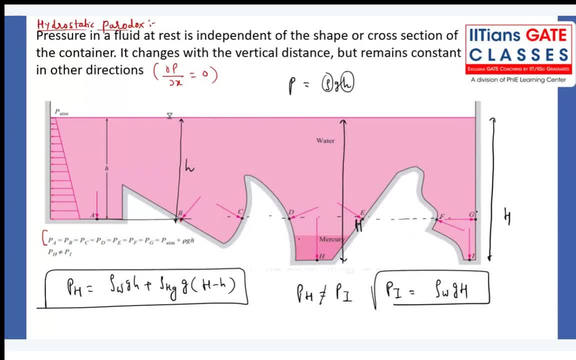 the pressure value at the bottom of that container will remain same until unless you are- not until unless you are- changing the lipids. that means pressure value at h point, as you can see, the total height is remain same for h point and i point, but still the pressure value. 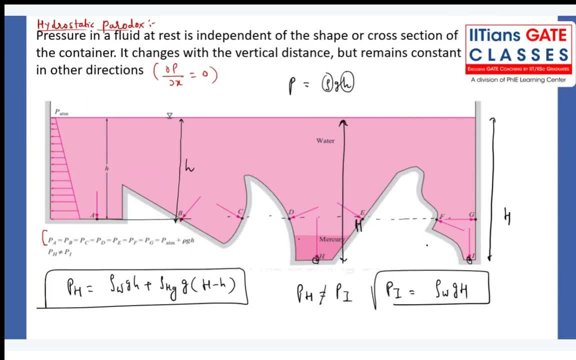 is not same, even though shape of the container is different. why? because here you have the water, up to some height, then you have the mercury, but here, when you see only water, is there right? but apart from these two point, when you consider a, point b, point c, point, 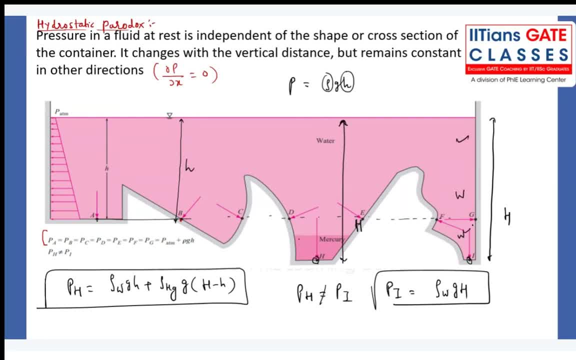 d, point e, point f, point g, point, you have the pressure value exactly equal to p atm plus rho gh. yes or no, guys? can i move to the next one? so you might have heard about the hydraulic jack or hydraulic lift, right? so that is also working on the principle of what? 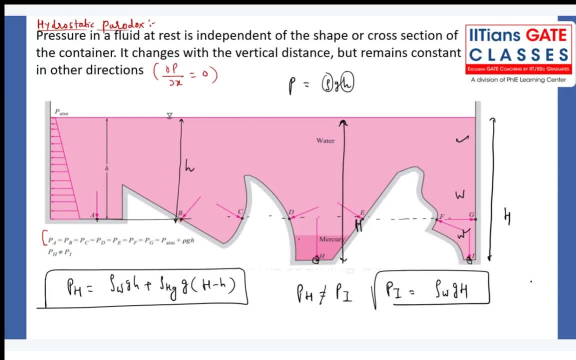 right, no, pg will not be equal to pi, why the height of the liquid is different. getting my point, as they are having different, different heights, what is the pg value? rho of water- g into small h and what is the pi? rho of water into g, into capital h? 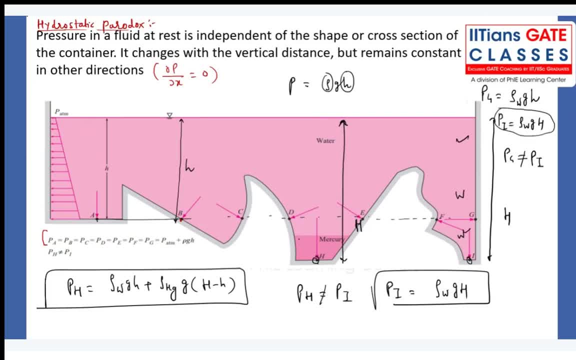 right, and what is the sign of the point at one point, at one point at one might have equal, all of your noted down. can i move to the next one then? so note down the next particular concept, that is, hydraulic lift. which is what is the hydraulic lift? 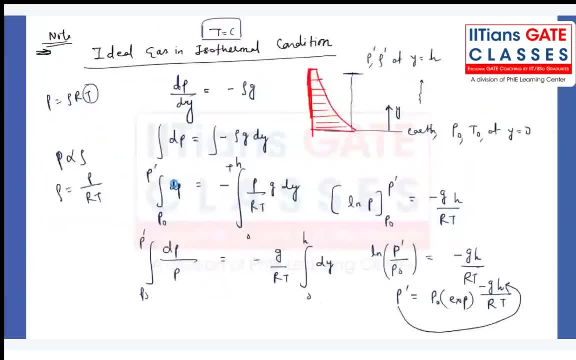 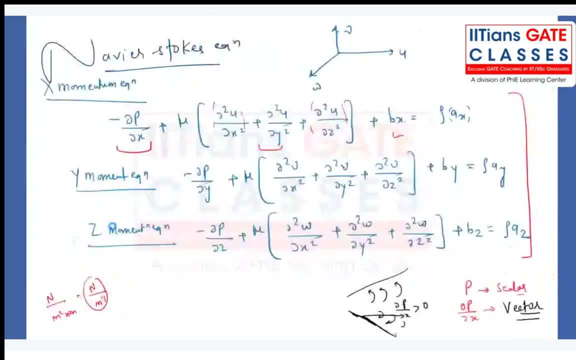 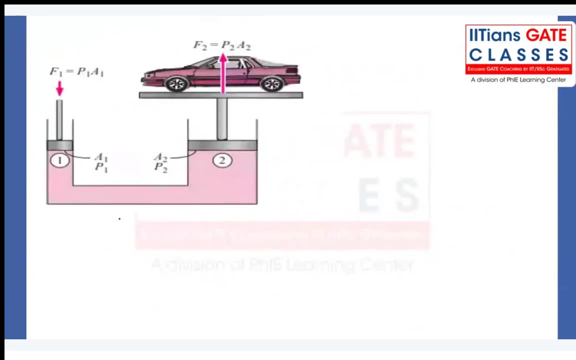 which is one thing, which is another one that you can see of the process of the hydraulic lift. what is the hydraulic lift? okay, not on this one. so, with this small effort, how can the particular in automobile industries- you have seen that they are lifting the car for some, you know, maintenance purpose or some doing? 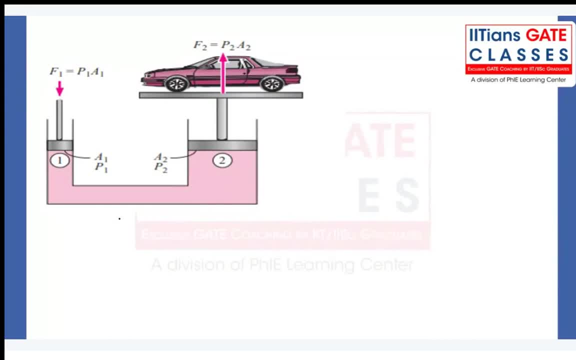 uh, you know checking, and all they used to lift this one by the hydraulic jack or hydraulic lift. that is basically working on the principle of what same thing: dopy by do x. uh, that is equal to zero. that is a pascal law. we also say hydraulic. 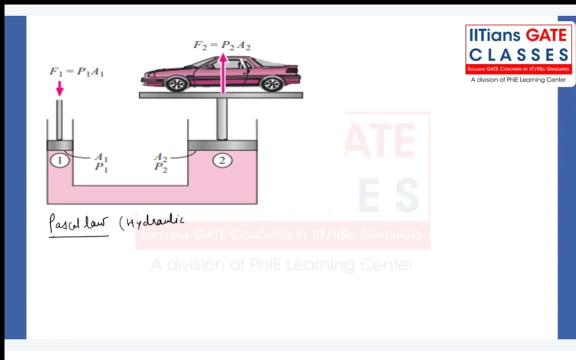 lift. so what you are observing: pressure at one point for this particular fluid which is being traveling, you know that is being continuously present. then what we can write: pressure at one that is equal to pressure at two right, because both the points are at the same level, dopy by do x, equal to zero right. there is a no variation of pressure in the x directions. 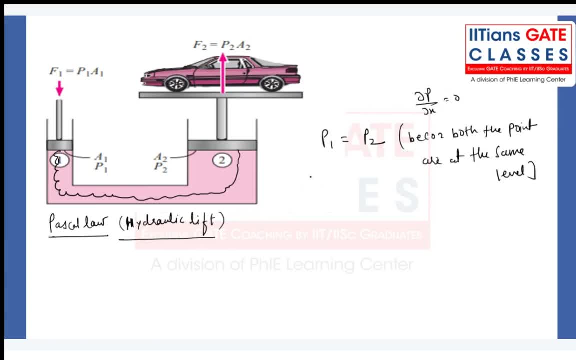 so what we can write one is what f 1 force. we are applying little bit of force and we are lifting a very huge weight that is equal to what the weight of the, what we are calling the car. so, as you can see here, f 1 will be what f 2, a 1 by a 2, a 1 is what less than a 2. so definitely f 1 will be less than f 2. so we do the little apple level. weight of the vehicle. where is y ui? is x 1? is it more than 0.2? so that is equal the weight of the car. so, as you can see here, in terms of publishers, looking at this, we just have two. all. we can start here and see here: x: 1 for the dopyices, the f1 force captain and each the give some answers. first we can just write downке manyежhjiafish g 170 Photoshop Pèt. structural part which can be seen from year to year. so we will go through this page here next, sa: thousands of objects which will be seen later so that we can write out the definition that, as you will be getting the item that is. 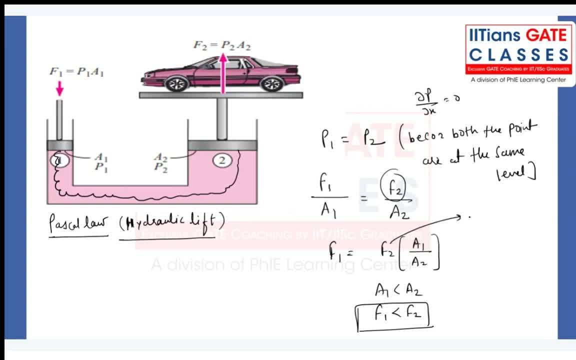 effort right and after is what the weight of the car you to provide a witness. what you can write. you can write. there are two points, one, two, and the distance is, for example, it is at a distance of X 1, X 2. so what we can write P 2 minus P 1 and whatever the gap is there that is equal to 0. so P 2. 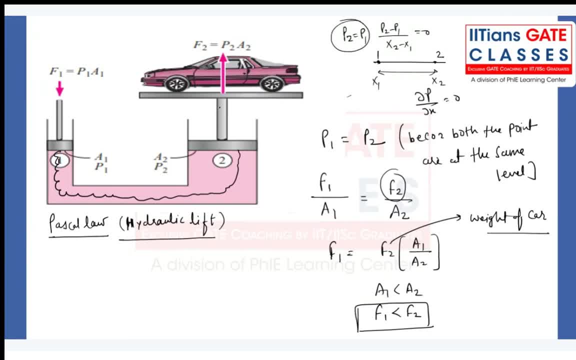 will be equal to P 1. points which are on the same level in the x-direction will have equal pressure, and that is the basic principle behind the manometer which is used to measure the whatever the gauge pressure of a container. is it done? you, you, you, now let us. 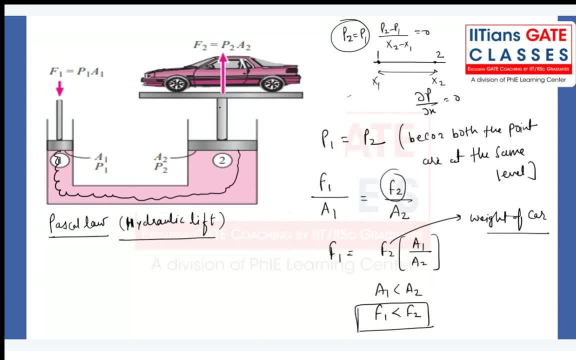 now. let us now let us some of the basic fundamental, at least some, some of the basic fundamental, at least some, some of the basic fundamental, at least some definitions of hydrostatics or definitions of hydrostatics or definitions of hydrostatics or fluid statics, and then we can start with the 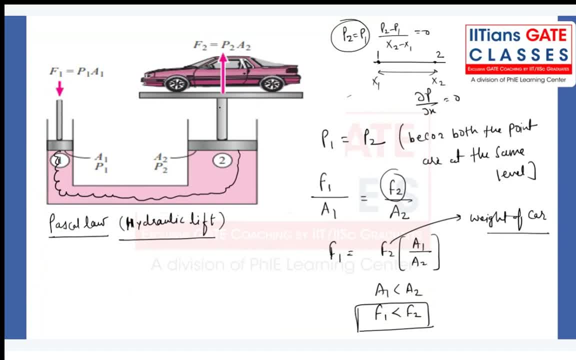 fluid statics. and then we can start with the fluid statics, and then we can start with the pressure measurement devices. that is pressure measurement devices, that is pressure measurement devices, that is barometer, piezometer, manometer, barometer, piezometer, manometer, barometer, piezometer, manometer. 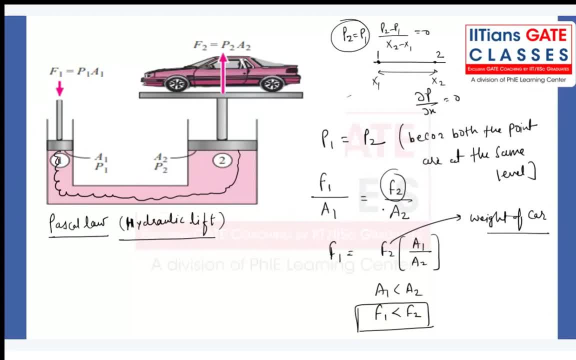 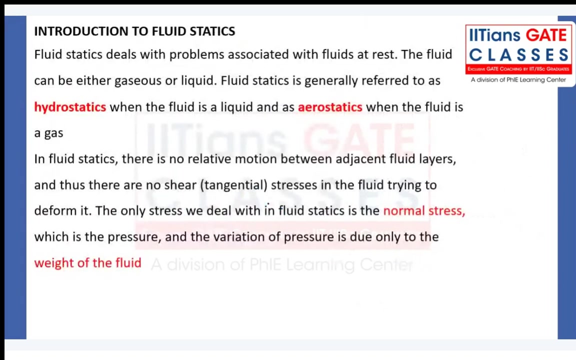 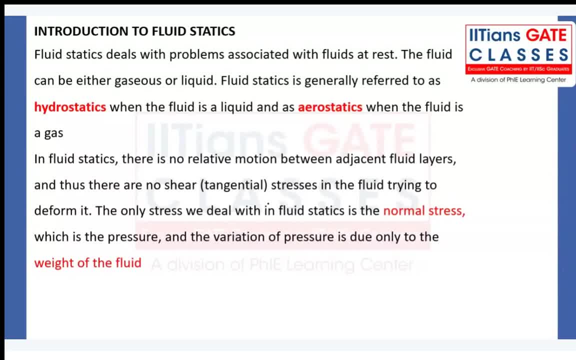 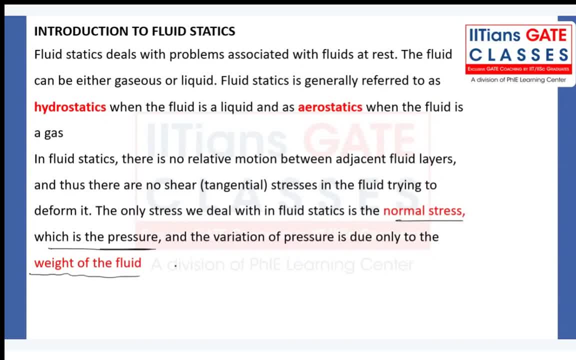 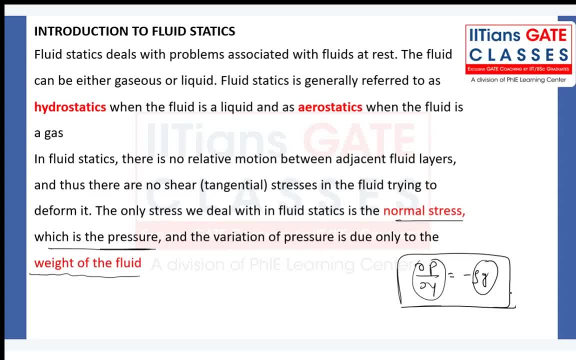 When the fluid is moving with some constant velocity. still, we can apply this law Again. I am asking: think carefully again. you just think- and tell me When the fluid is start moving and it is doing motion under constant velocity with no accelerations. 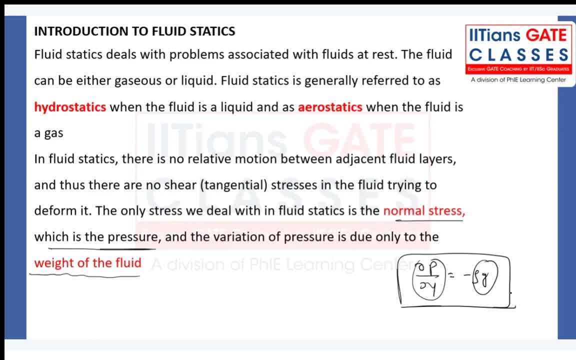 whether we can apply dou p by dou y equal to minus of rho g. Tell me, guys, why you can apply, how you can apply. tell me, when the fluid is start moving with the constant velocity, definitely shear force will be coming into the picture. 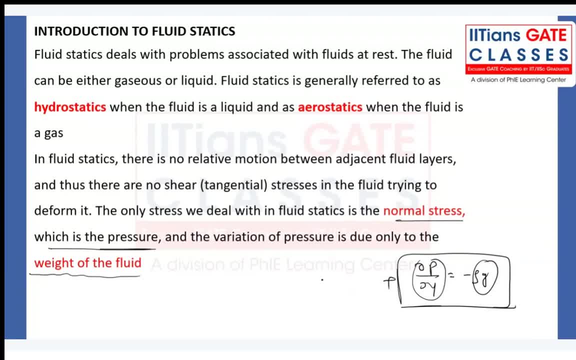 then definitely, this will also be coming: dou square v by dou x square plus dou square v by dou y square. this term will be coming. then how can you apply? I am getting my point, yes or no? The viscous force will be zero when under two case: when it is rest or when it is under. 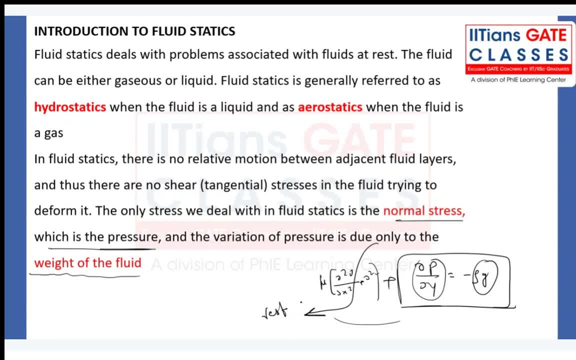 doing the rigid body motion. but again, in the rigid body motion the body will have the acceleration. so once again, this law will not be applicable. getting my point or not, Tell me guys, Is that clear? Because in MSQ they can ask even with the very basic, fundamental things. if that is. 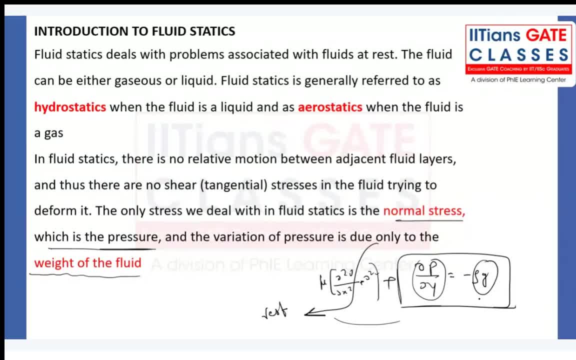 clear. you can just throw that question like anything in examination hall And remember, when you are able to solve those type of problem, then only you can expect some good rank. So don't think that, sir, with the less understanding I will be focusing on some subjects. I will 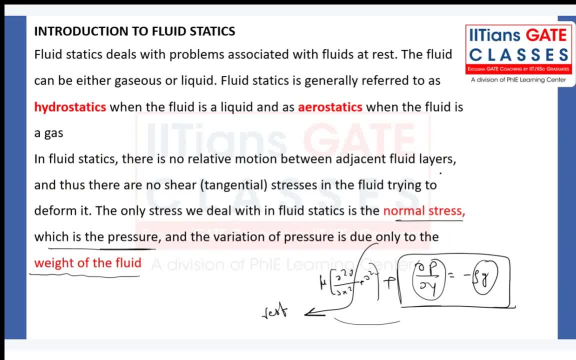 be getting 60 marks, as I know that 60 marks rank one will be there. don't fool yourself like that. Many aspirants are there. who is just doing the? you know hard work. they are understanding all the subjects. they are attempting some good number of question. good mark from that. 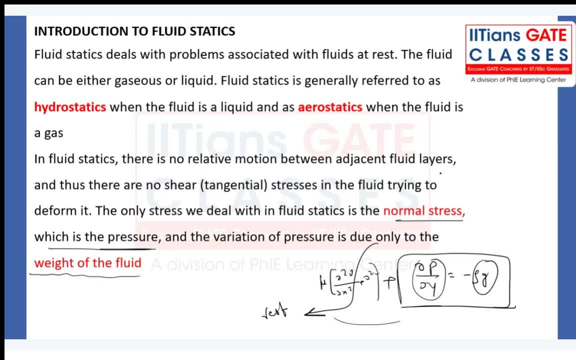 they are getting low marks. And if you are attempting only that many marks, believe me, you will get very good marks. So don't think that, sir, with the less understanding I will be focusing on some subjects I will be getting very good marks. 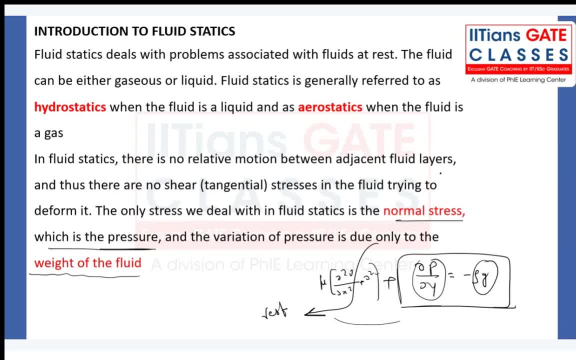 Believe me, you will not be able to get more than 40 marks. So don't be so smart in preparation that I will be studying only those few topics based on the previous segments, based on the previous year content, and I will be getting the good. 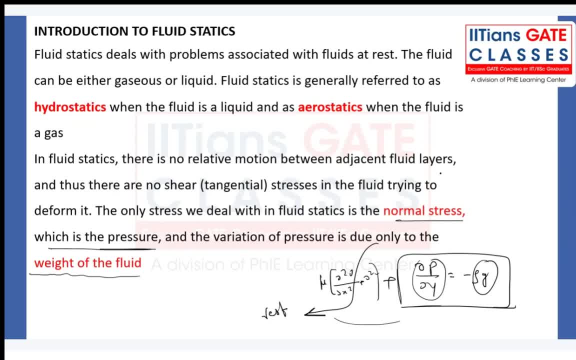 rank, That is, some in hypothetical or maybe in imagination world you are right now. If you are thinking like that, Now let's go to the next slide. Is it done? we will discuss one, maybe what we can do. we shall close it because I want. 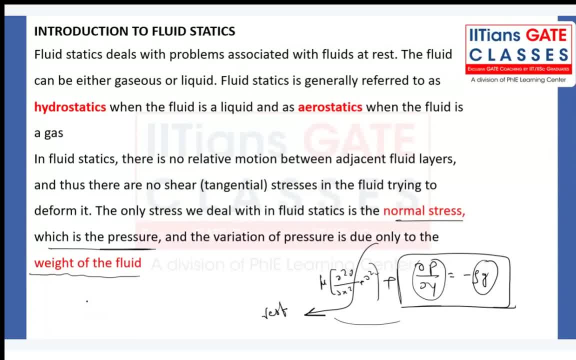 to start freshly about the barometer right, Because the moment you talk about the fluid motion, the force will be coming into the picture until, unless it is a rigid body motions, This will be zero for us or for a rigid body motion. always remember you should have basically. 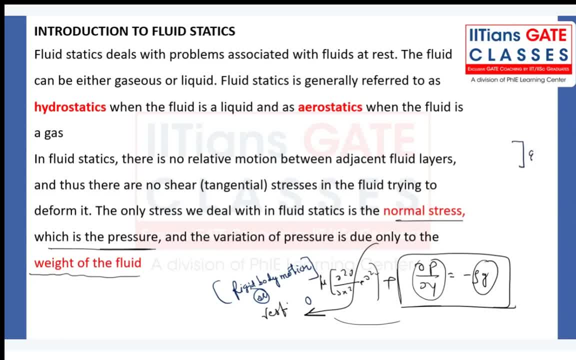 aim for a higher marks. I will be attending basically what 85 plus marks, in that you may be getting 60 marks or maybe 65 marks or maybe 55 marks, depending on the level of the question paper. right, Always aim for attempting the very good number of questions for a very good marks, you know. 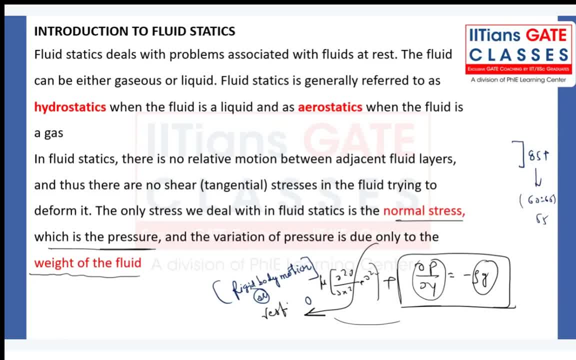 very high marks In that definitely you will be getting some 20 marks less than that. That is a general statement for all the. you know especially what I have observed in the aerospace Because I have talked about it. So basically I have basically what I have the conversation to the basically what with. 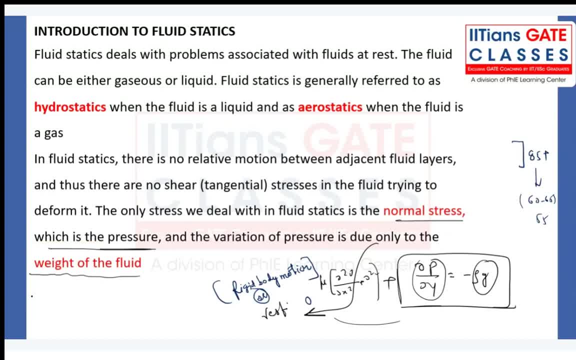 the toppers. they have said that you know this thing, they have attentive somewhat. you know 80 plus marks in that they got something like 60 marks or some of the students. they got like 55 marks And this year I think 55 marks, 25 rank was the height. 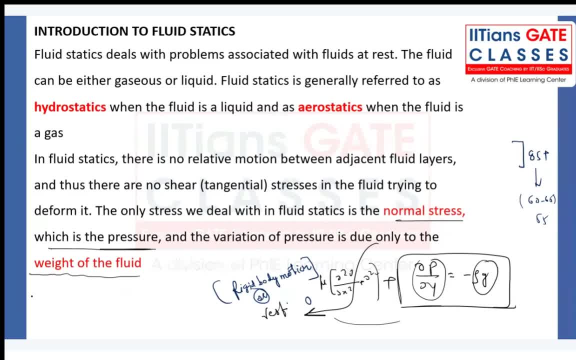 So no ways For 2023.. Correct, Because one of the students- I know that he was continuously in touch with me as he was asking the test series mock test series question and all. so he was only telling me that I attempted some good number of questions but that got incorrect. 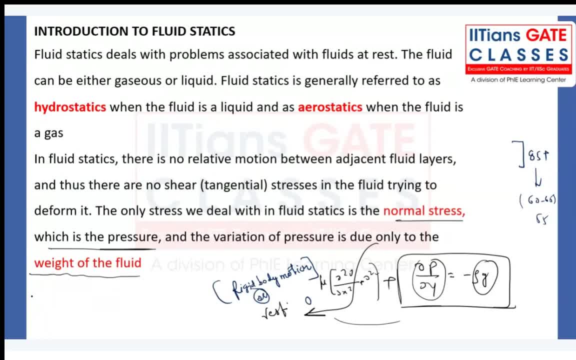 So he landed up getting this 55 marks exactly. Good, Do not. I am not going to neglect any simple topic. also, we are dealing with a very low topic. I'm telling you This: fluid statics is zero. You may not be able to get single question also. 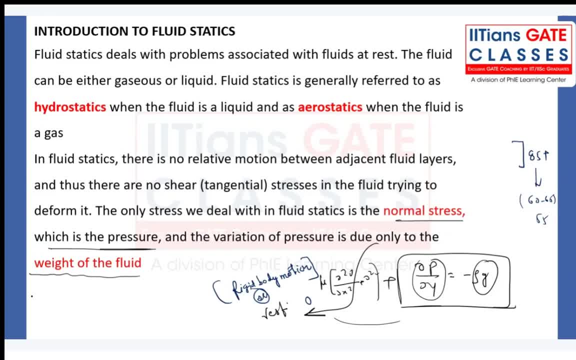 But if you are getting question, you make sure you attempt correctly that particular question, don't do any kind of mistakes, And you can see that I'm not dealing with only fluid statics. I continuously basically invoking the or maybe indulging some other topics of fluid dynamics. 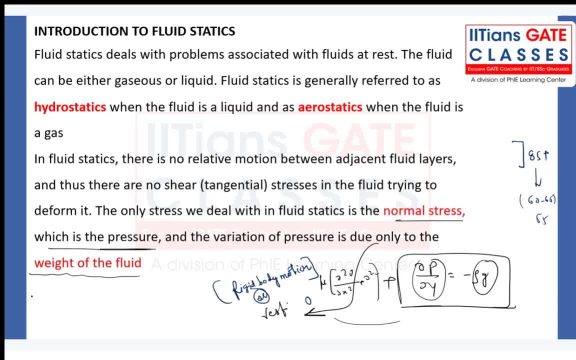 and fluid kinematics: Right, So that we can link the topics or we can connect the dots between the topics of a particular subjects, Right, Okay, guys, Thank you, We can see on Tuesday remaining topics or maybe Wednesday, right, So only we left with the two topics hydrostatic forces and then we we are left with the topic. 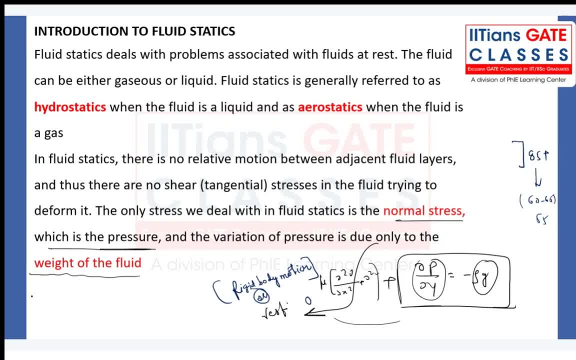 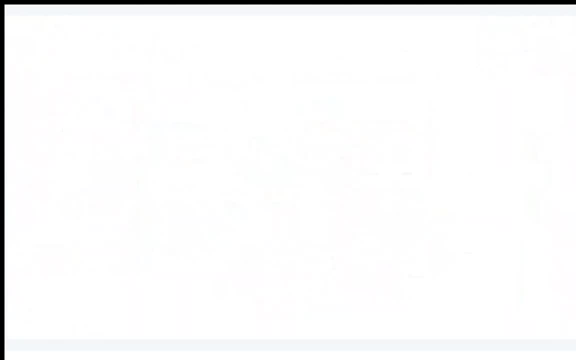 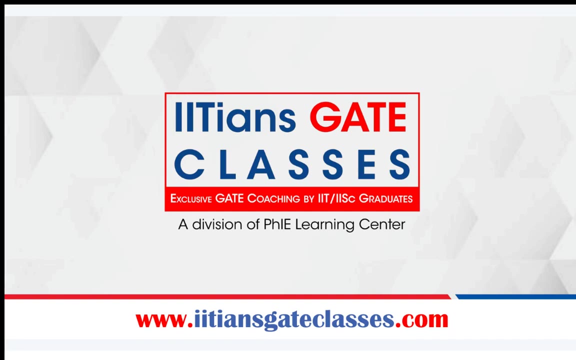 of this pressure measurement and hydrostatic forces, Then we will start the fluid kinematics. Okay, So let's start with the fluid kinematics. surface tension: are you from mechanical send you? No, that is not that important. I will be discussing in separately for the mechanical. 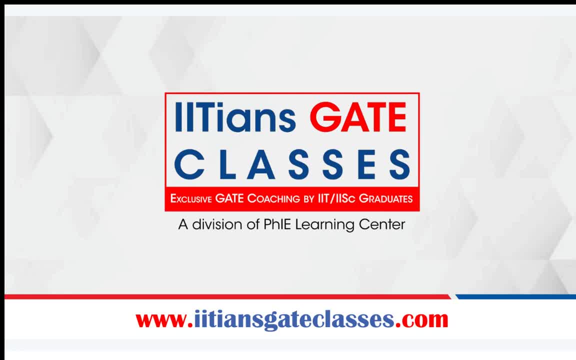 If you want it, you can attend that session. Capillary action- surface tension. I will be dealing separately for mechanical, because that is not that important, because surface tension, you know, that is also one type of force which will exist when the fluid is at the rest conditions. but we have the very negligible value of that surface tension. 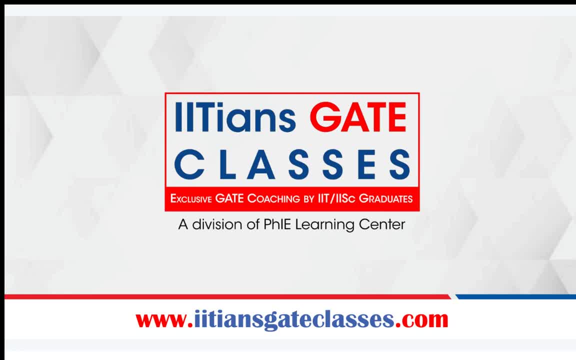 Okay, Thank you, Thank you guys.